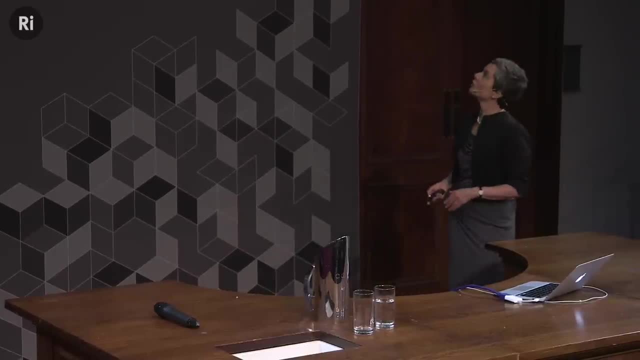 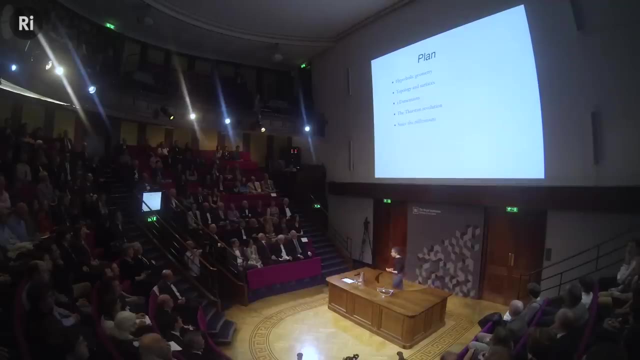 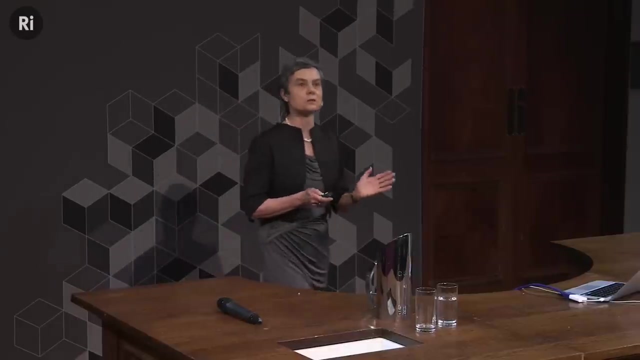 try and give you some sense of the enormous strides that Thurston introduced. and then, since the Millennium, there have been further enormous strides that have been made in the last 20 years, which in some sense have completed a large part of the programs that Thurston initiated. so I want 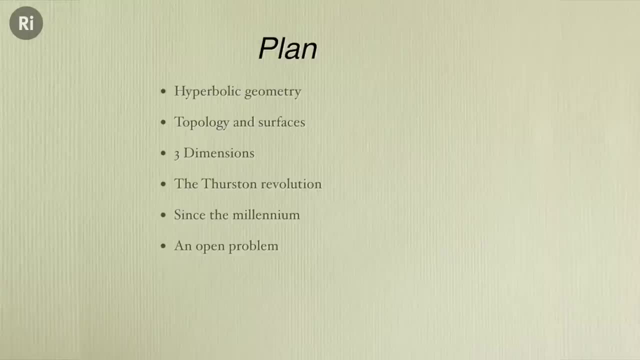 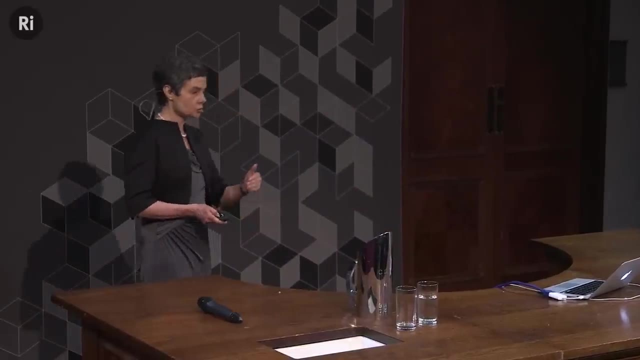 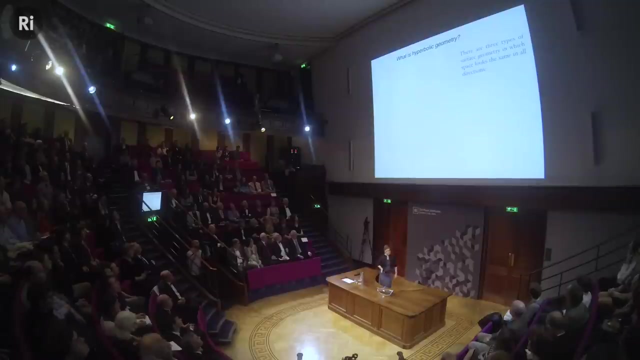 to try and give a flavor of that and then finally talk a little bit about an open problem which I think is very fascinating and which touches on the work that I've been doing and which also relates to some of the ideas I shall be telling you. so that's where we're going to go, so hyperbolic. 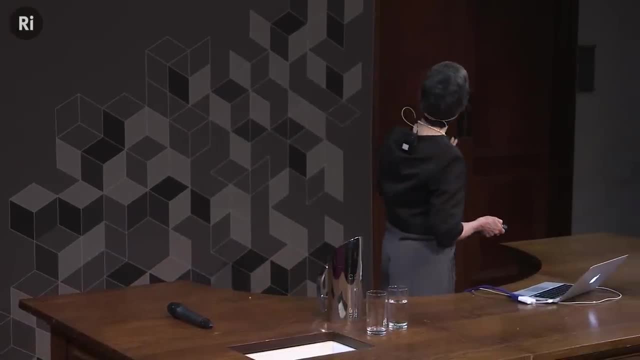 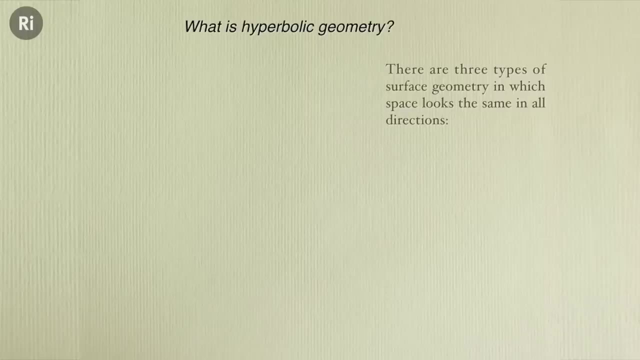 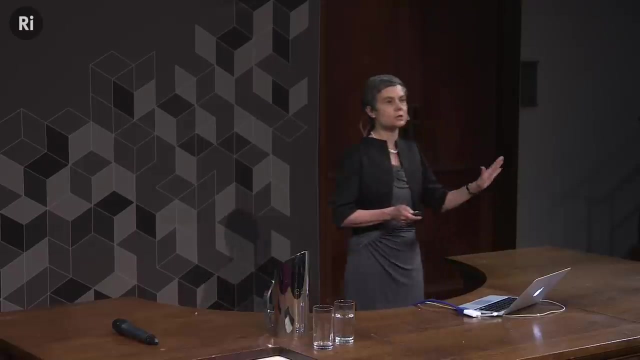 geometry. if you think about geometry at the end of the nineteenth century, it was the first time that there was a lot of discussion. what is geometry? you could say geometry is study of space. well, we're going to start in two dimensions: space in which, wherever you are and whichever direction, 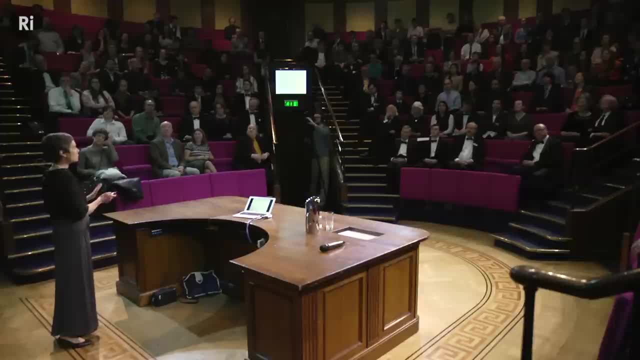 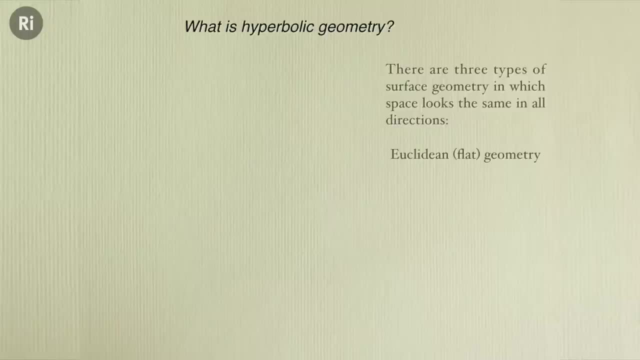 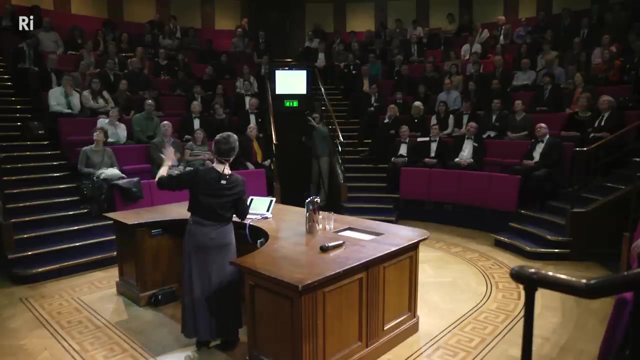 you look, what you see is kind of the same. so, whatever it is, it looks the same everywhere and of course the most obvious kind is ordinary Euclidean geometry. but you might also be living on the surface of a sphere, and wherever you are on the surface of a sphere, you might also be living. 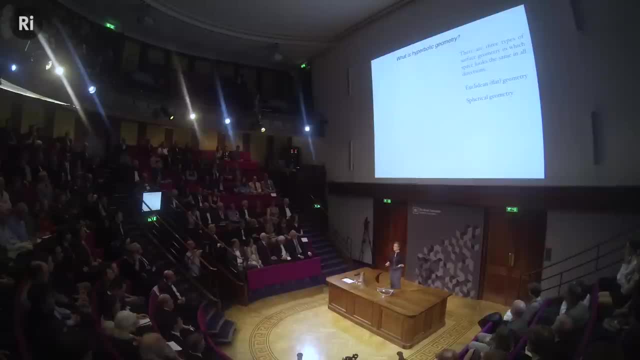 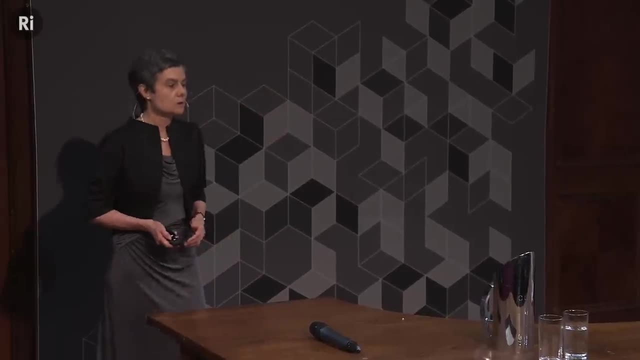 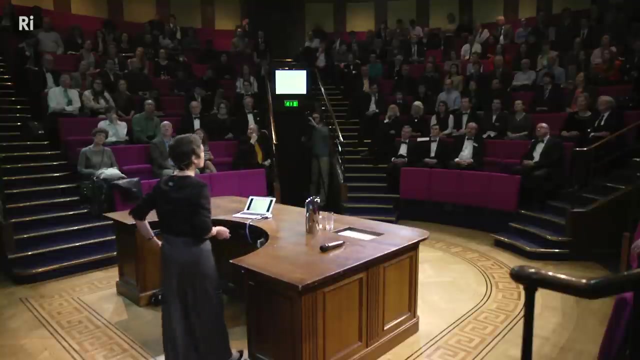 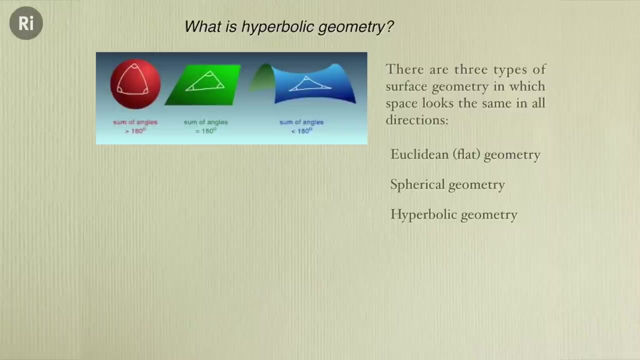 on the surface of a round sphere, things look the same. they don't look quite the same as if you're on the flat, but they look the same. and the third kind, the kind that was missing up to about 200 years ago, is called hyperbolic geometry. so here's a picture that shows rather well Euclidean geometry. 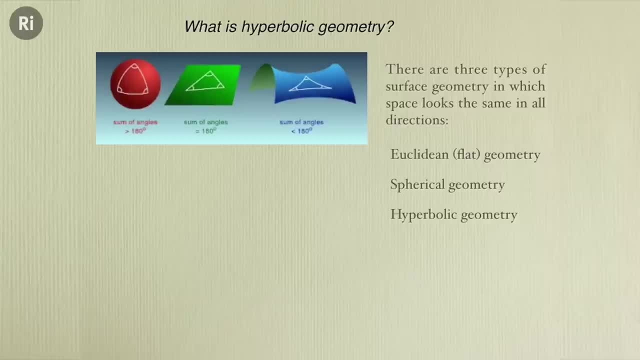 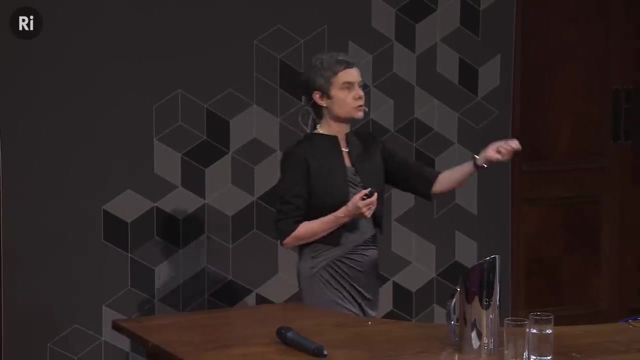 everybody knows, the sum of angles in a triangle is 180 degrees in a sphere. well, what are the straight lines on a sphere? they're the great circles, the way aeroplanes would fly to go the quickest way. so the great circles on the sphere. and if you start, 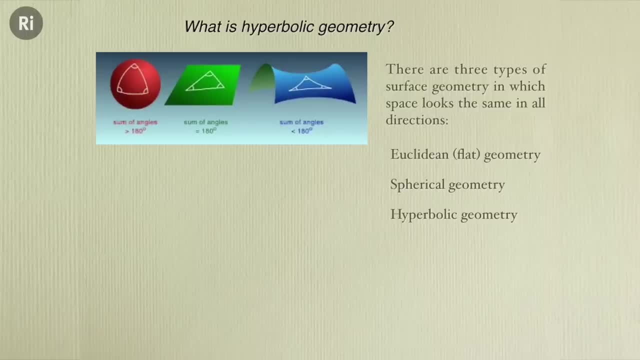 playing around drawing triangles on a sphere whose sides are great circles, you very quickly come to the conclusion that the angles add up to something greater than 180. how much more than 180 depends by a very precise way, and that's what we're going to talk about in the next lecture. 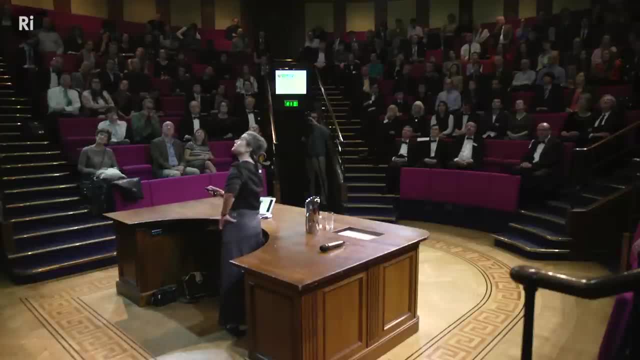 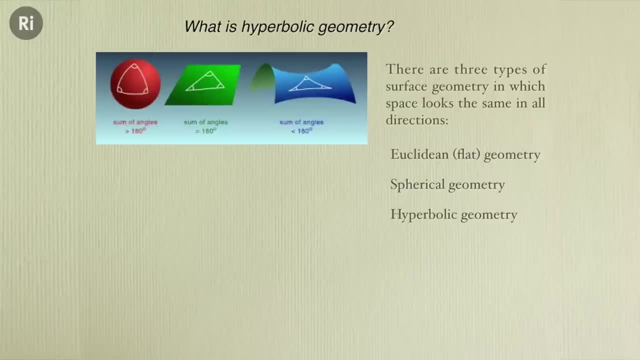 These ropes move the almost at the end this way on the area of the triangle. and the third kind of geometry then is the kind where the sum of the angles in a triangle is less than 180, so there's a kind of pairing between these two things. so hyperbolic geometry you can. 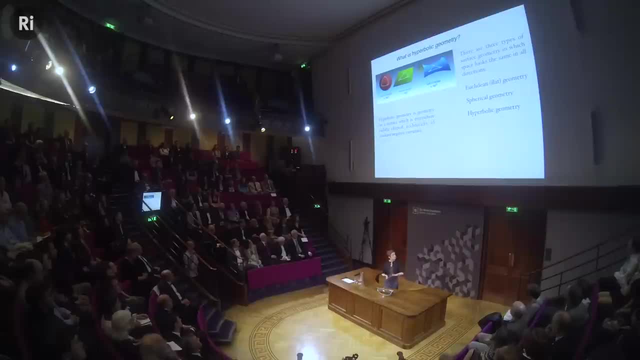 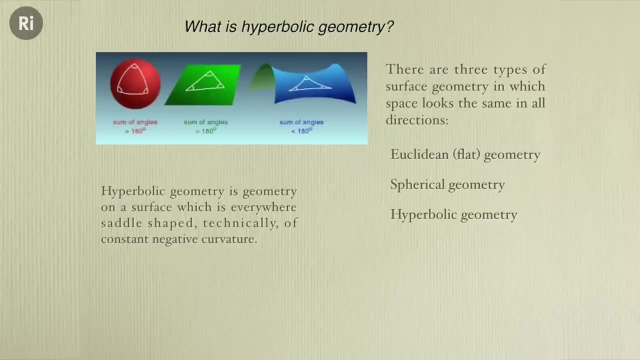 think off as geometry on a surface which is everywhere saddled, shaped, so you see in this picture, afraid it sort of curves down that way and then over at Hump in the other direction. so, assertingank, the eye is now a bump in another direction and this is actually a distinguishing. 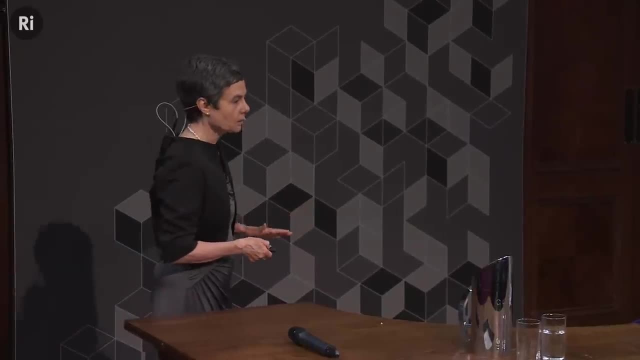 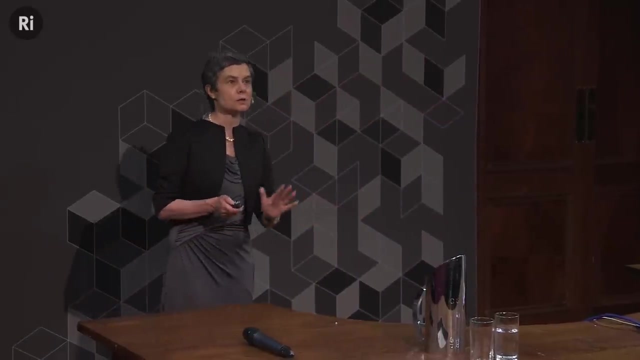 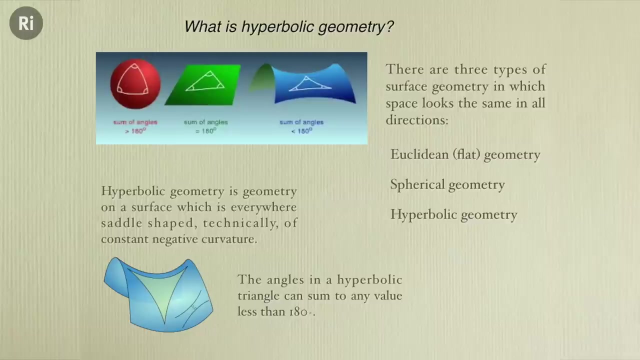 surface of negative curvature. Hyperbolic geometry was first discovered in the search for a proof of Euclid's parallel postulate. But rather than finding a proof, a whole new world of geometry was discovered, and we can nowadays Interpreted in this rather nice way. so 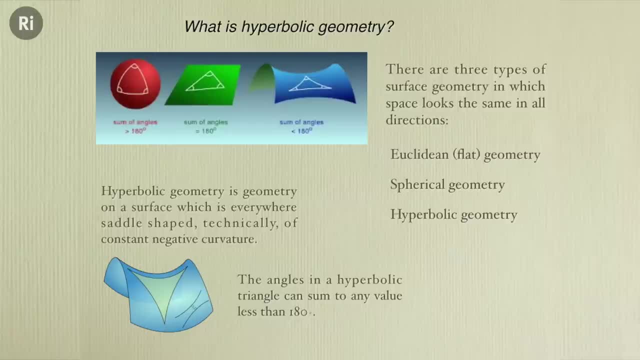 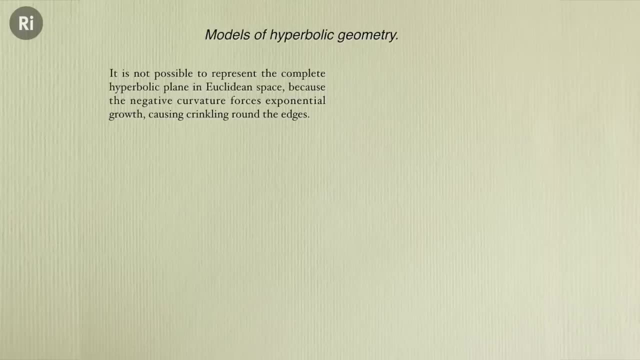 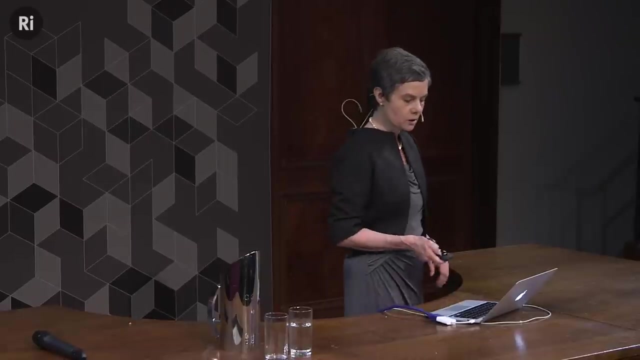 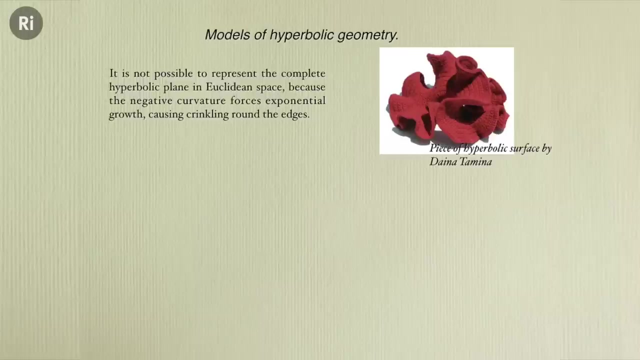 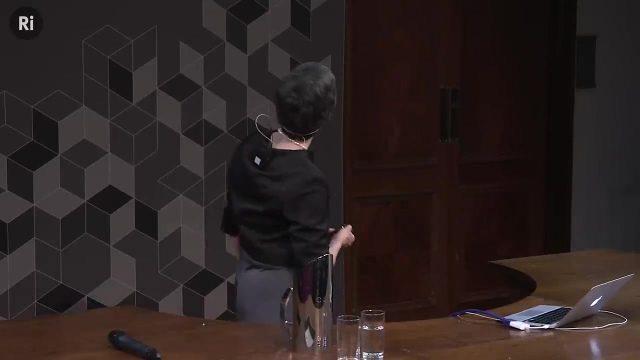 How are we going to model this geometry? well, you Can't put the whole sort of plane of this geometry into ordinary flat Euclidean space, Because it's too big, basically. so this is one of a rather nice series of crochet Models that's been developed by this person, Diana Tamina. There's a, in fact, a whole book. 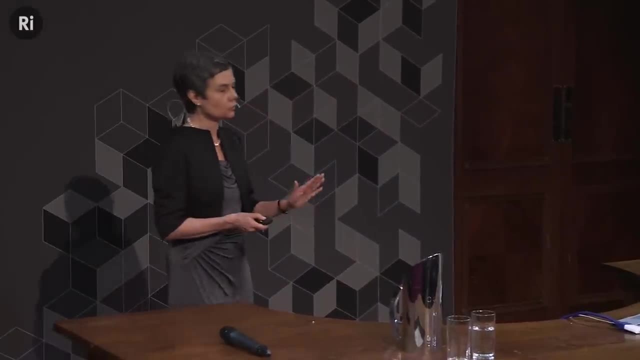 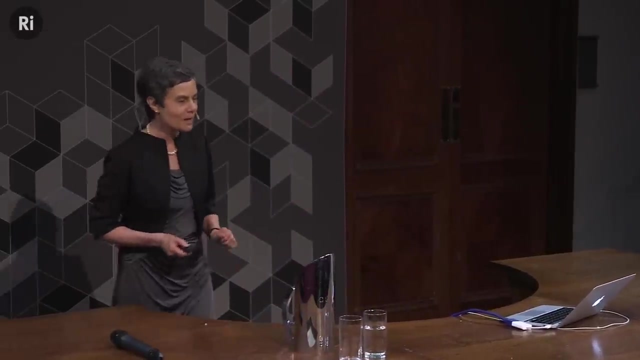 You can buy about making crochet models of geometry. There's a whole project which has made a coral reef out of crochet, which I think is in Dublin, I'm not quite sure. anyway, You can make these models and the main point is once you start trying to make a surface, 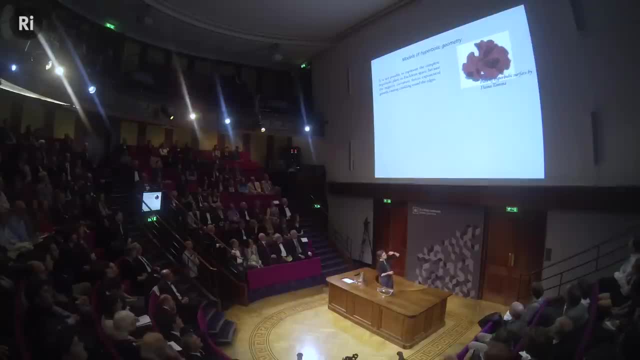 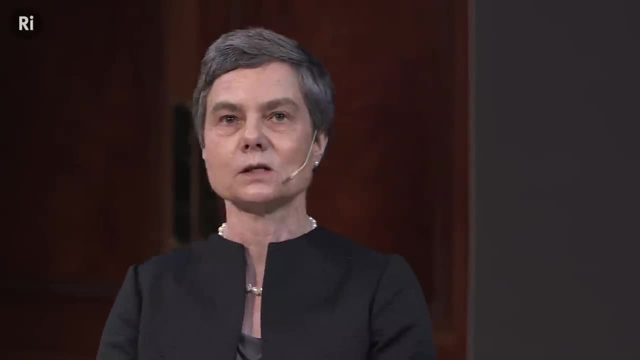 That's curved the right way. it starts crinkling up and crinkling up And if you kept on before too long you would find it was just so crinkled around the edge that you just couldn't fit it In there anymore and you would just have to stop because you you wouldn't have any more space to make your stitches. basically, 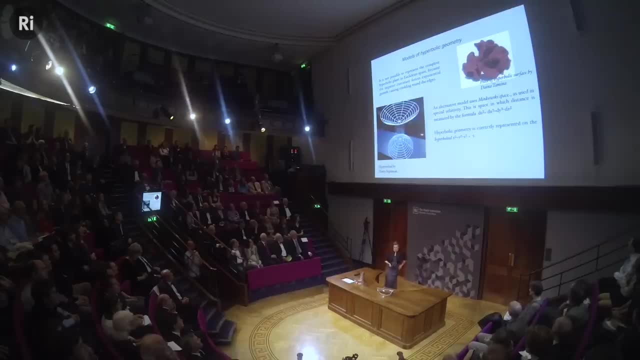 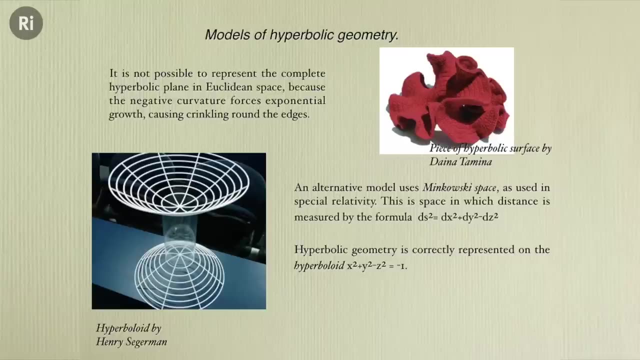 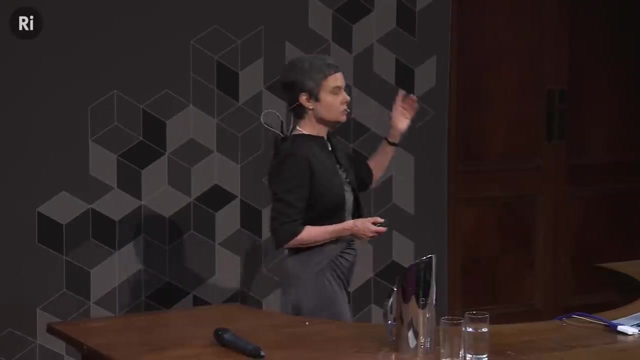 so Here's another way to do it, which perhaps Some people may be familiar with. so if you know anything about the theory of special relativity, you can use the space which in which special relativity takes place, and I'm talking about a two-dimensional. usually one has three dimensions of space and one of time. this we're just going to have two dimensions x. 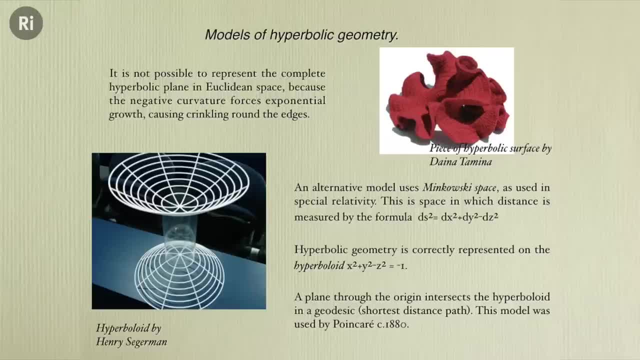 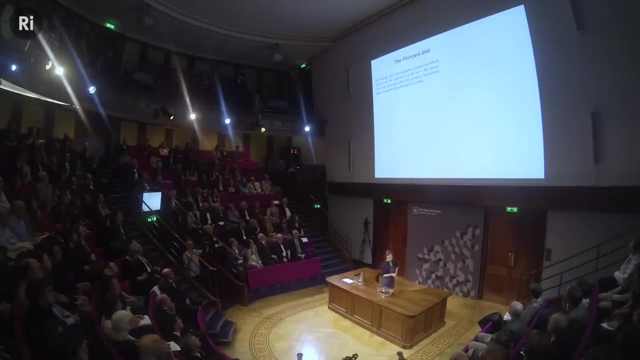 and y is space, and this is time, and this picture over here on the left is a rather nice model made by a colleague. so this is the shape on which geometry takes place, and Let me just go on. and it's not so easy to understand geometry there, so rather than doing that, we project it. 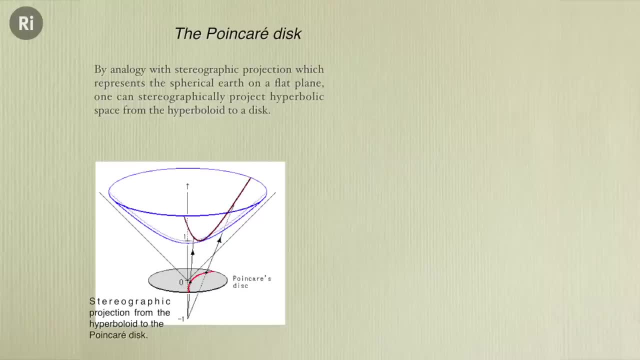 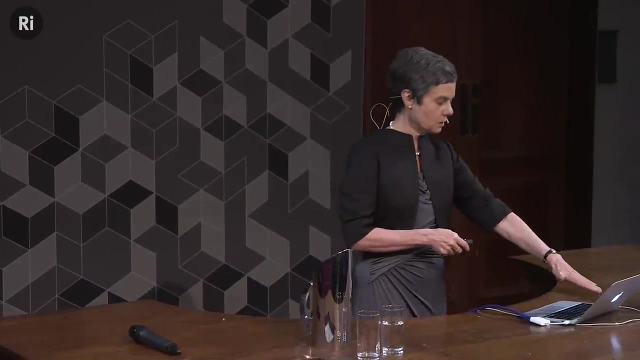 so just as you can think about geometry on the surface of a sphere and projected onto the flat plane, So we can take geometry on this shape here, with this rather curious formulas, And we can project it onto this circle. and this is the first time point Karei's name comes up. his name will come up repeatedly. 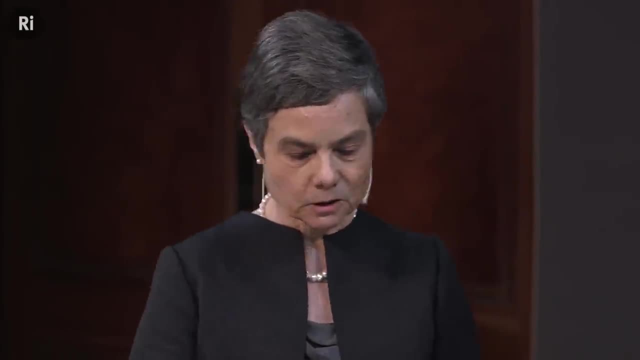 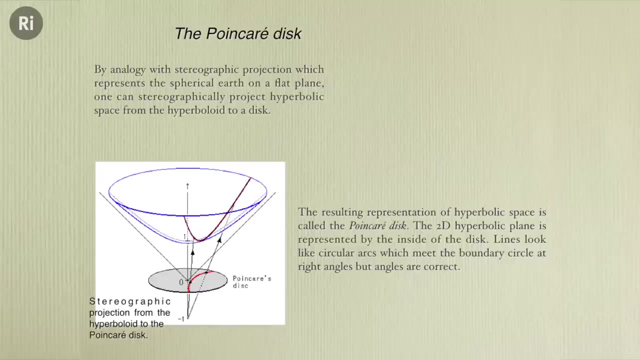 through the talk We projected onto this circle- now I didn't say but a shortest distance path on this thing turned out to be the intersection of a plane through the origin with this Hyperboloid, this blue object. and when you project it down, what you see is 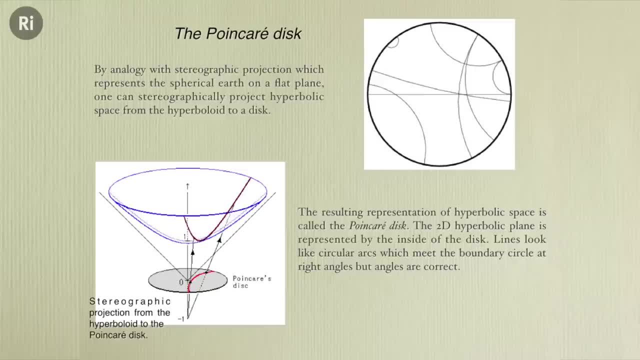 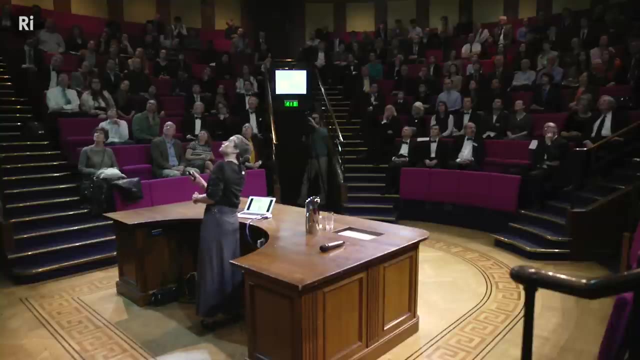 You see a disk here and you see these lines. so these are shortest distance paths, sort of straight lines in this geometry, and What they look like in our map projection is arcs of circles that hit the boundary at right angles, and So things are very distorted But angles are correct, so that's good. 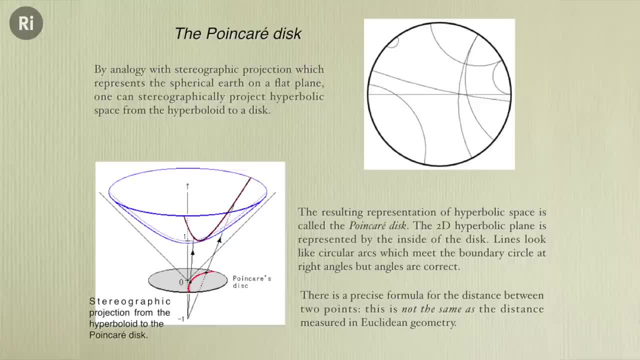 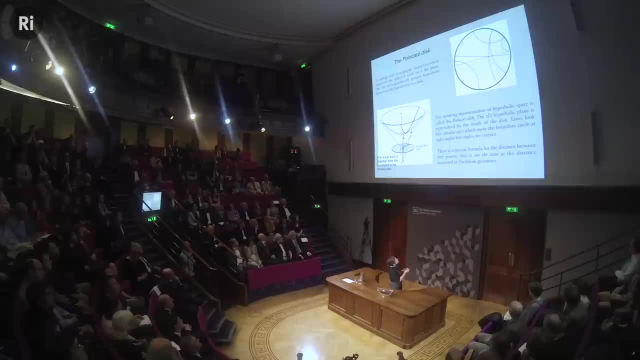 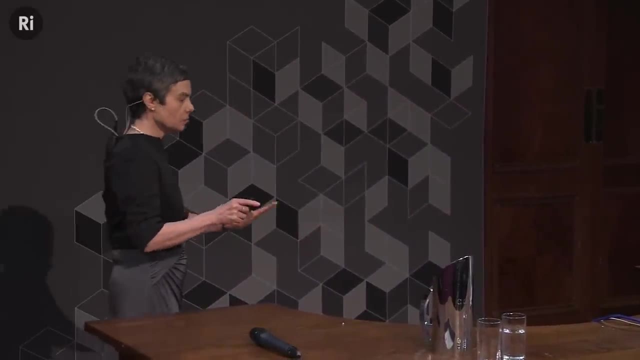 There is a, of course, there are precise formulas for all this, which I'm not going to try to explain tonight there. formulas And the main thing to remember that this is like a very distorted thing, like when you project onto a flat atlas. Things are completely distorted up near the North Pole They're very wrong, so don't think that this is a correct picture. 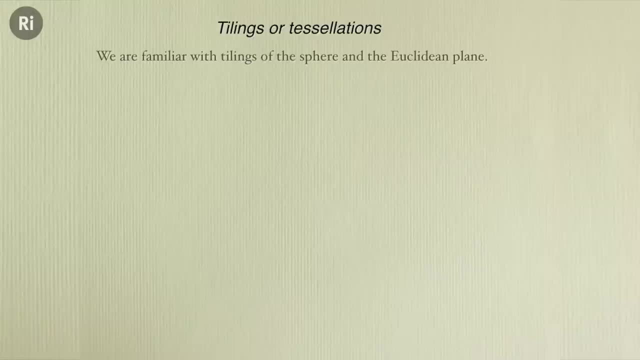 But nevertheless, let's do it again, Drew. Let's carry on and talk about tilings. A lot of what I want to say is connected with tilings, So everybody knows how to make tiling patterns in the ordinary Euclidean plane. 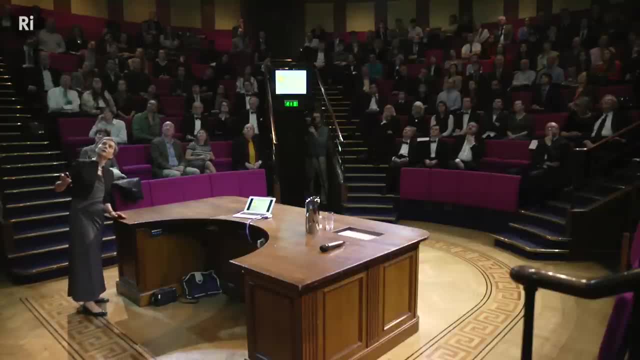 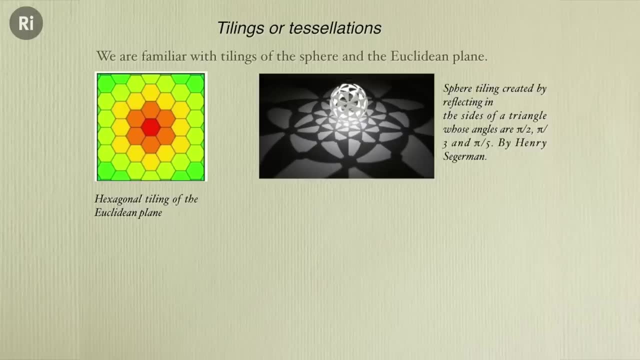 the kind of thing you play around with at school, And you can make tilings of the sphere. This is another nice model made by Henry Siegermann. So here is a sphere with a tiling pattern on it, and he's rather nicely projected it in this photo. 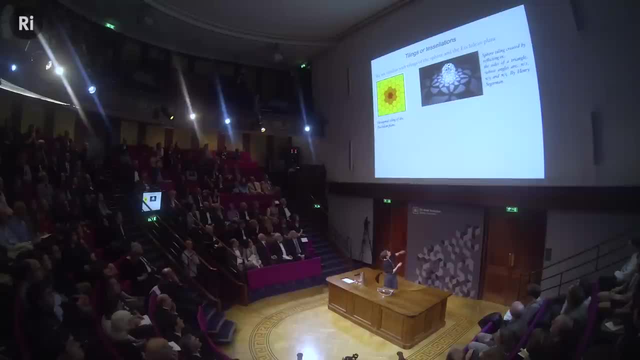 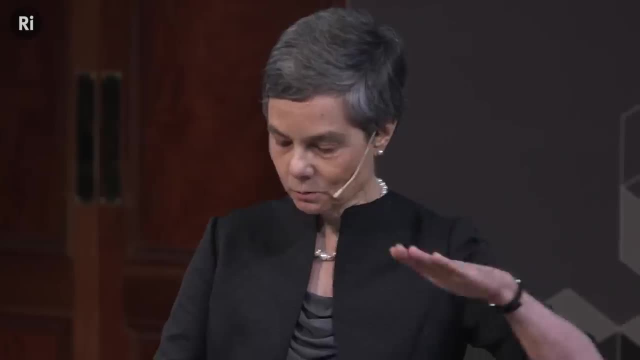 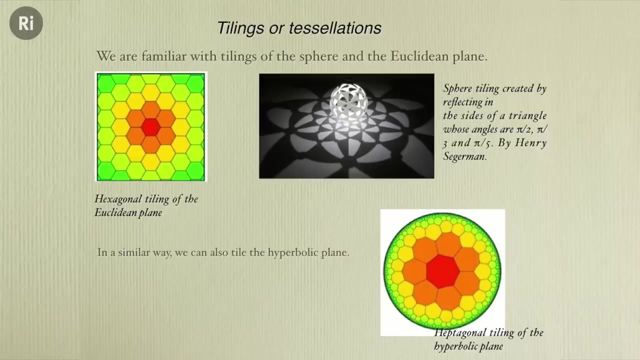 onto the flat plane And of course here you can see, here's a sphere, well, here's everything distorted. So we kind of see the idea of distortion in a projection. What about tiling the hyperbolic plane? There is a picture of a tiling of the hyperbolic plane. 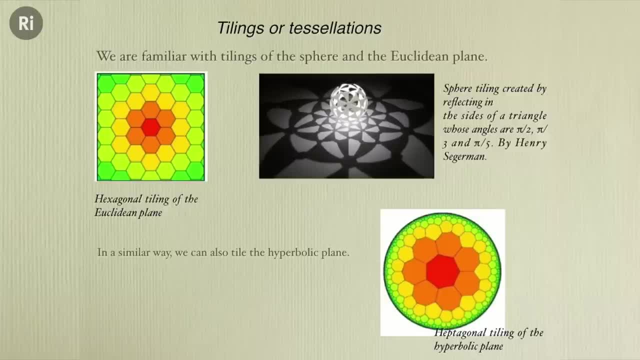 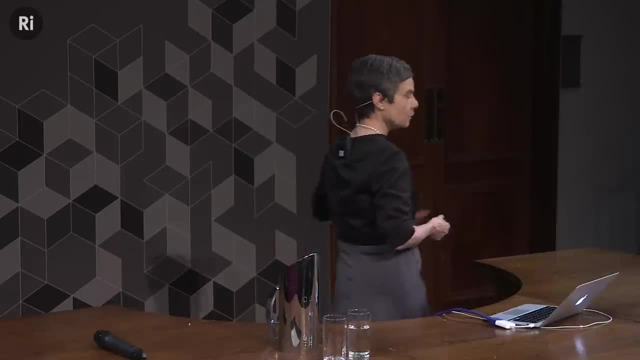 and the thing to take in here is that, although these shapes, they're actually heptagons, although they look different actually, from the viewpoint of this geometry, they're really the same. So, in other words, just as in the hexagon picture, 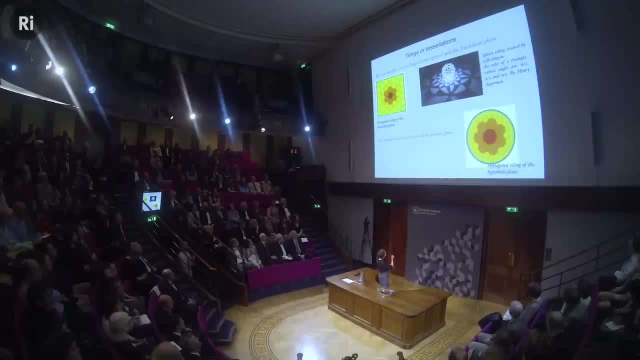 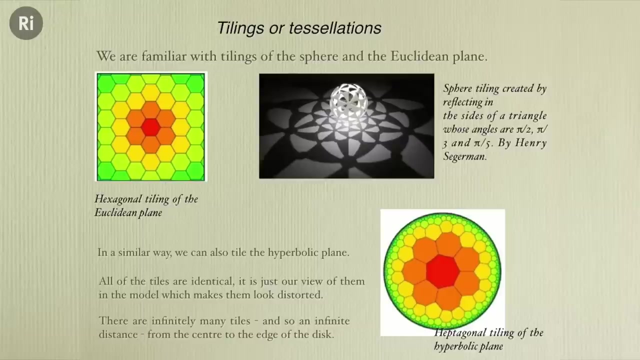 every tile is identical to every other one. There's a rigid motion of geometry that carries one to the other. The same thing is true in this picture. One thing about this picture is that if you count the number of tiles around here, they increase. 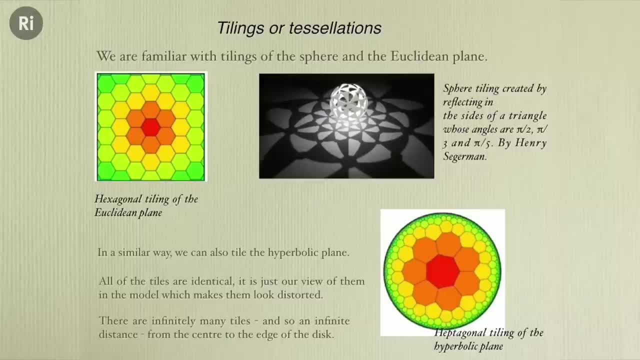 Linearly as the radius of your circle. if you count the number of tiles here, you find they increase exponentially fast, and that's related to this crochet surface that I had. that was all crumpled up. There's more and more and more of them. 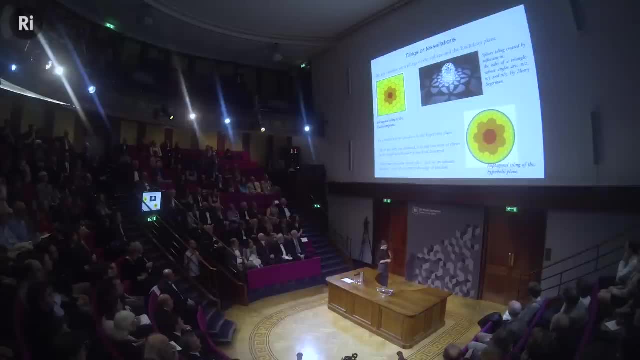 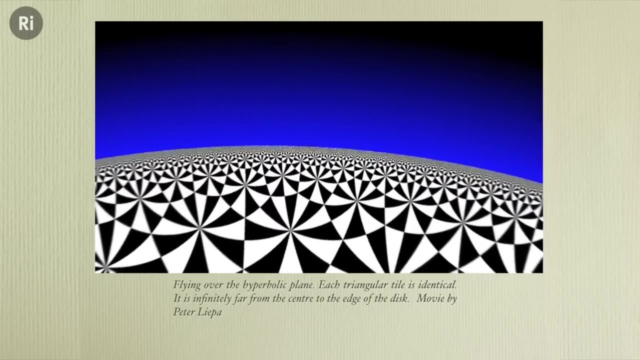 and there's an infinite number of them. to get from here to here. It's an infinite distance and this rather wonderful little video clip shows you probably better. It's going very fast, but there we are. There we are. All of these shapes are the same. 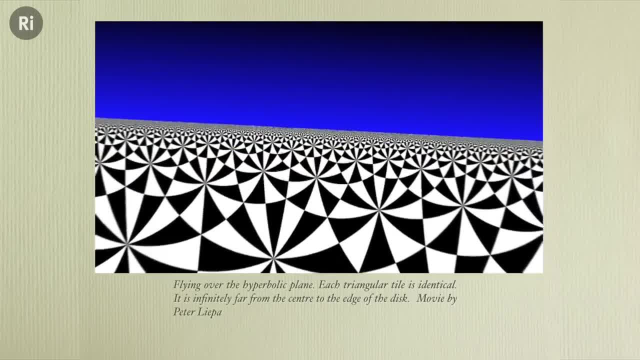 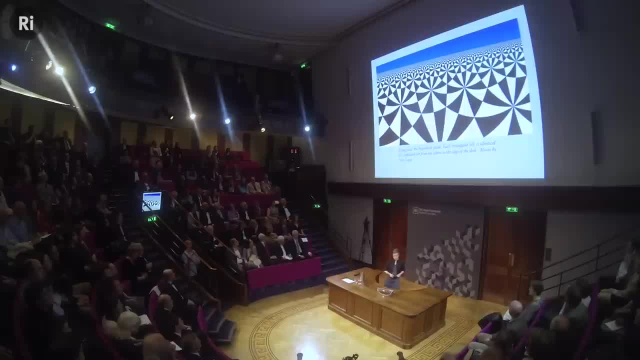 and we're zooming on. Peter Lieper is another computer graphics person who's got kind of fascinated by some of the things that can be done in mathematics. So this is a picture and, as you see, we go on and on and on forever. 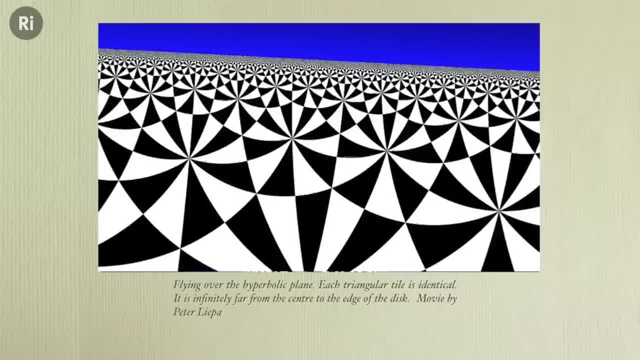 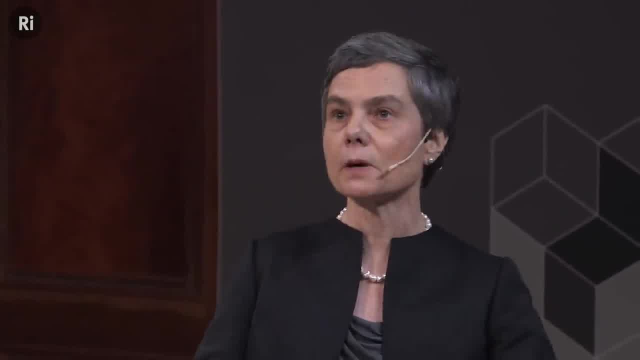 and out at the horizon. it just goes on and on and it's infinitely far away. So that's my very quick introduction to hyperbolic geometry. We're going to come back to this geometry repeatedly. Let's go on to what the word topology means. 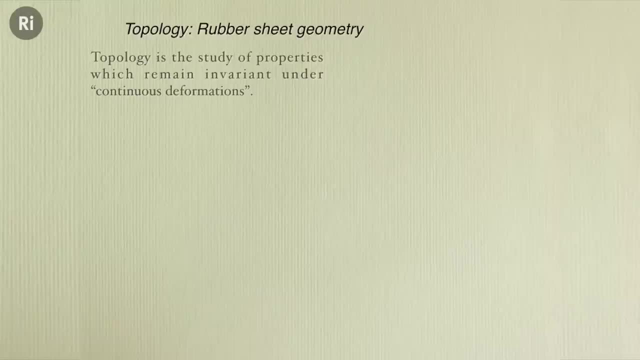 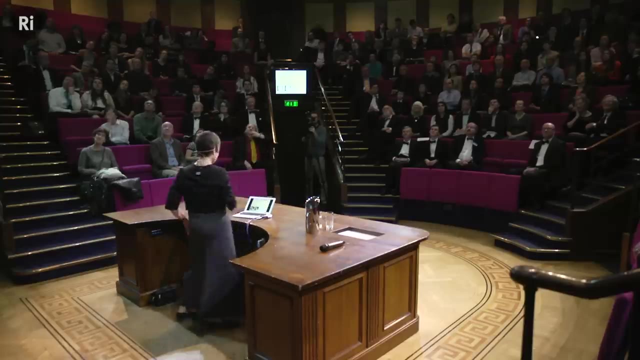 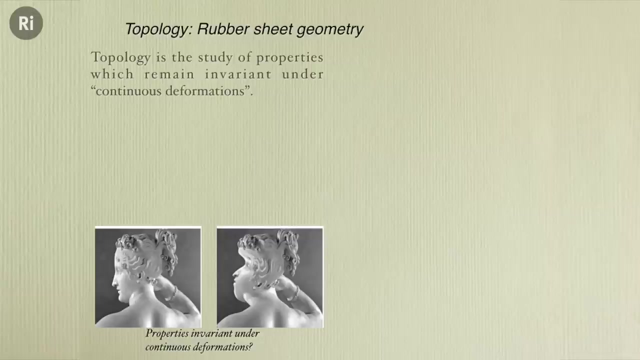 So topology, what is it? It's the study of things that remain invariant, unchanged when you do deformations. So here is a picture of what do I mean by a continuous deformation. Well, I take a thing and I squish it, and I scrunch it. 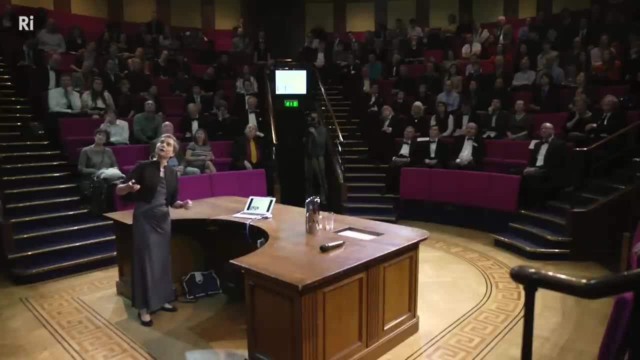 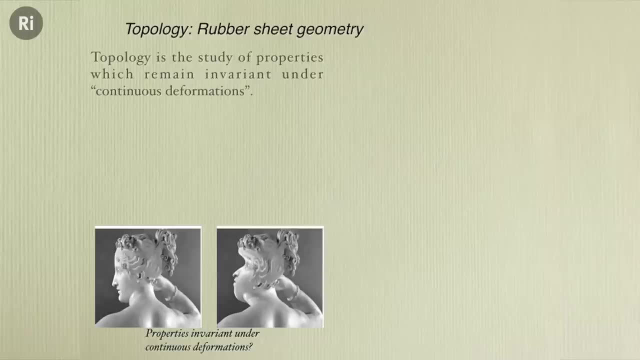 and I pull it, but I don't rip or tear it, and I want to ask what remains the same. Well, if you like, the fact that there's a little hole that I could sort of go through here between her back and her front, it's still here. 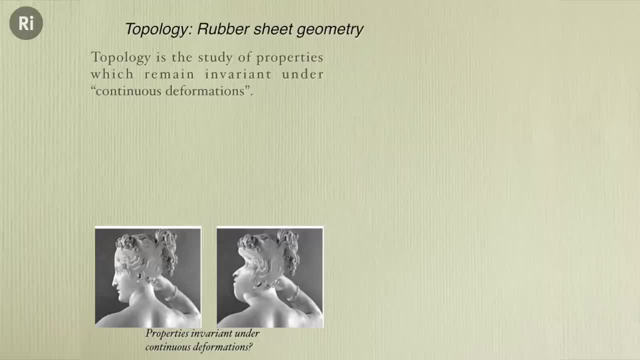 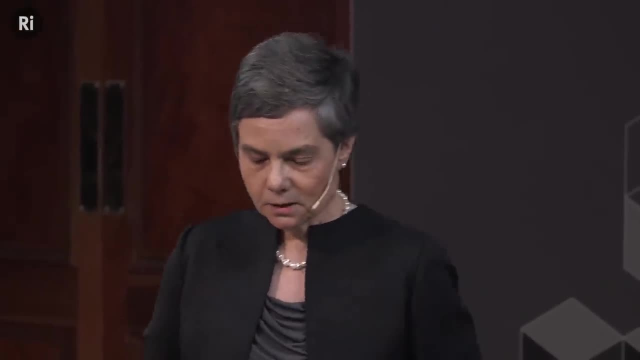 even though things are a bit kind of distorted. Well, there's more the same in these pictures, but you could distort much more than that. So that's what topology is about, and well, again, the name of Poincaré comes in, so let me introduce Poincaré. 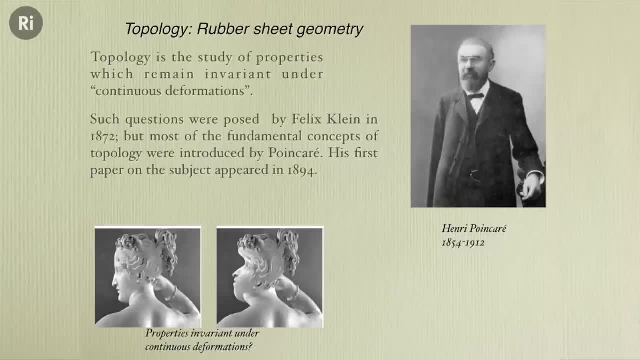 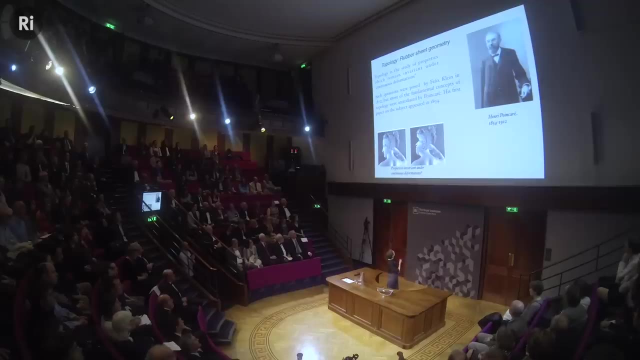 I'm sure many people here are well-acquainted with Poincaré. He was really one of the absolutely great mathematicians of all time. mathematician in mathematical physics He contributed to enormous numbers of different areas and in particular he's often known as the father 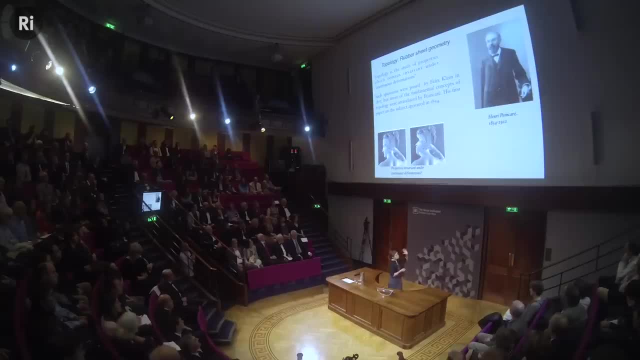 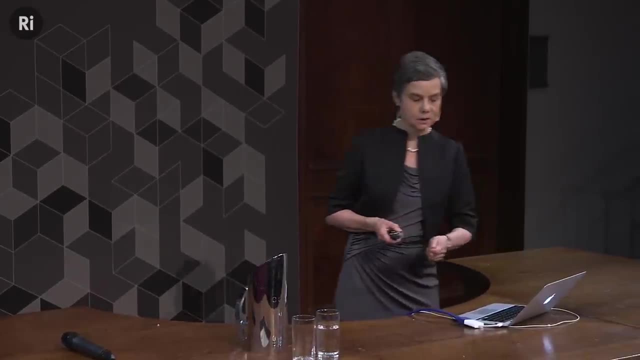 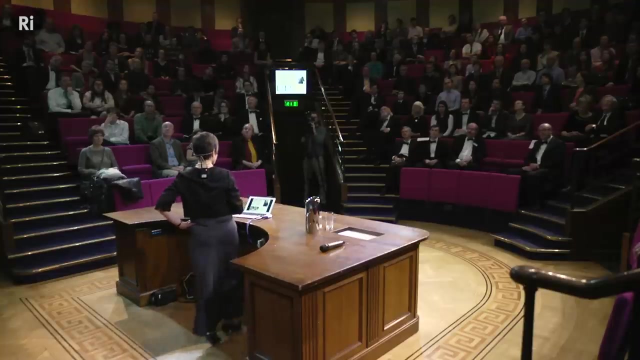 of this subject of topology, although he wasn't quite the first person to do it, but he was really the first person. He introduced an enormous number of ideas that are still the fundamental, The fundamental tools of this subject. He also, of course, was the person who wrote: 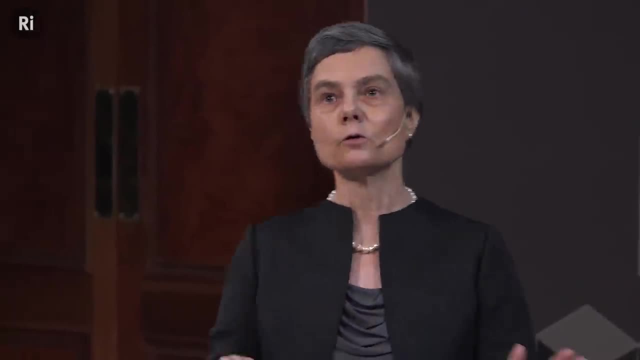 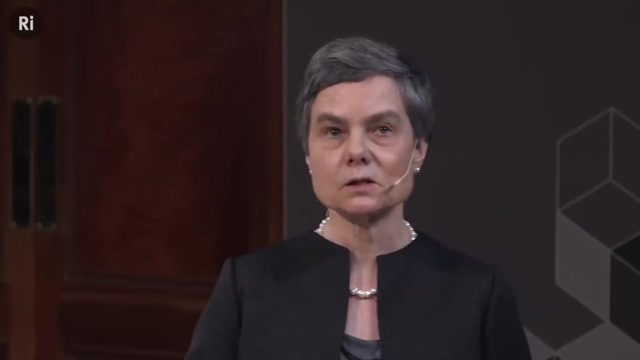 down the Lorentz transformations in their modern form, which are used in the theory of relativity, special relativity. He was the person who probably can be credited with the invention, in some sense with the invention, of what we now know as chaos theory. 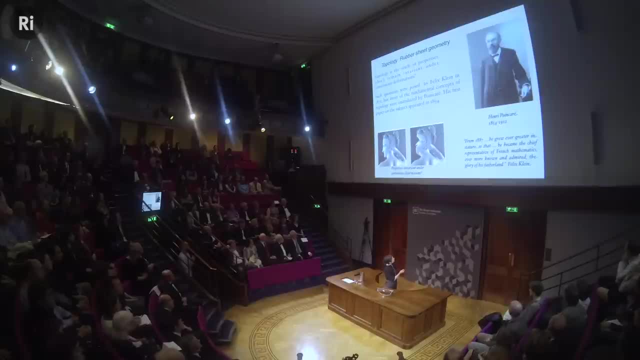 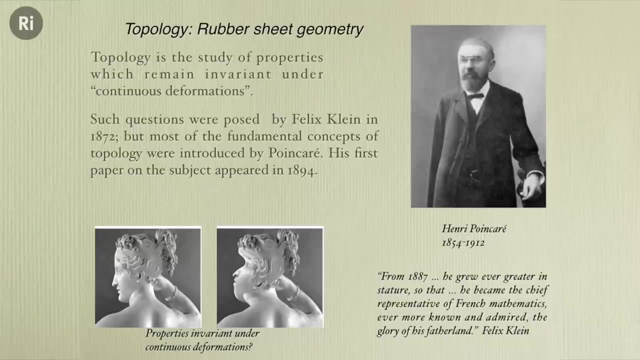 So many many things, and I rather like this quotation, which I'll leave you to read: Felix Klein, Felix Klein. Felix Klein was one of the leading German mathematicians at the sort of later part of the 19th century. Klein actually drove himself into have a breakdown, trying. 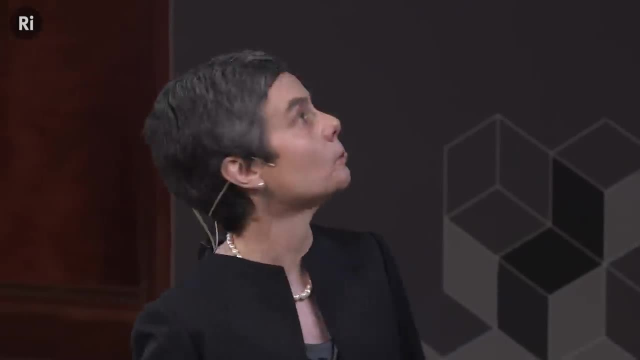 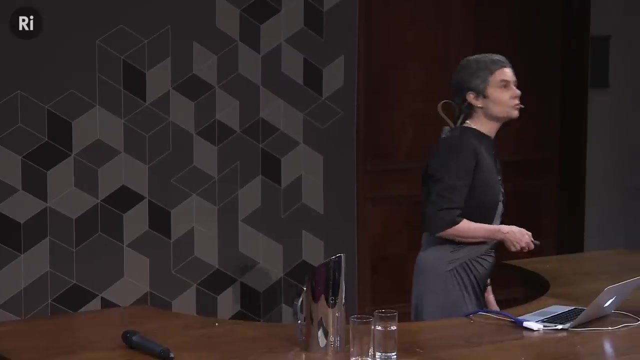 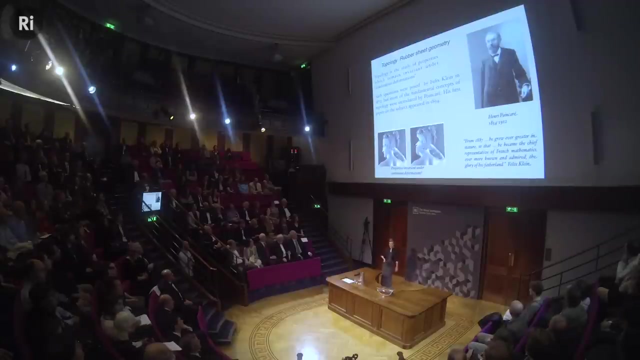 to compete with Poincaré and eventually, I think, gave up and realized and wrote a lot about Poincaré and this rather wonderful tribute. So this is Poincaré and, as I say, his name is going to keep continually cropping up throughout the 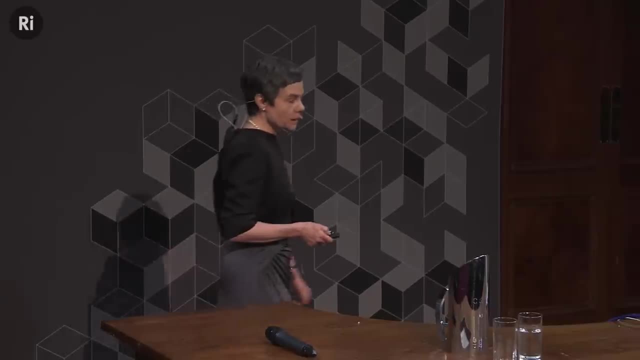 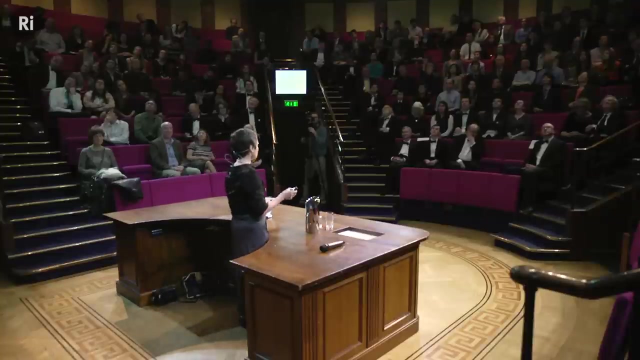 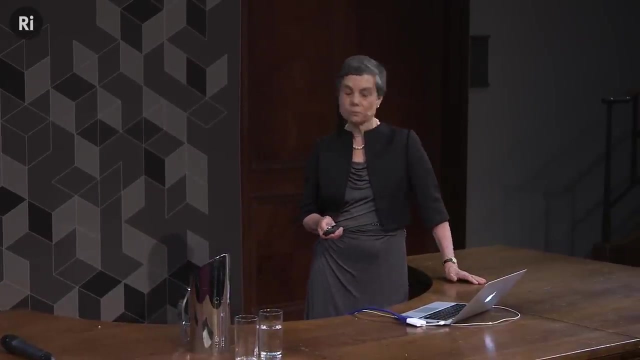 throughout the course of the evening. So what about surfaces then? What can we say about surfaces from this viewpoint of topology? And perhaps by the time I've said it you will have a bit more feeling. So the idea is: we take, it's easier to see a picture. 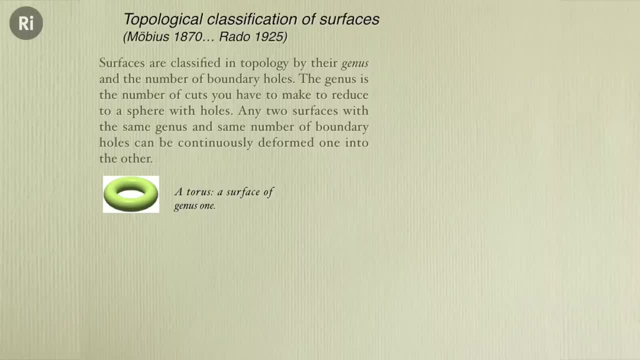 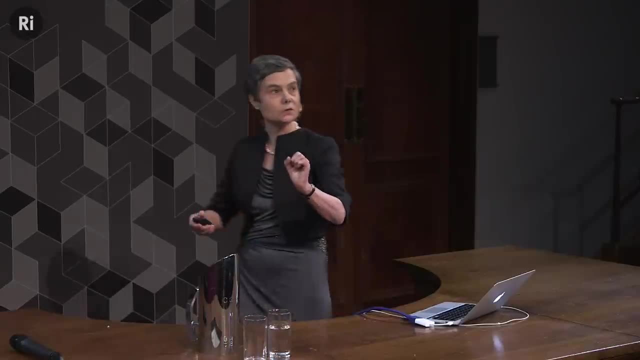 Here's a surface. Now, if you take a loop, a closed loop on this surface that just kind of goes around it once here, and you cut it, of course it'll come apart. And what will it look like in topology? Well, it'll be like a cylinder. but a cylinder is really the same thing. if I took a sphere and I cut two discs out of the cylinder and then I squashed it. So from the viewpoint of topology, if I make one cut through this thing, I get a sphere with two holes. 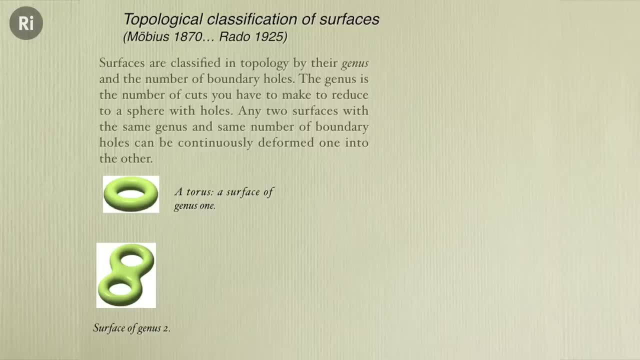 And if I took this one and I cut each one of the two handle things with a cut- and I opened it out, I would find I had a sphere with four holes. And if I did it on this one, I would have a sphere with. 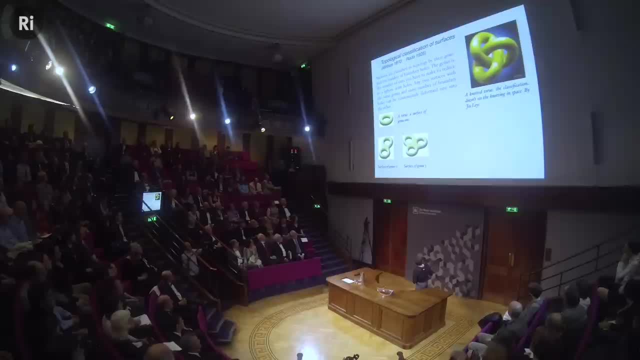 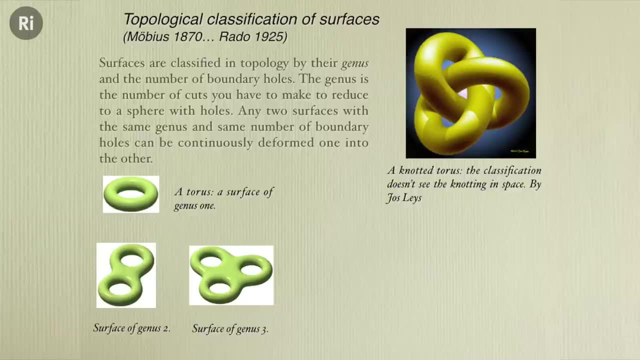 I think six holes. So here's another one. You might think this one is different because it's all twisted up. It's still like this, but it's all twisted up, But it's only twisted up from the viewpoint of how it's been put inside three-dimensional space. 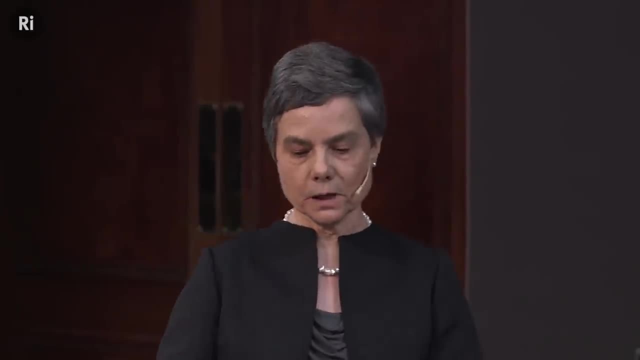 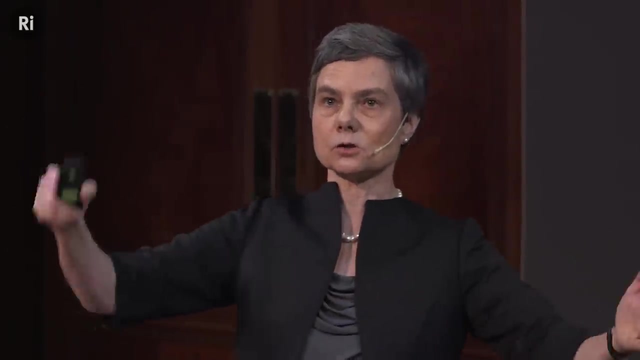 And the classification. I don't know if you know this, but the classification that we're talking about doesn't see how it's sitting in three-dimensional space. Still, if you made one cut, it would still fall apart into this sort of cylinder with two ends. 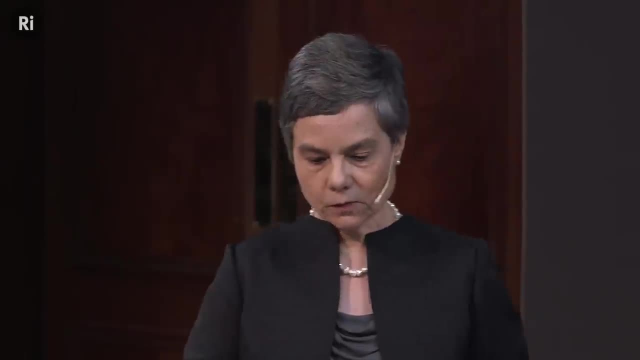 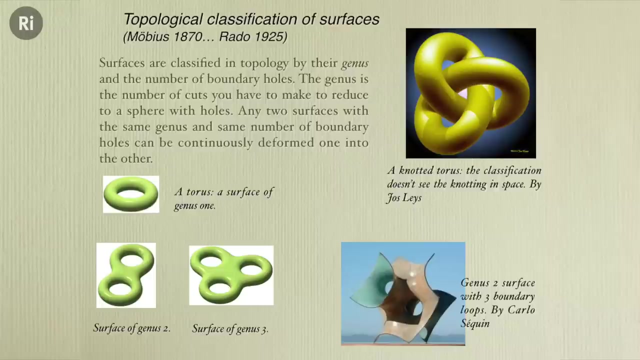 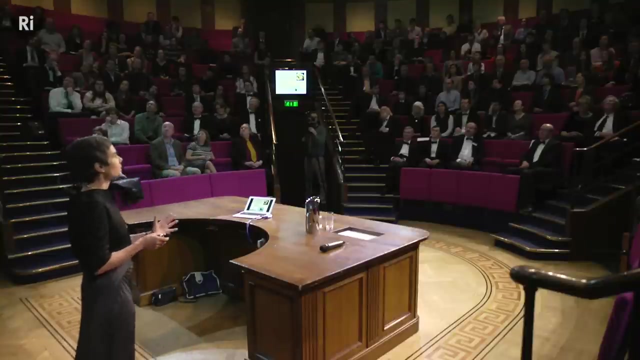 So it's still a torus. So the way we classify surfaces, here's a rather beautiful. I think this is a bronze cast. It's not very large. I think the real thing, Carlos Sequin, is another of these kind of computer people. 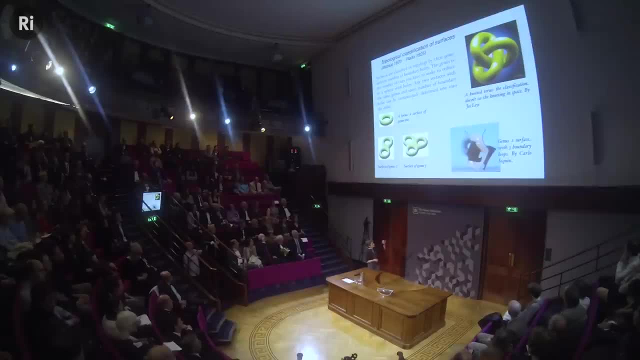 with a very artistic bent, who you know. he's a very, very, very, very, very, very very who makes rather wonderful representations of topological objects. So it's much harder to see this. It's got two. you can see it's got some holes cut in it. 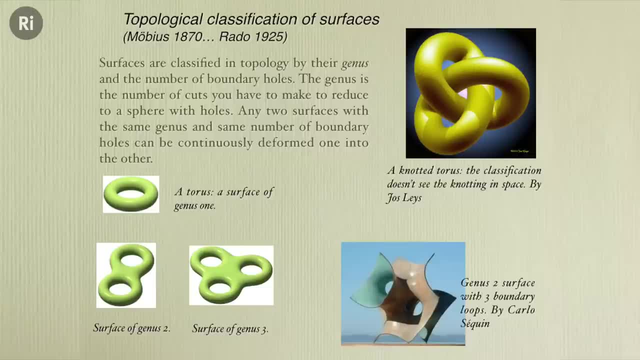 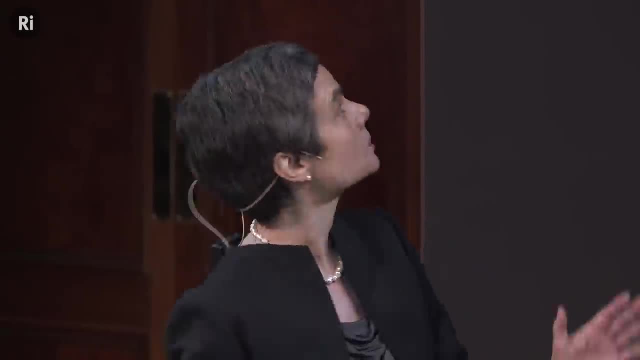 but it's harder to understand. it's got its genus two, but let's believe that's what it is. So that's surfaces, And it took. I've told you this in less than in a couple of minutes. it took a long time to sort all this out. 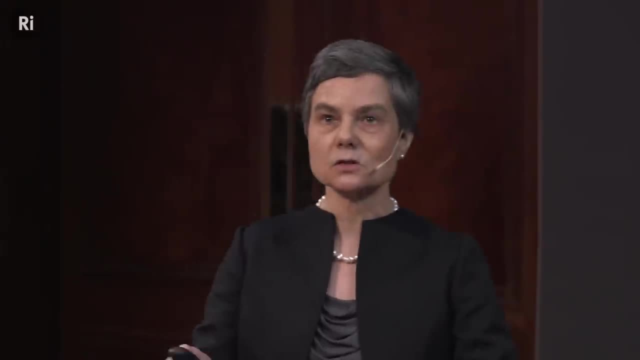 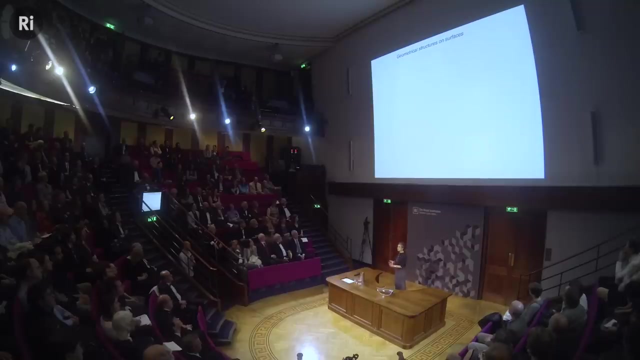 So this is not meant to be obvious. It depends what you think of it. So surfaces to start with. Anyway, that's surfaces Now. we're going to now go into geometry on surfaces. What can we say about geometry on surfaces? 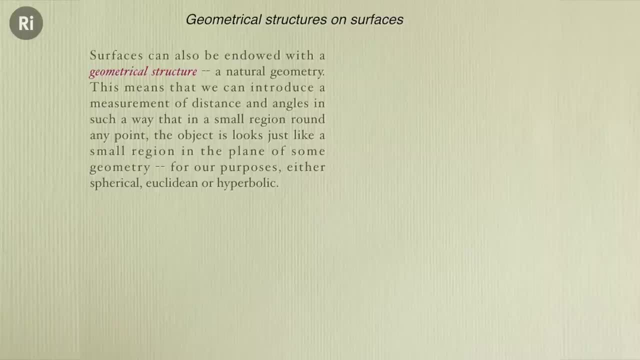 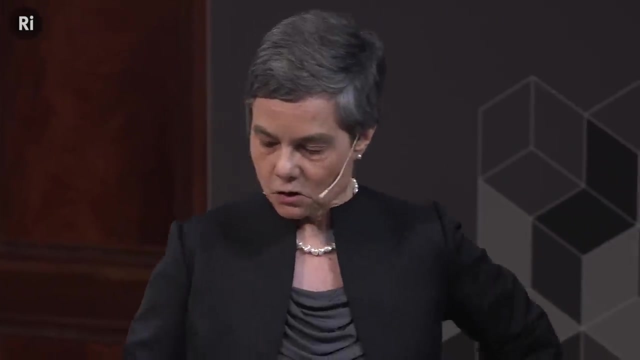 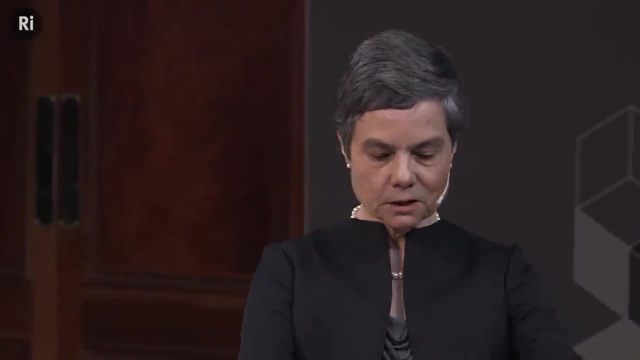 So this is one of the very important ideas in this talk and one of the important ideas in the, I could say, really in the modern study of topology, What's a geometric structure? So, Supposing that I've got some objects and supposing that in a little region, 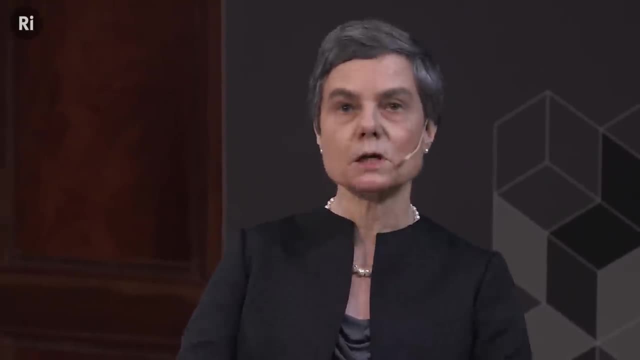 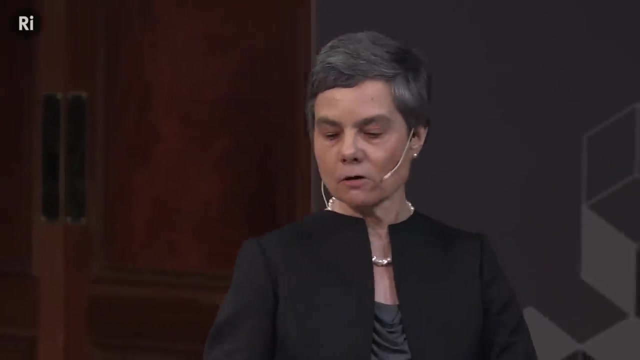 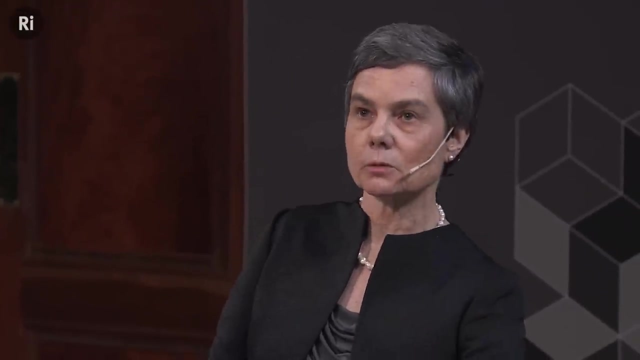 around where I'm standing. I can manage in some way to measure distance and angles in such a way that it looks identical with a bit of one of these basic geometries I've talked about, So it might look a bit like this flat Euclidean geometry. 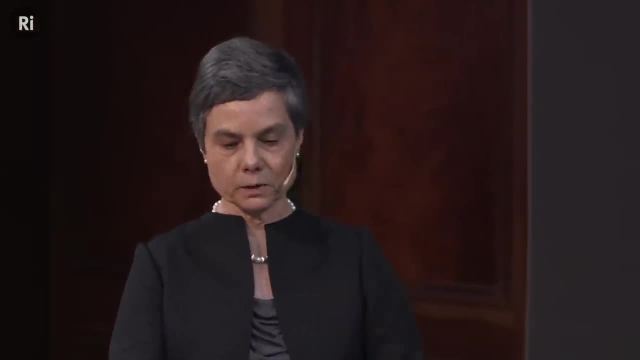 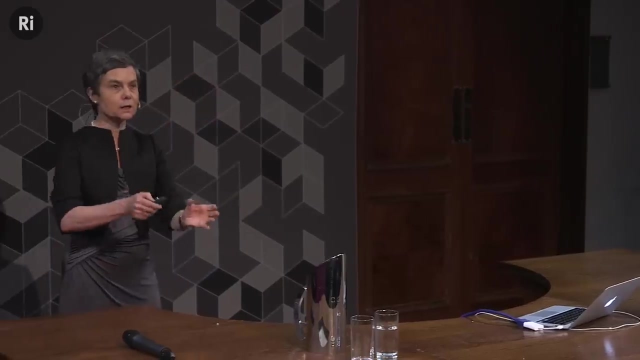 It might look like a little piece of sphere, or it might look like a little piece of hyperbolic geometry, So a sphere. well, everywhere I stand on a sphere and I look around me, I see a little piece of a sphere. 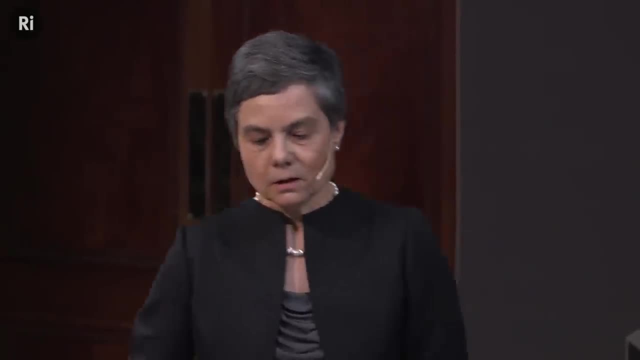 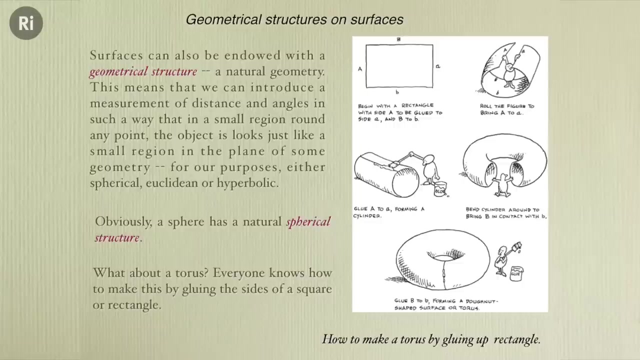 So that's not very exciting. What about a torus? So I'm sure that you've seen pictures like this. You take a rectangle of paper. You glue two sides together to make our cylinder. Here's our cylinder. You pull the two things around. 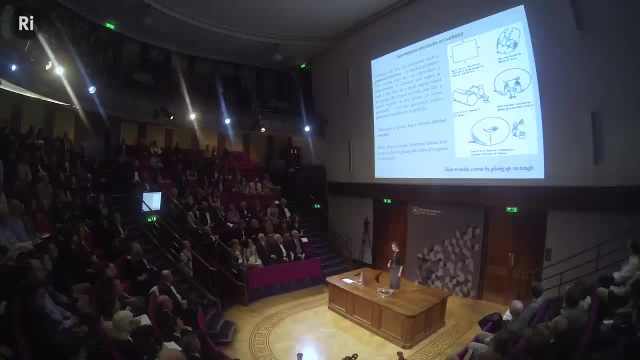 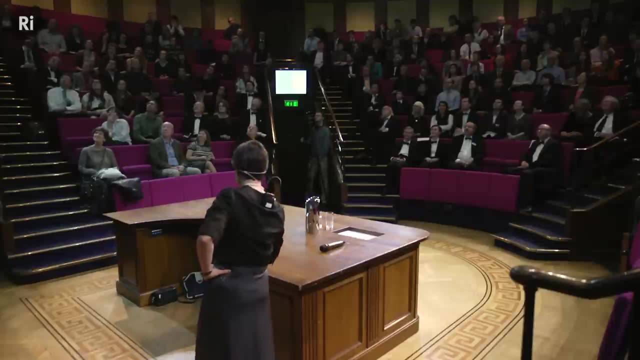 You stick them together And you make a cylinder And lo and behold, you've got a torus. I'll tell you where this picture came from later. Okay, so we can make a torus. Actually, there's a sort of cheat in this, because, of course, 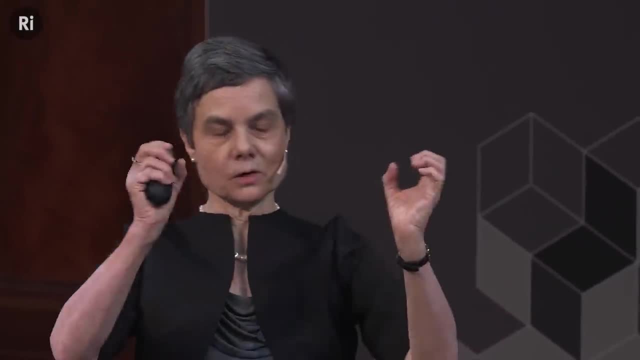 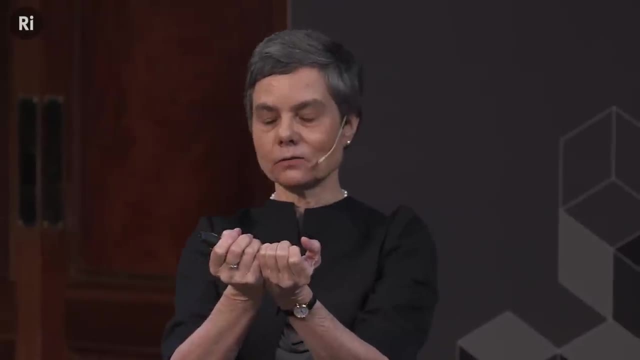 I can roll up and make a cylinder. if I try to do this part. Actually, if I try and do this in 3D, naively, plainly the thing's going to all crinkle and crunch all up. It's not going to work very well. 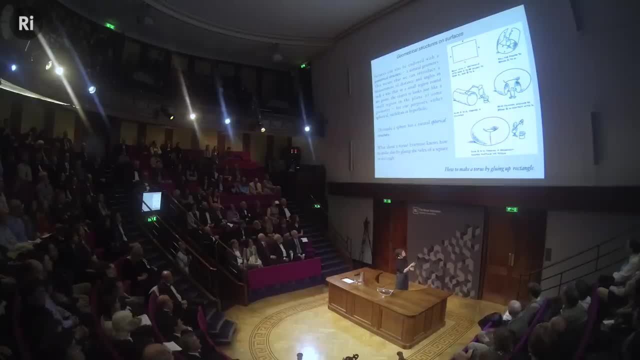 So there is a bit of cheating here, but it's not really cheating, because what I'm talking about is what you would see if you were a fly. This is a kind of abstract concept, if you like. If you were a fly living here, well, actually, or if you even was a fly. 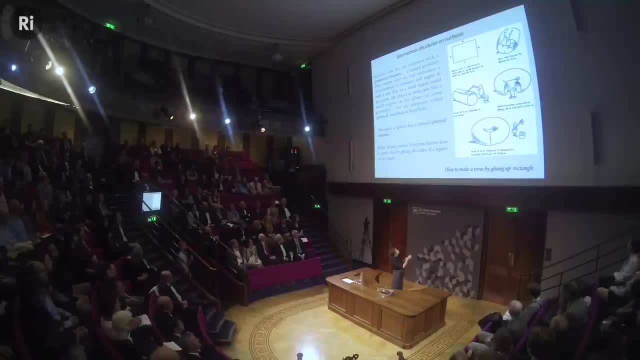 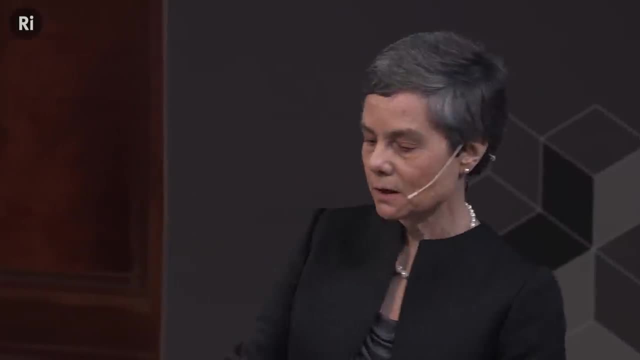 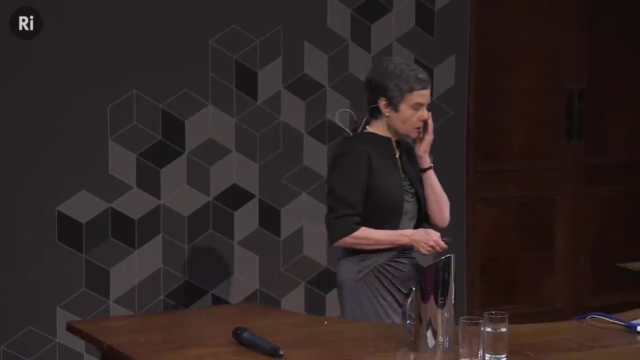 and you walked across this line. it would be no different from going across here and then coming back in here. So somehow there is a meaning to saying. this thing is basically coming from a rectangle cut out of Euclidean geometry, So the torus has got Euclidean structure. 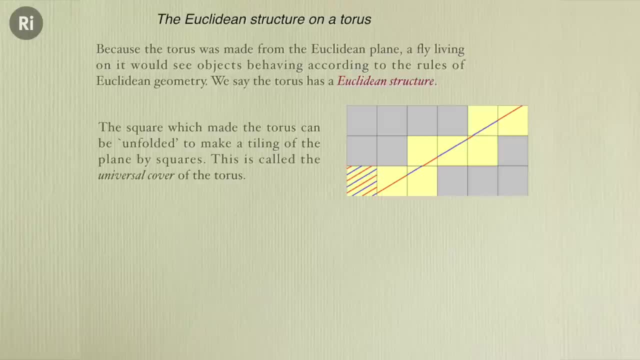 So here's a picture: I take my square, but then if I went across this side I kind of unfold it and see another copy of the square, and another copy, and another copy. Really I translate it, but let's not get too detailed here. 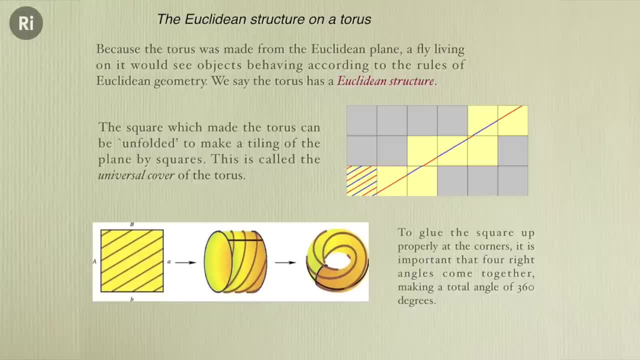 So you can. so here is another picture. Here's another picture of gluing up the top. Okay, This torus. and there's one very crucial feature in doing this: that it was very important that when I glued- well, first of all, 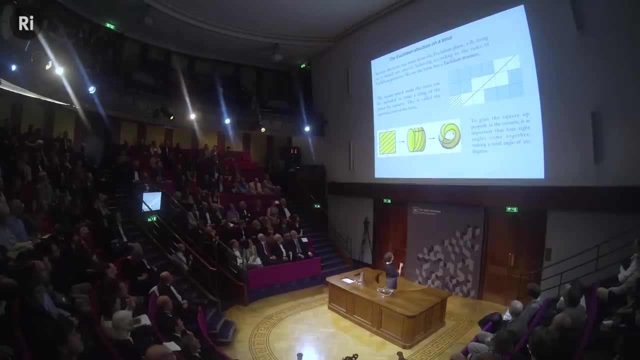 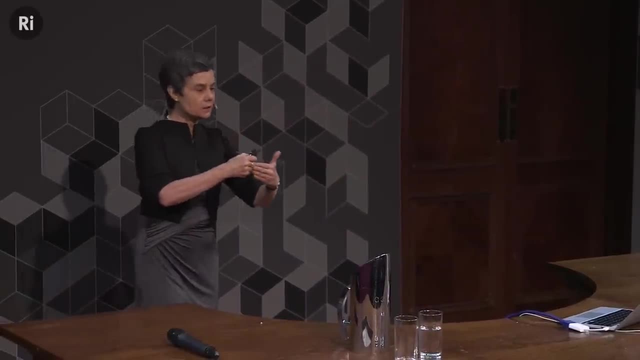 when I glued from here to here that this plus that were 290 degrees, so they made 180 degrees, so they met at a straight line And then when I put the two ends together I've got two lots of 180 degrees. 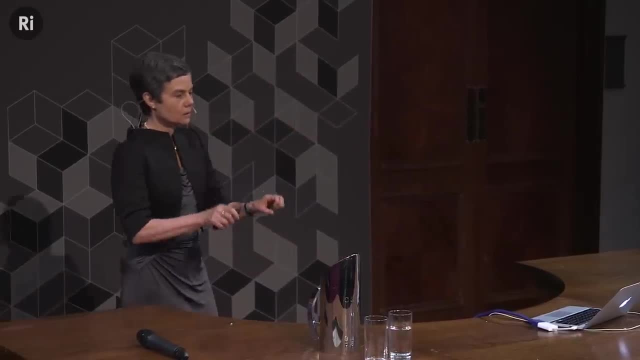 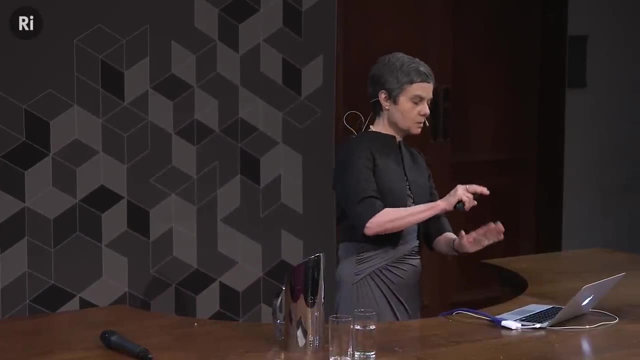 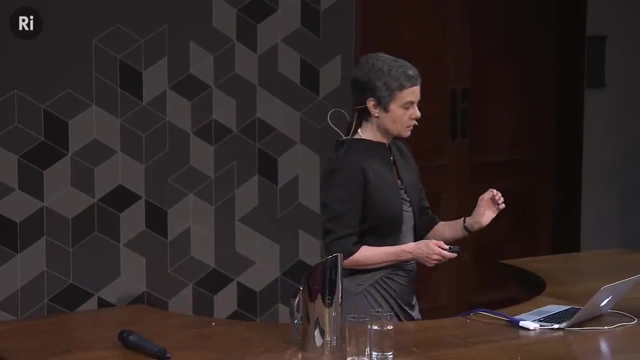 And that's Well. those add up to 360, and that makes a nice smooth, flat piece. It makes 360 degrees and that's fine. So there is what we mean by saying a torus has a Euclidean structure. 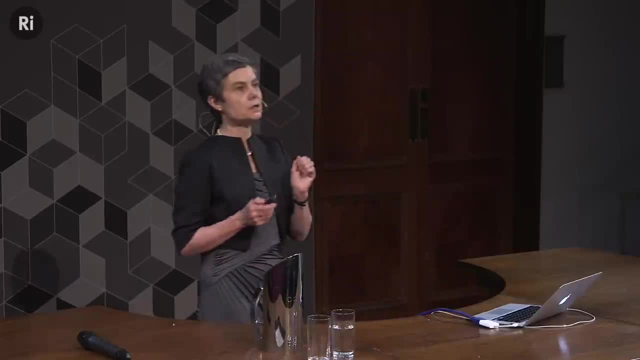 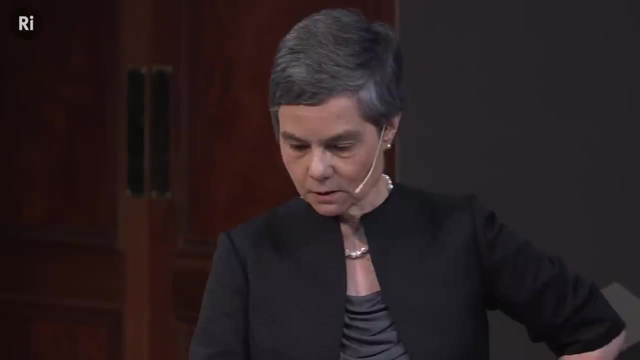 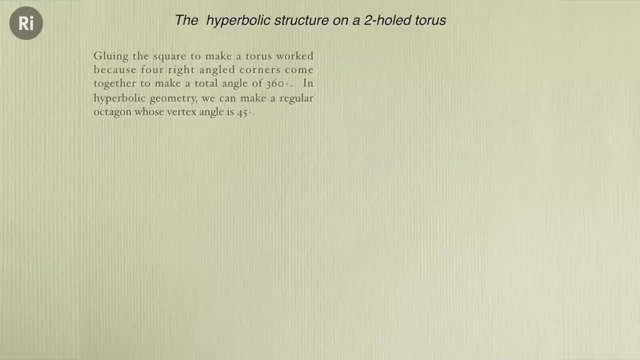 So I've somehow, to this surface, attached a natural notion of Euclidean geometry. Well, what happens if I know that the torus has a Euclidean structure? I now go to a surface which has got two holes, genus two. So here is a picture. 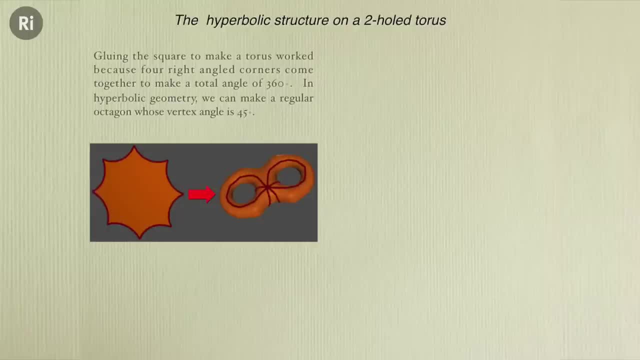 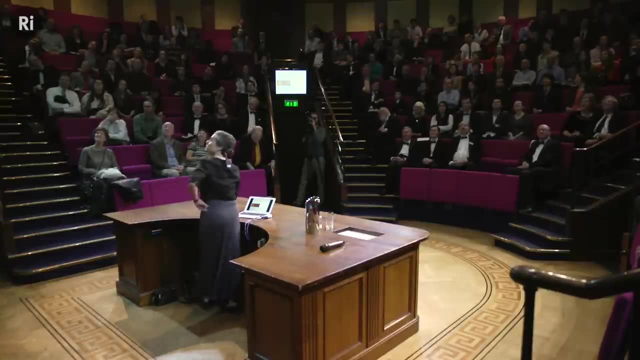 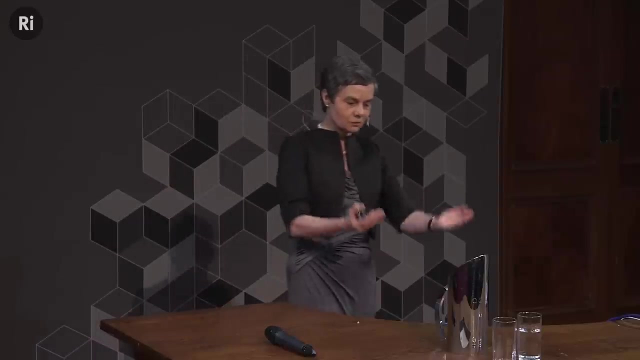 If you follow through this, if you were to glue the opposite sides of this thing together, you can go home and puzzle about this for a long time. But it is true, I assure you that if you glue the opposite sides together, you're going to have to kind of come around yourself, maybe go through yourself. 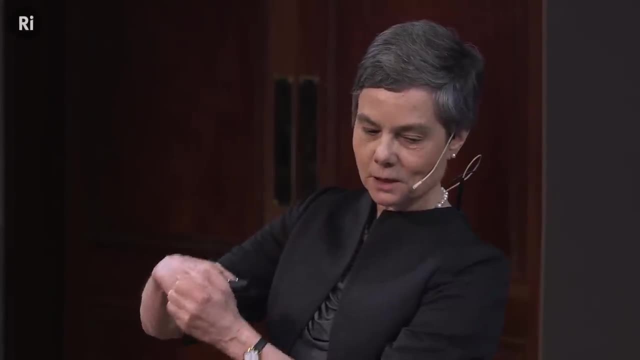 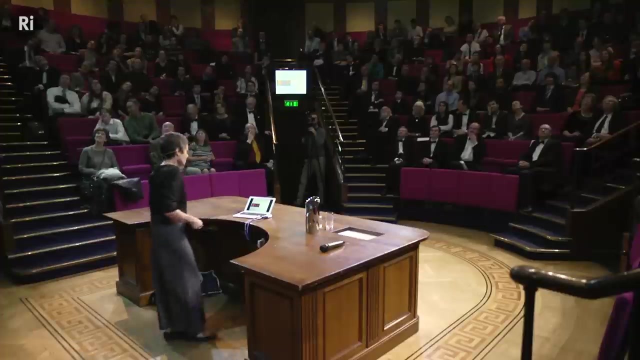 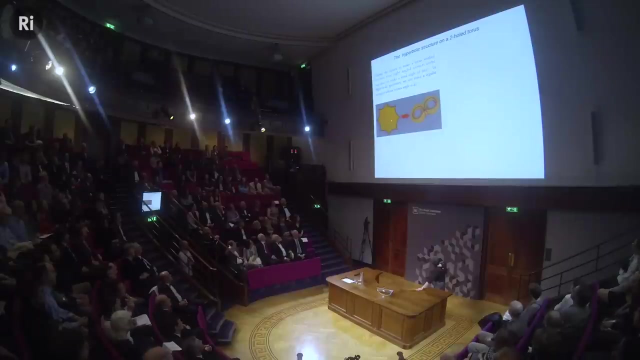 depending how you do it, but you should, in the end, be able to convince yourself that if you glue it up, you come out with a thing like this. Okay, So let us believe that. But the trouble is, if you took an ordinary octagon, 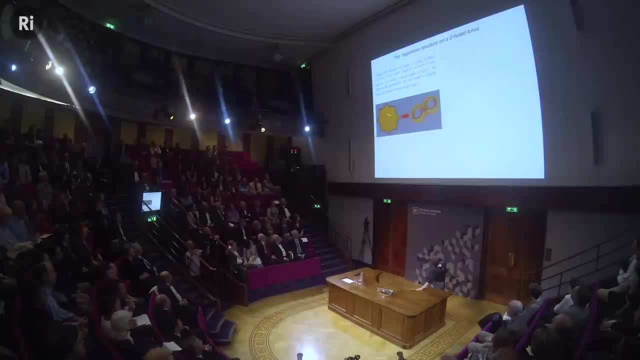 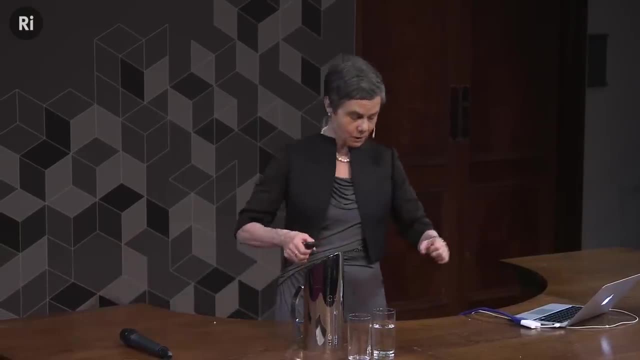 then eight of these corners have got to meet up here And whatever the angle in an octagon is, I think it's 135 degrees. Anyway, if you glue, If you glued them together, there's no way it makes 360 degrees. 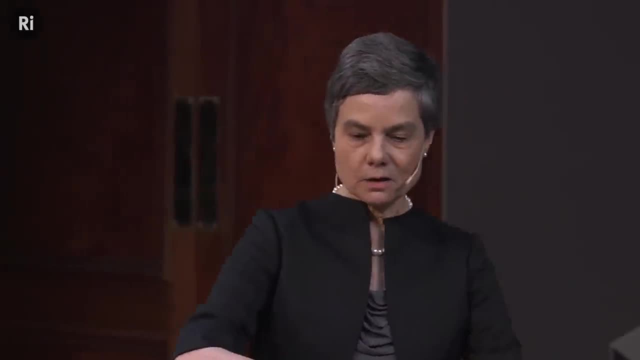 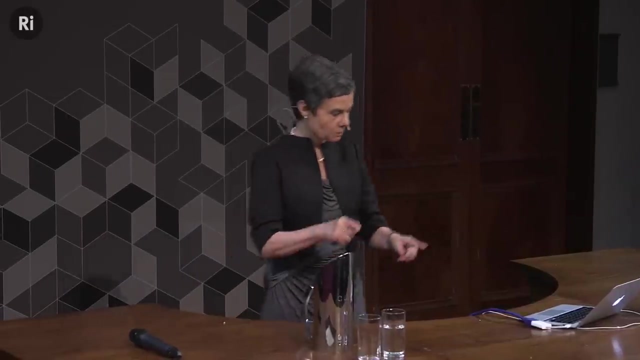 It's way, way more. It's too much, So you glue them together and the angle is much too big. so you haven't got a nice Euclidean structure, because if you try and cut it out of a piece of paper and glue it up, 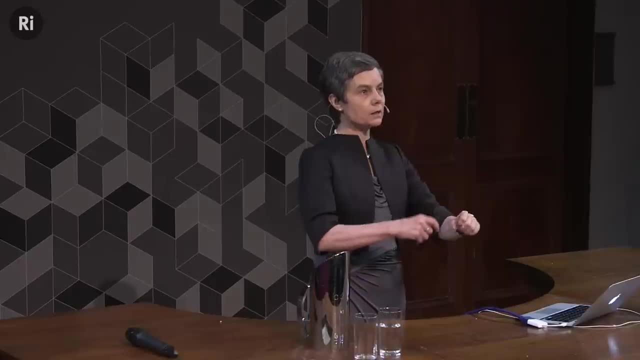 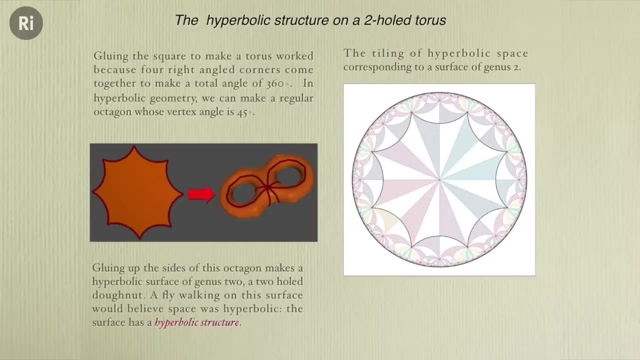 at the last minute, you'll have a nasty mess in the middle, where it doesn't fit together flat. So what are you going to do about it? Well, you remember that in hyperbolic geometry the angles in a triangle don't have to add up. 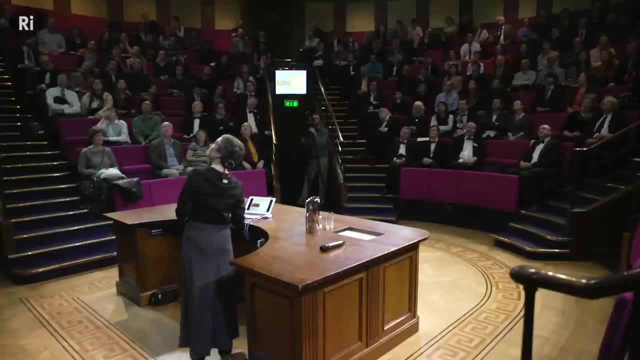 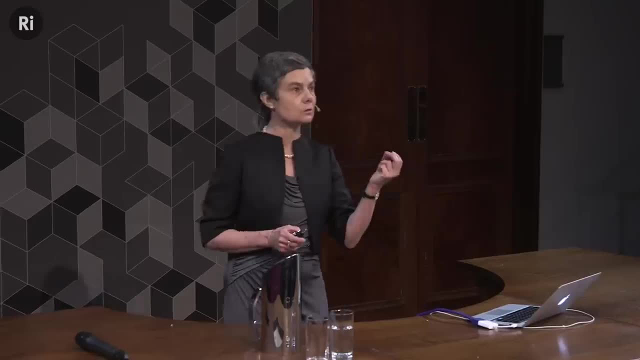 or don't add up to 180.. They add up to something less than 180. And actually you can create triangles whose angles add up to anything you like, less than 180.. And here is a rather beautiful tiling of the hyperbolic plane. 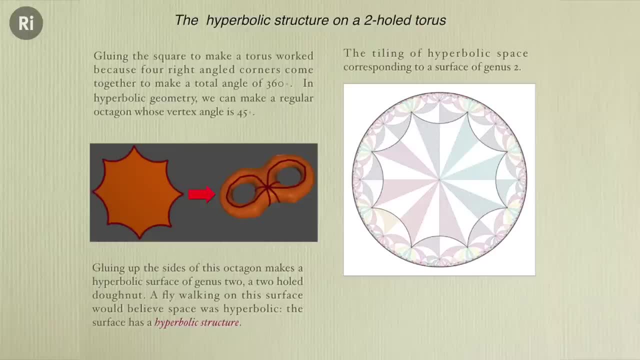 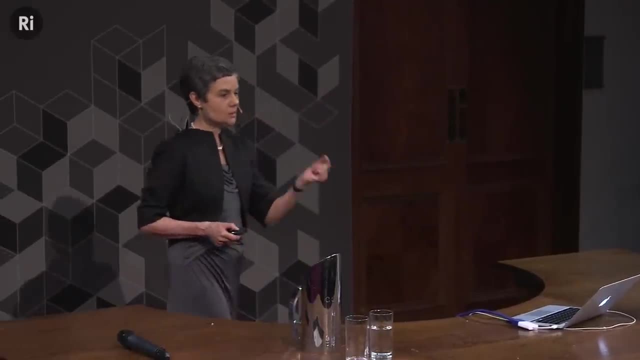 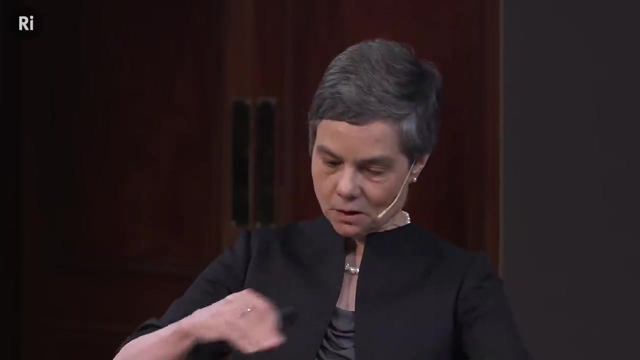 in which we've got a nice regular octagon and the angles here have been manufactured each to be 45 degrees. so when I stick eight of them together, lo and behold, I make 360 degrees. so it's nice and locally making the right angle that it should do. 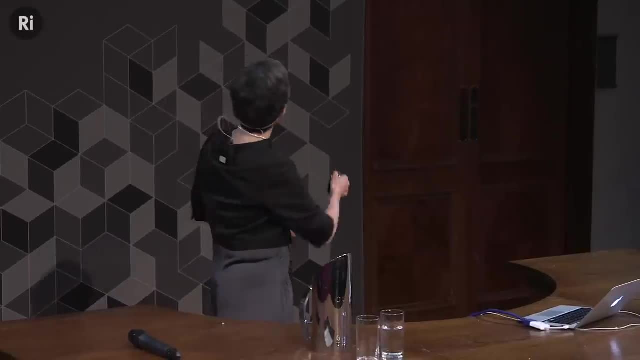 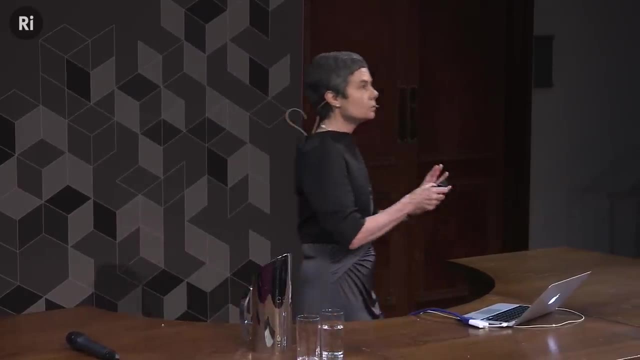 And so I've created a surface. If I could cut this piece of paper out of hyperbolic paper which has got this kind of curvature, and if I could stick them together, I would have created a surface of genus two And actually. 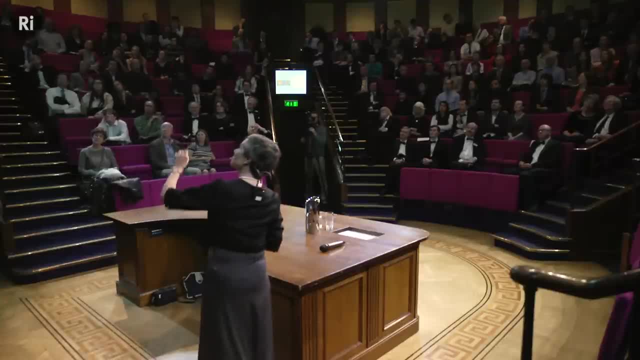 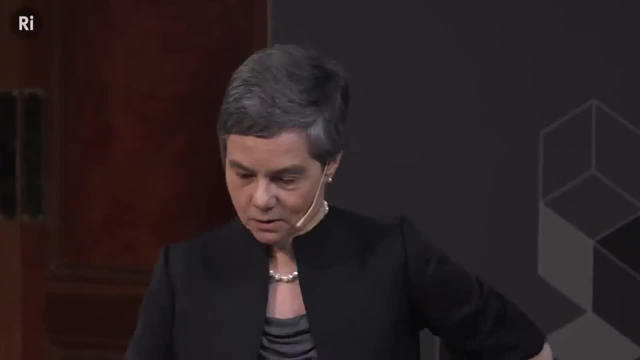 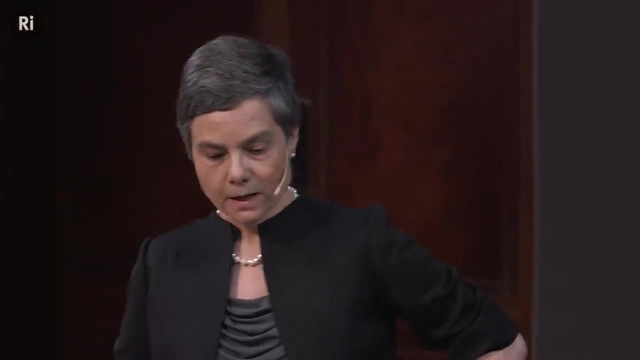 by just adjusting the angle. using this trick, you can make a surface of any higher genus you like, And this was, I suppose, known and understood. It was being studied a lot in the 1920s And you might say, well, so what? 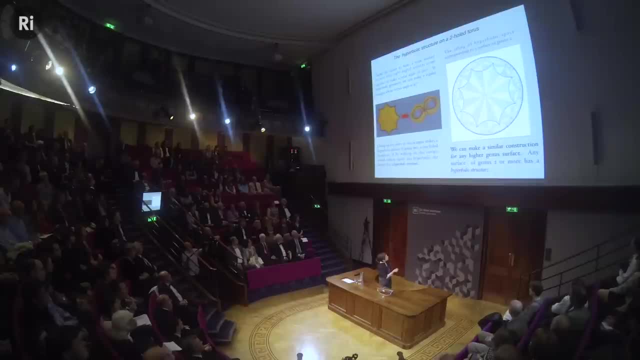 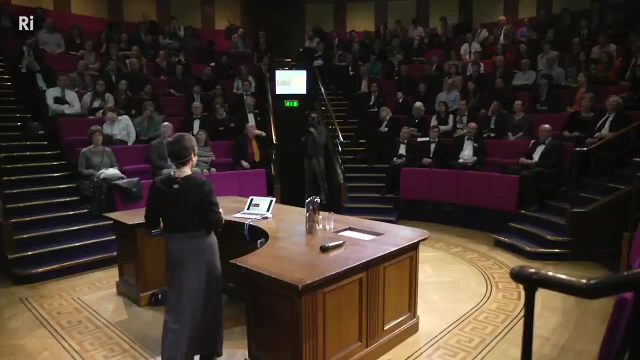 Actually it became very important because anything you want to study about this surface, you want to know what closed loops are on it, and you want to know what closed loops are on it. So, somehow, if you look at this pattern, this rather complicated but beautiful pattern, 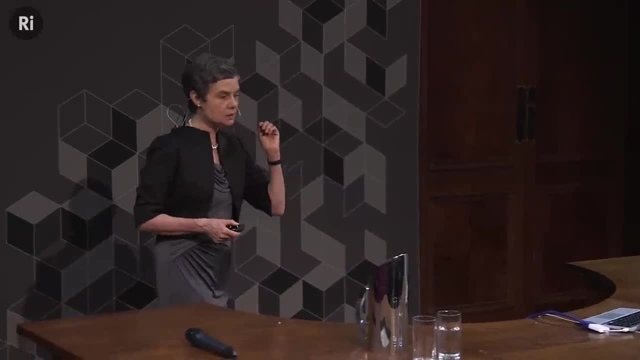 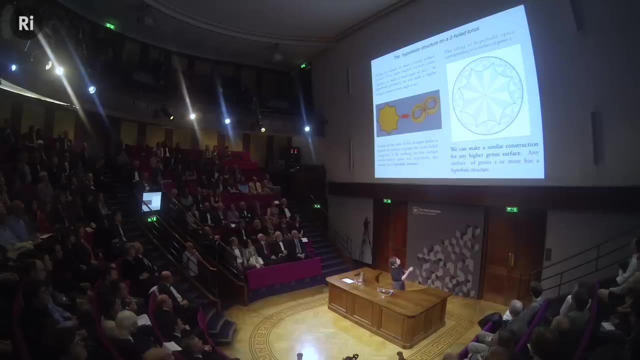 you can read off all sorts of things here, and one thing you can do is you can study particles sliding around on this surface and it turns out that by studying the intricacies of this pattern and by realising that things geodesics in this hyperbolic plane. 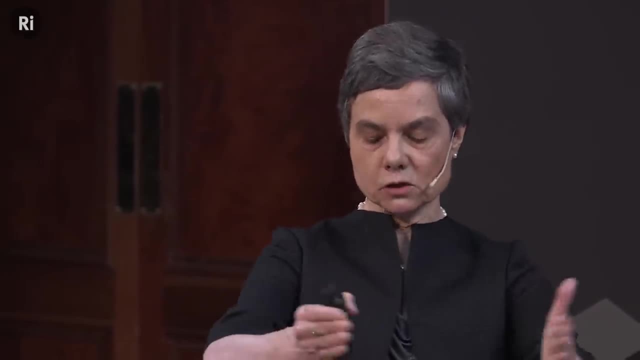 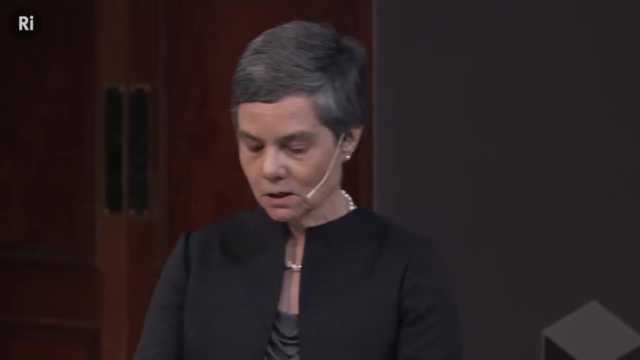 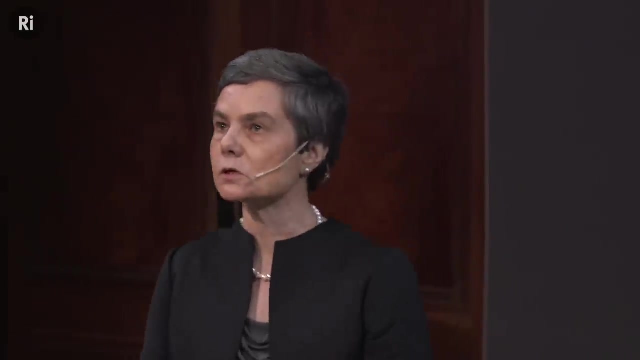 they come close together and then they kind of diverge from each other, and that's the essence of chaotic motion. So sliding around on one of these surfaces is a prototype for what we now call chaotic motion, and this was one of the first examples that was really studied. 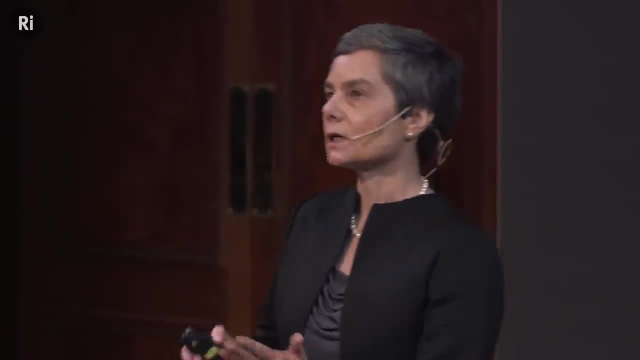 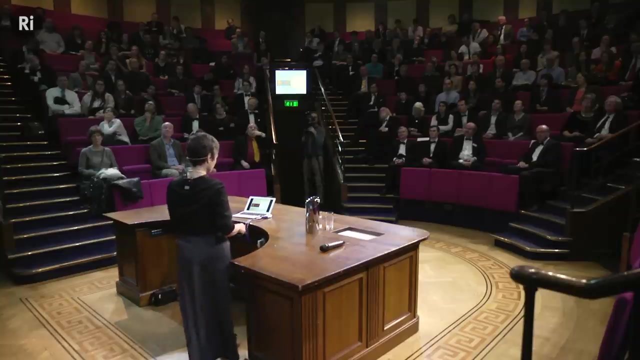 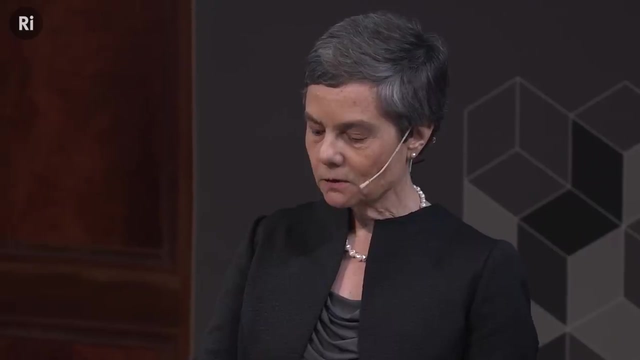 and introduced the idea of randomness and chaotic motion, but by a perfectly well-defined formula. So this was in the 1920s and probably 1930s for that. So let me just recap very fast: We have learned that we know. 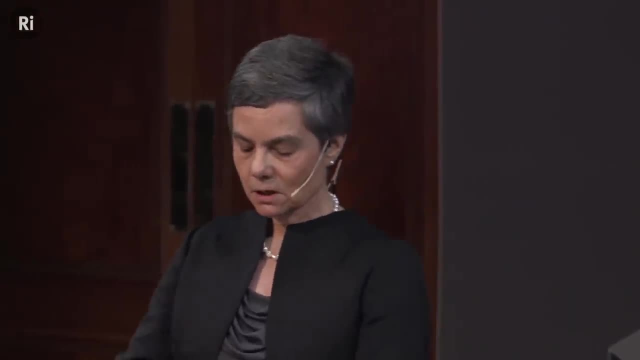 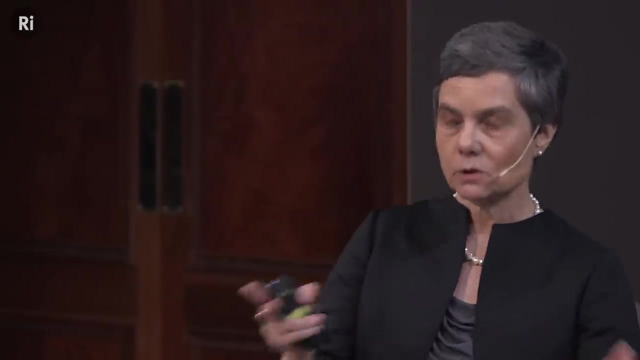 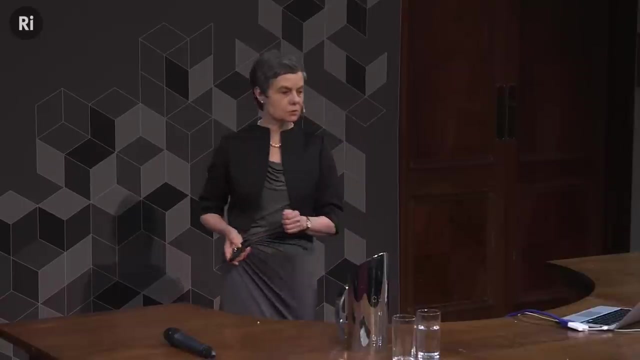 how to classify surfaces, and every surface, in a natural way, has got a geometry on it. It's either like a sphere, or it's like a piece of Euclidean plane, but usually it's like the hyperbolic plane. So now we are set to proceed into three dimensions. 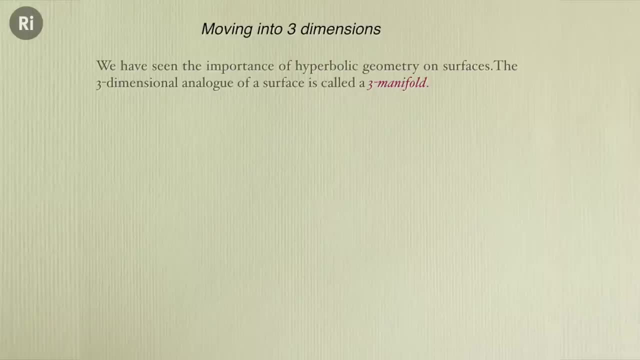 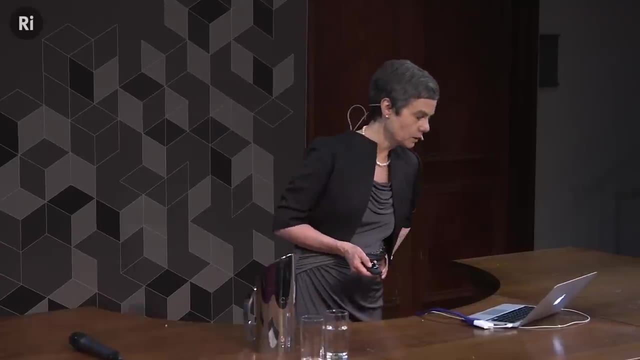 So my first problem in this is there is not a normal English language word for the 3D analysis. It's an analogue of a surface. Nobody has yet come up with a very good word, So a thing that's an analogue of a surface. 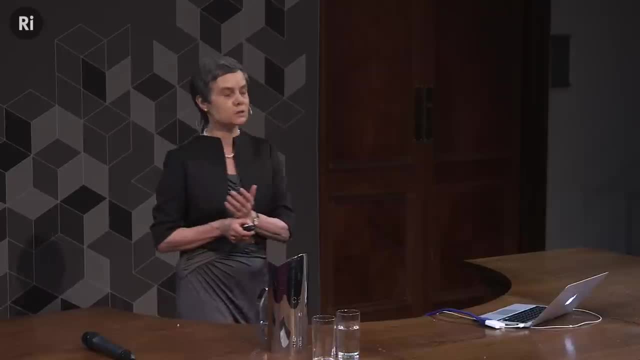 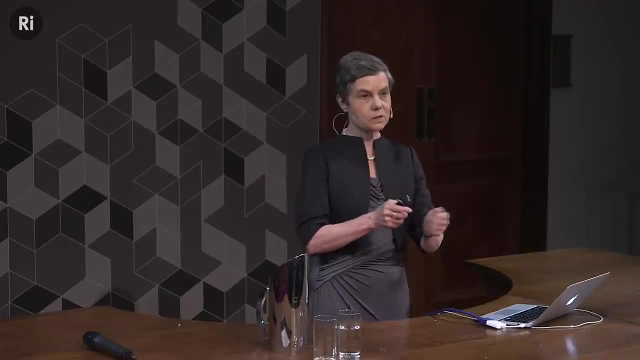 but in more dimensions, is known to mathematicians as a manifold. So we talk about a three manifold. So what it means is, everywhere you look in a little bit, it looks like some sort of very squashy, vague version of three-dimensional space. 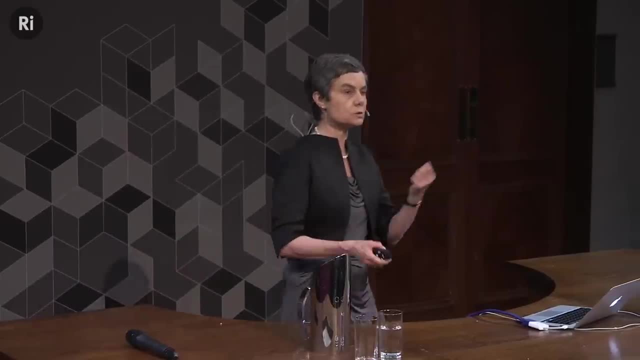 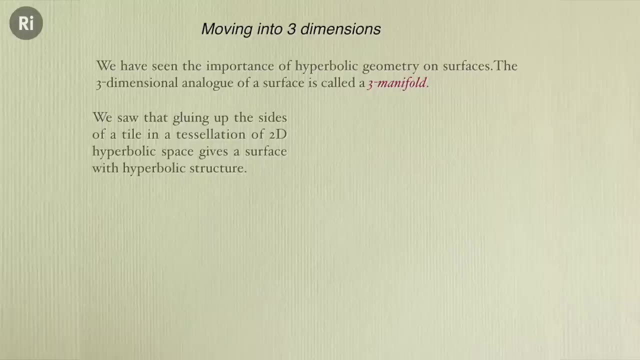 but it's got all sorts of complicated loops and tubes and holes and goodness knows what in it, So some very complicated thing. Well, we've just seen how to make a surface by gluing up the sides of a hyperbolic octagon. 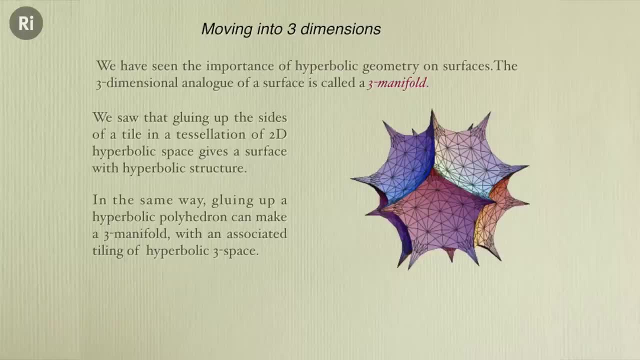 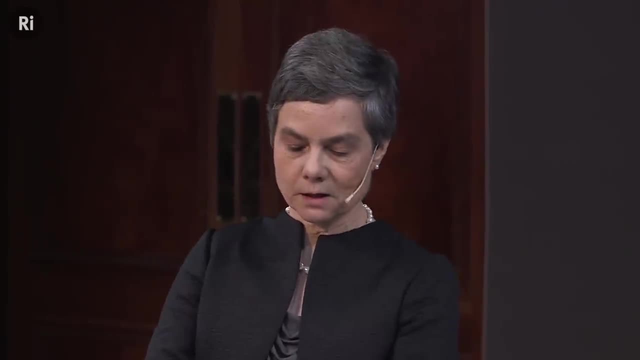 So supposing we took a hyperbolic polyhedron and supposing we glued up the faces, if we were lucky we could fix the angles, so it would all work and they'd fit round. they'd have to fit round the edges, nicely. 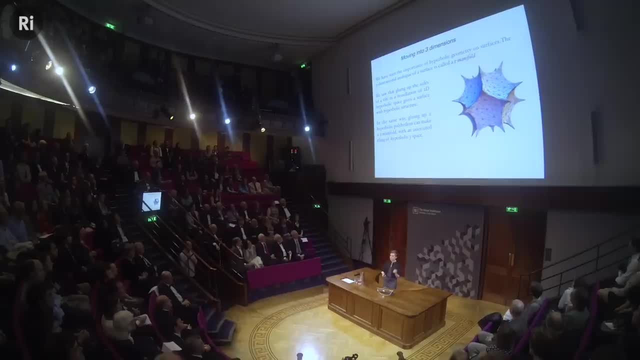 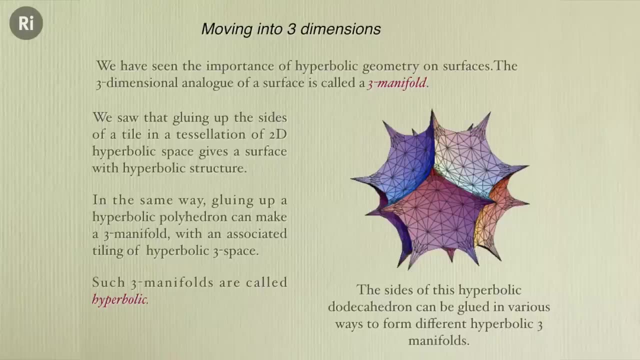 and they'd have to fit right at the corners. but if we were clever we might be able to do it And we might be able to produce one of these three-dimensional objects which, just in the same way that we glued up in 2D. 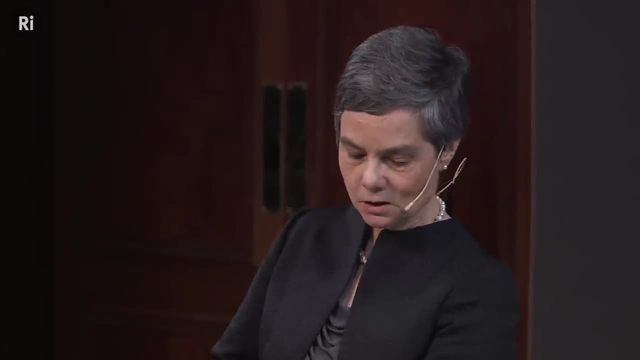 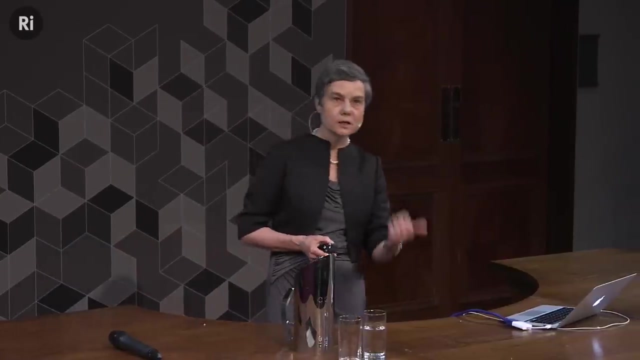 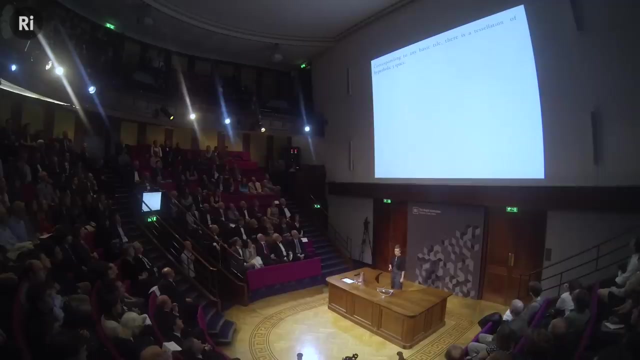 and created a surface of some genus. we can create something in 3D which we can say has a hyperbolic structure and comes from this process, And now we come to some really amazing pictures. Just as in 2D, we could tile, we could kind of unfold the thing. 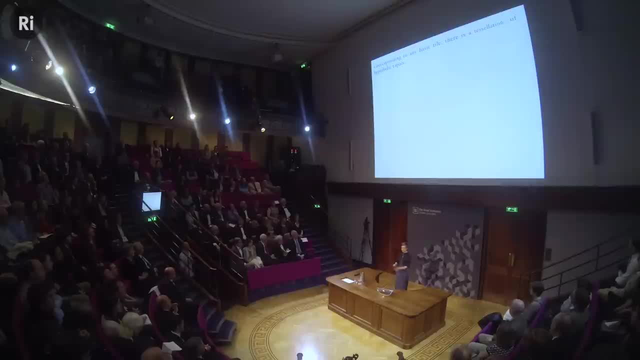 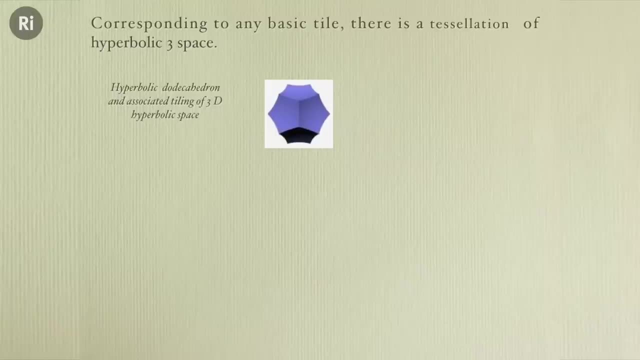 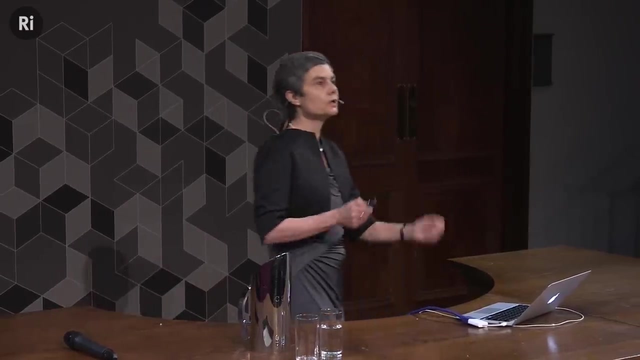 the torus into a square tiling. So in 3D, we can start with, for example, this, which is the same as the one on the previous slide, and we can unfold it into a tiling of three-dimensional space. 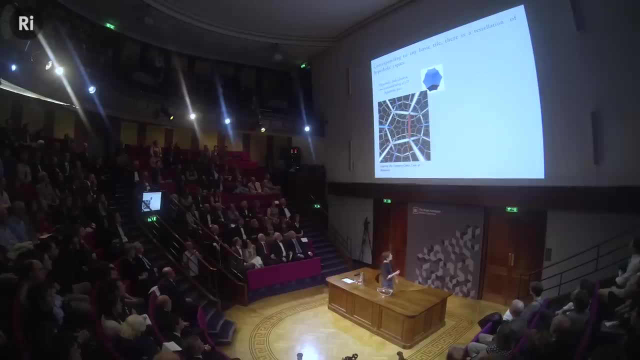 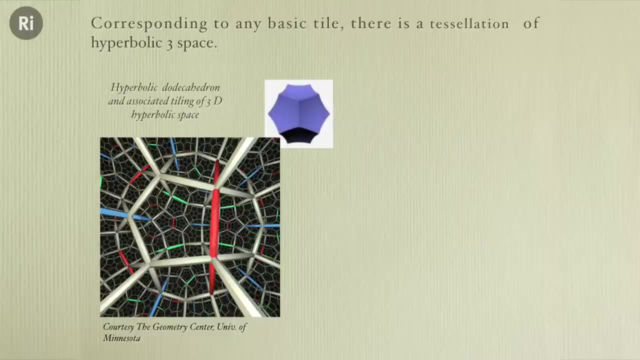 So I don't quite know how to make a drawing like this. I think it's amazing, But anyway. so here we are. We've got the. The walls of this thing have been made transparent so you can see, and you're sort of seeing through to the cells. 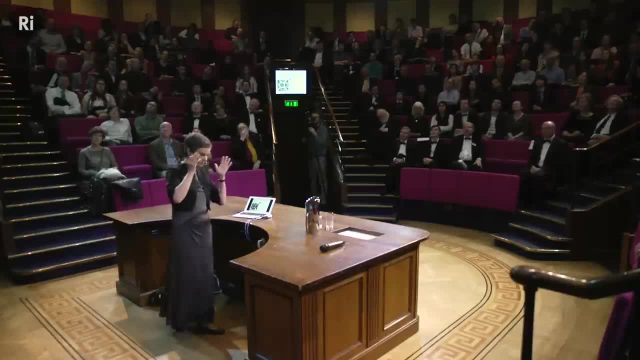 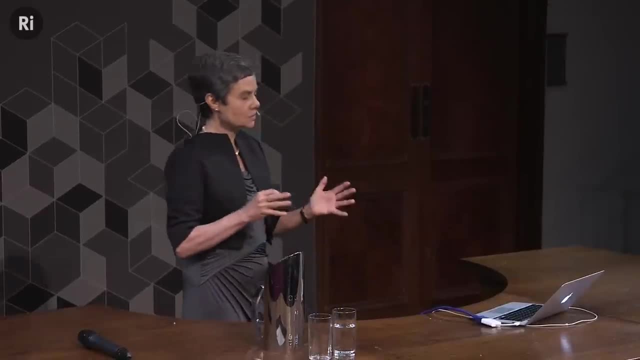 if you like So imagine. You could imagine a sort of cubical tiling of ordinary Euclidean space. This is an analogue in hyperbolic space, And Joss Leys- Joss Leys, by the way- has a rather nice website- 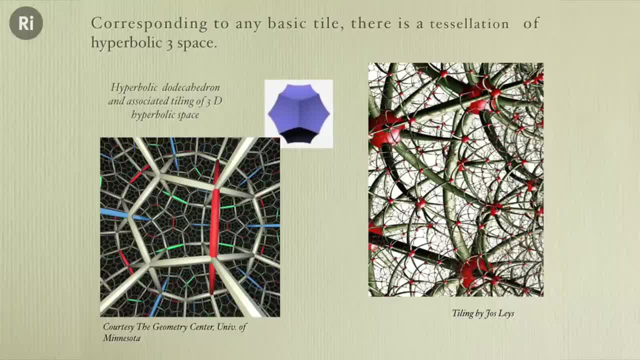 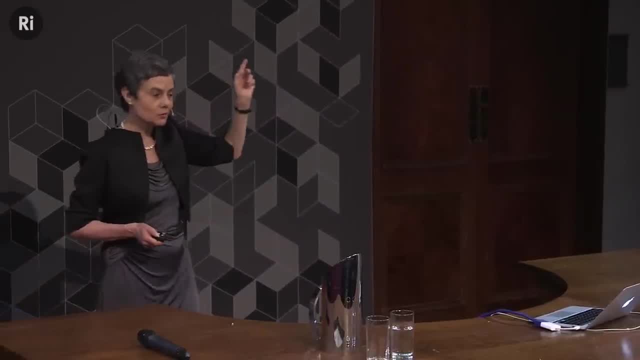 with all sorts of pictures. In particular, there's a whole section of rather wonderful tilings of hyperbolic 3-space. Okay so, hyperbolic geometry in 3D? well, it produces some pretty pictures, Okay, Right. 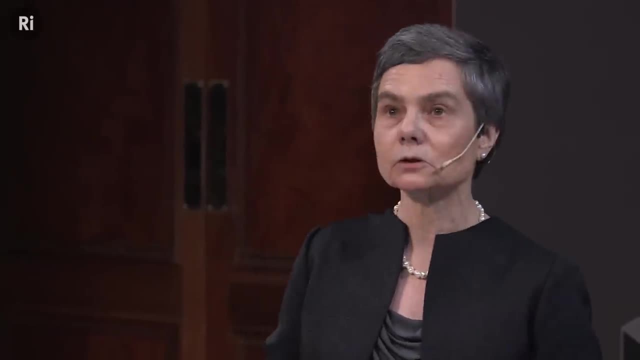 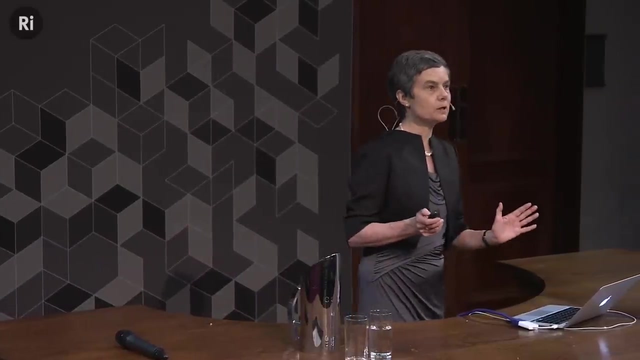 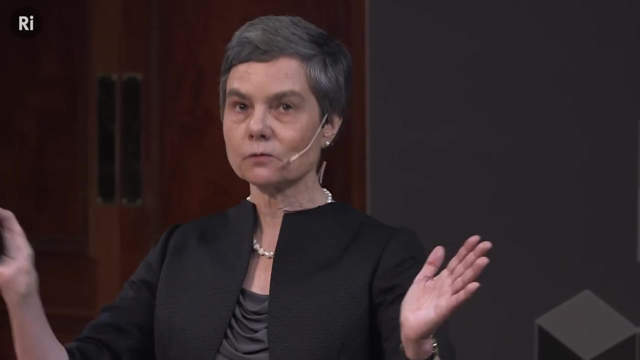 Okay, Before I can go on, I have to give you an alternative viewpoint. If you go back to my original picture about hyperbolic geometry sitting inside the Minkowski space of special relativity, if you look out to infinity along the light cone, 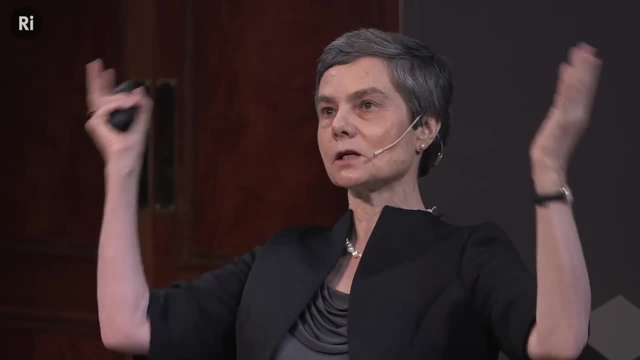 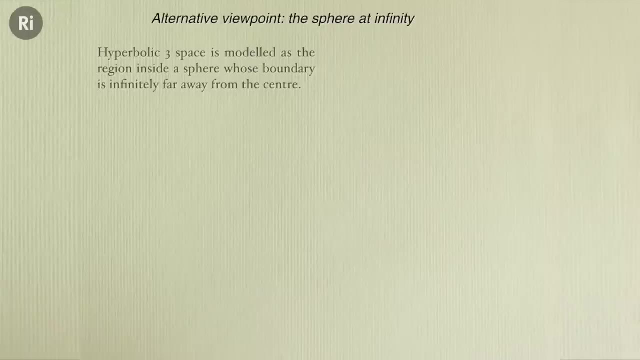 you see a sort of In 2D, you see a circle. In 3D you'd see a sphere of stuff that's way out at infinity. And I also said we can model two-dimensional hyperbolic space as the inside of a disk. 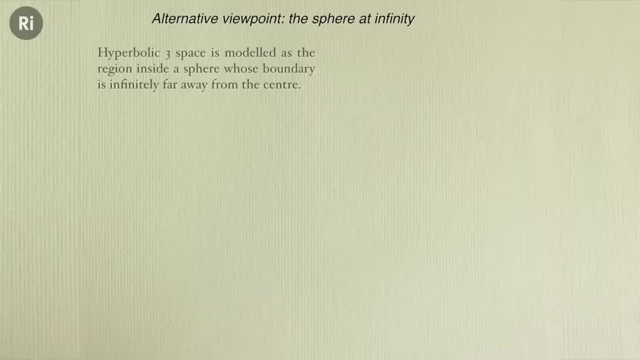 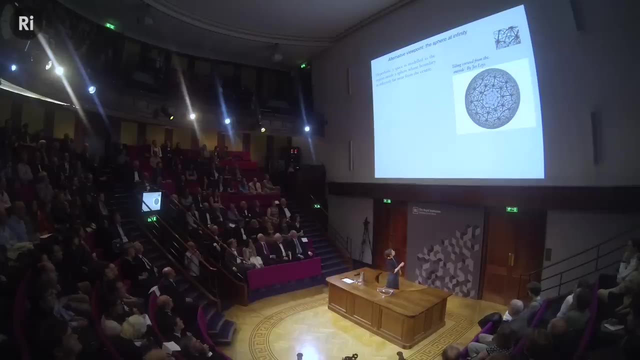 So, not surprisingly, you can put 3D hyperbolic space inside a sphere. So far, so good. So here is a picture. another picture by Joss Leys: This tiling that we saw you could stand. 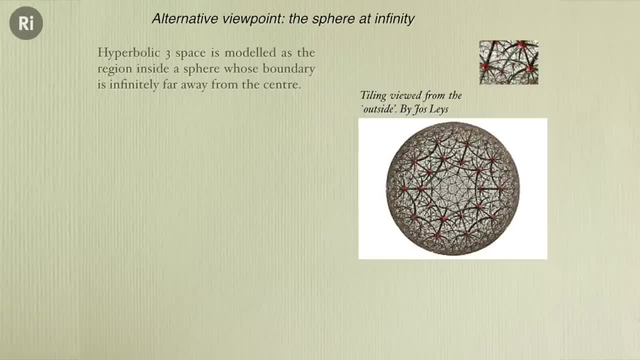 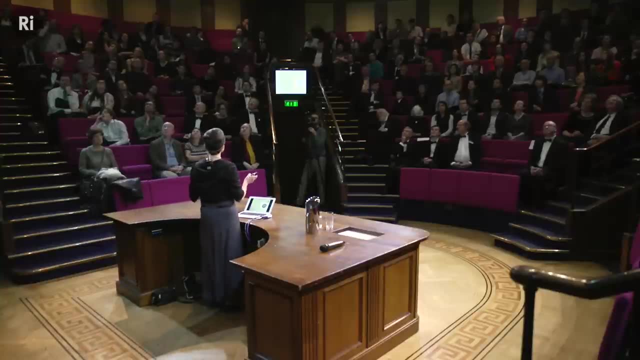 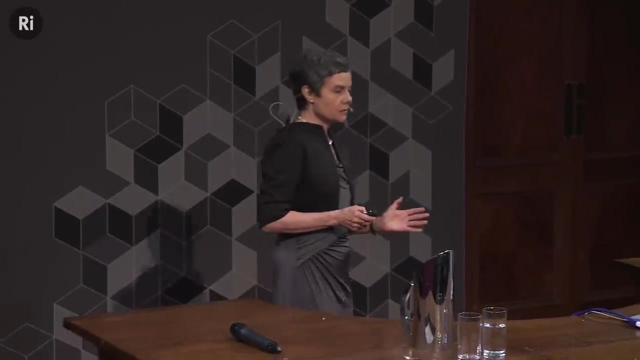 sort of on the outside of the universe and look in and you would see something rather wonderful. like this, Poincaré, I guess, when he was working with these Lorentz transformations of special relativity, realised that the isometry is a word I haven't used. 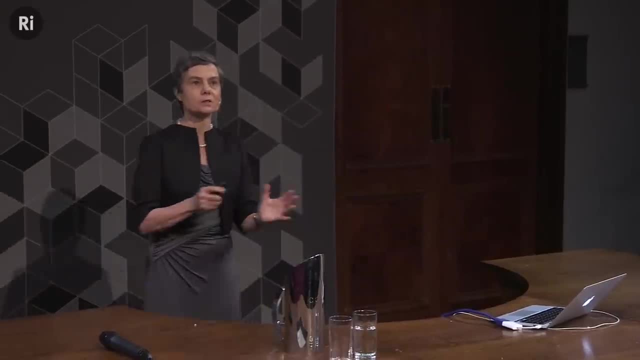 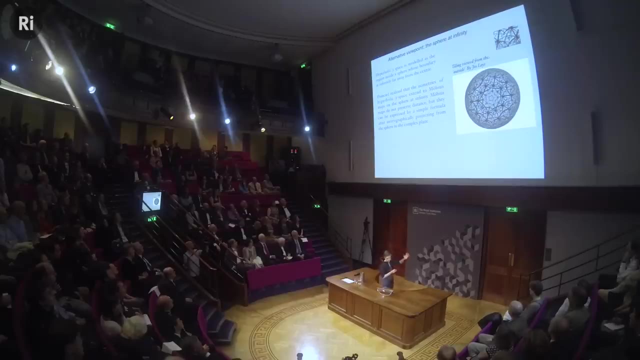 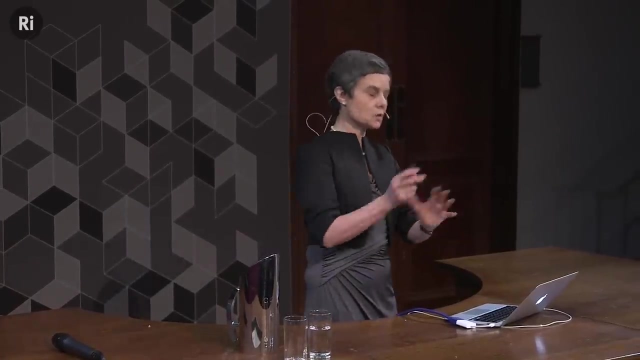 Isometry means a rigid motion, a congruence, Things that are like congruences in Euclidean geometry. So isometry means keeping the distances the same. So we have something, a rigid motion inside hyperbolic space that's moving tiles to other tiles. 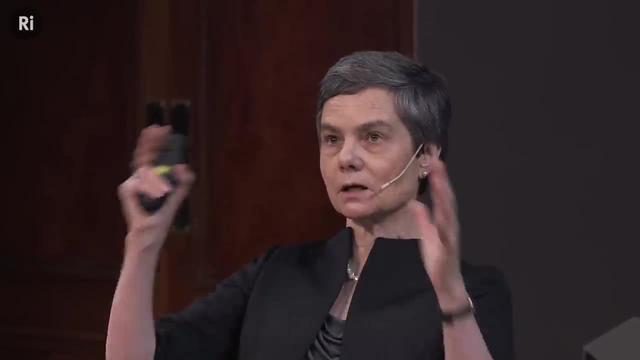 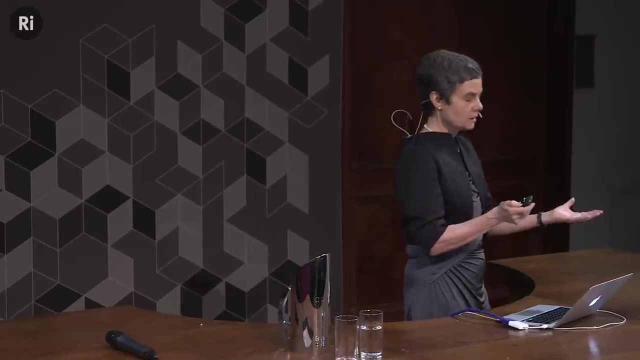 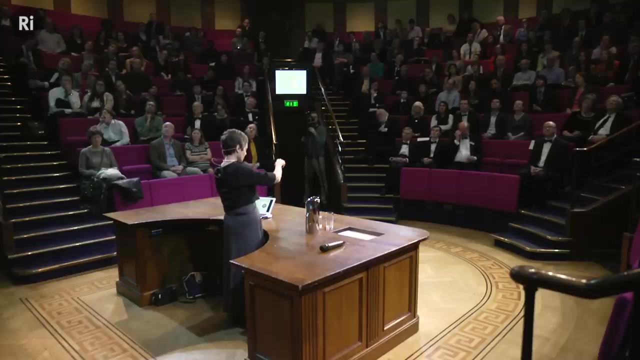 but actually it does something to this sphere at infinity And on this sphere at infinity you can calculate the formula. Now, it's a formula on a sphere, but no doubt some of you know how you can think of the sphere: you can project it from the top. 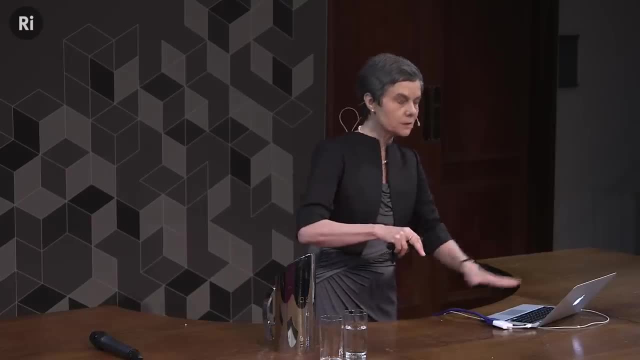 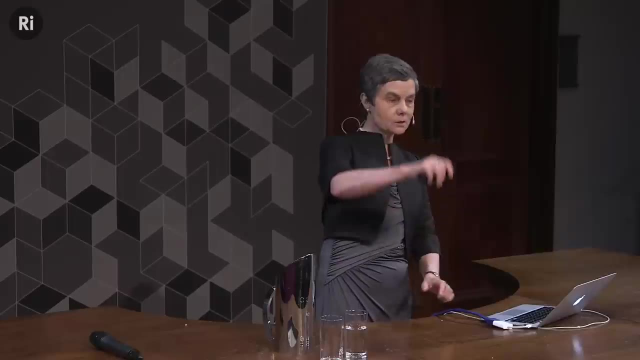 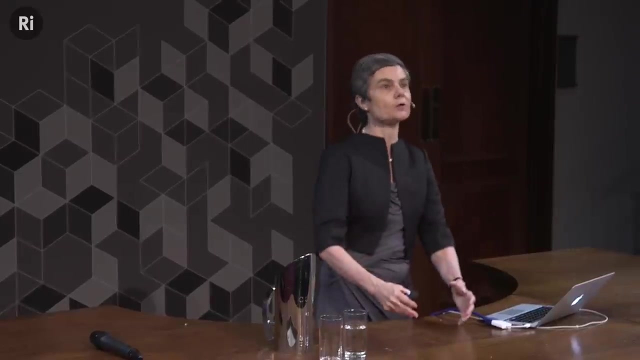 onto the plane and you can think of the plane in terms of complex numbers, X plus IY, and so if you take the plane together with one point- point at infinity- you've made a sphere. It's really like stereographic projection. 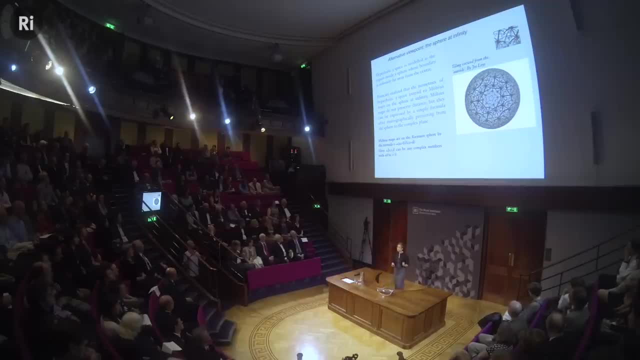 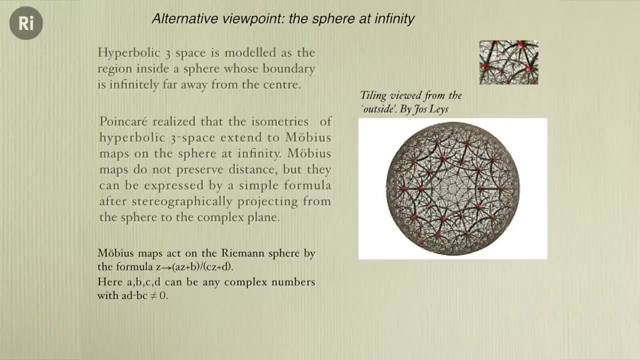 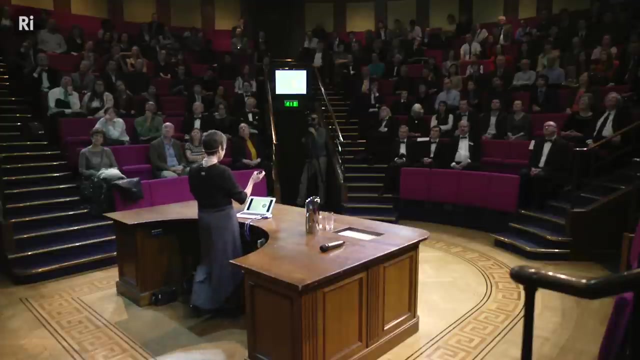 nothing more than that. So you can translate the formulas into some simple formulas with complex numbers and we can write down the effects of an isometry of three-dimensional hyperbolic space inside the ball. we can write down the effects out on the boundary. 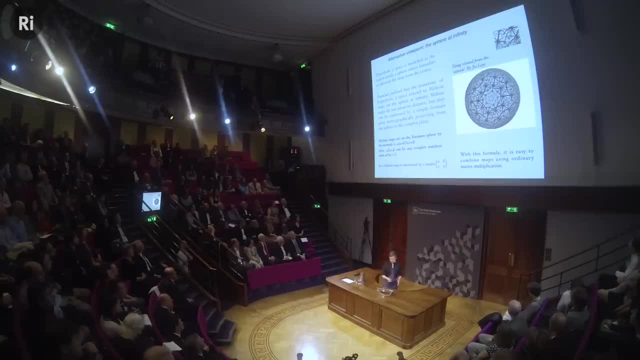 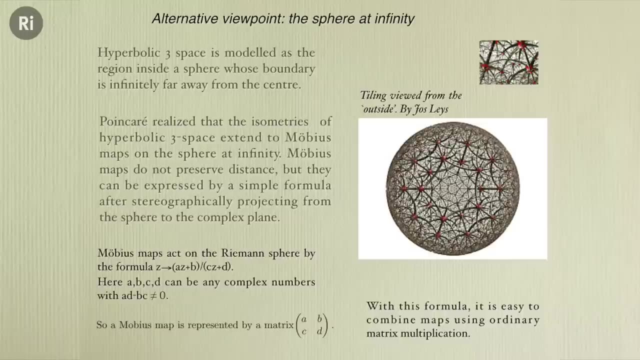 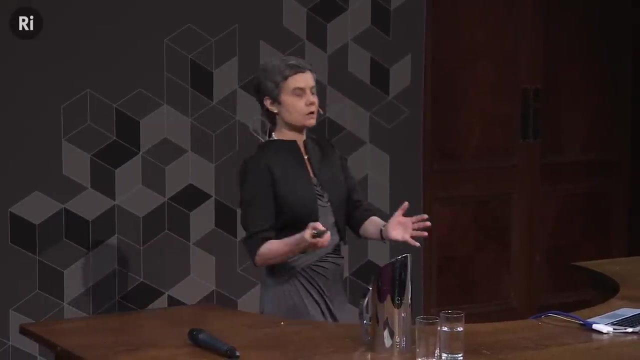 and this formula. the beauty of this formula is it's just a two by two matrix or a nice formula like that, and we can just multiply two by two matrices and do all our calculations. So instead of having to have quite complicated 3D stuff. 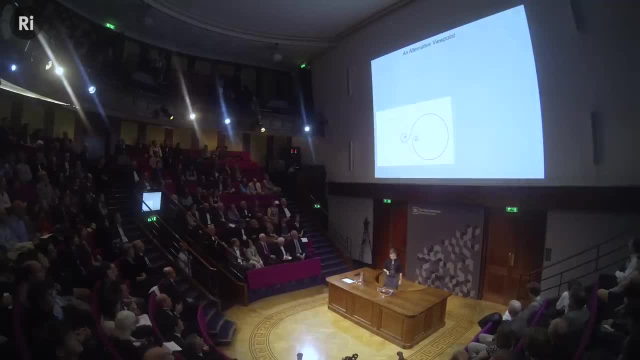 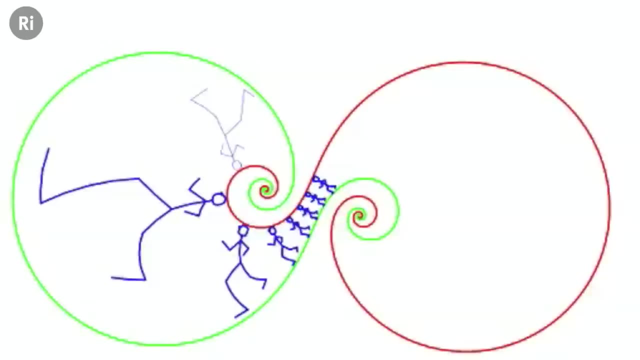 we can work in 2D And yeah, there we go. Now we can see. what I'm doing now is I'm showing you the effects of a particular isometry of three-dimensional hyperbolic space, but I'm just looking out at infinity. 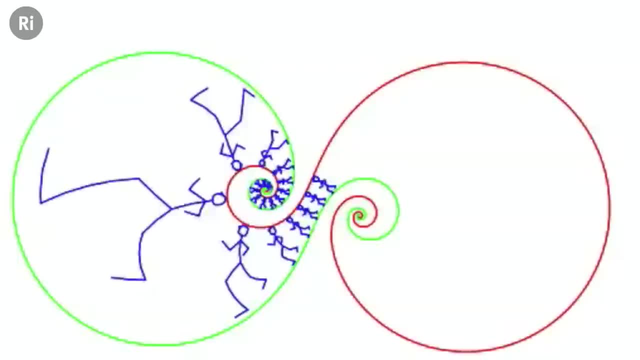 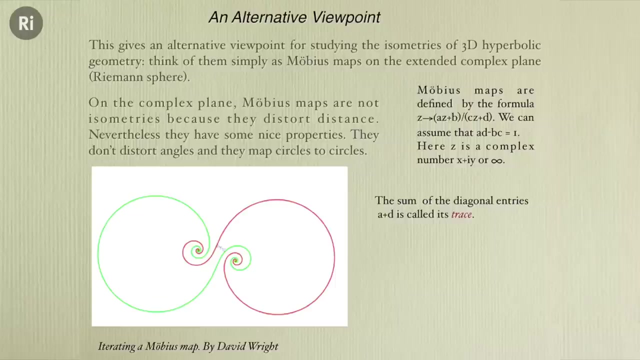 and watching what it does out at infinity. So this man is getting transported around and that's while we're watching him, waiting for him. Here's the formula. So I just want you to remember this for later on. I'm sure everybody will remember this. 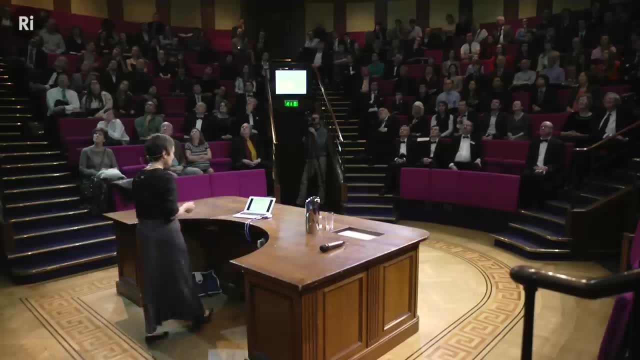 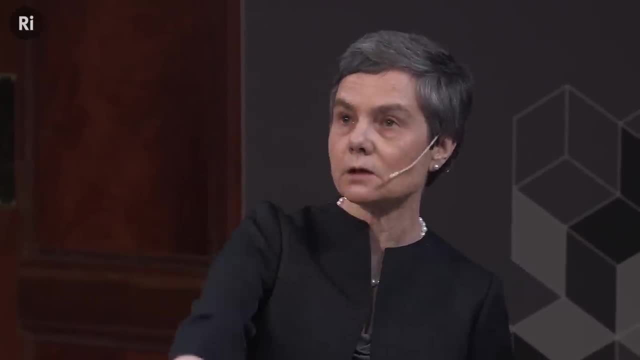 A plus D is an important quantity. and why is it important? Well, you can see that this person is going around in spirals and he goes forward into a kind of sink and he goes backwards into a sink. So there's a forward sink and a backward sink. 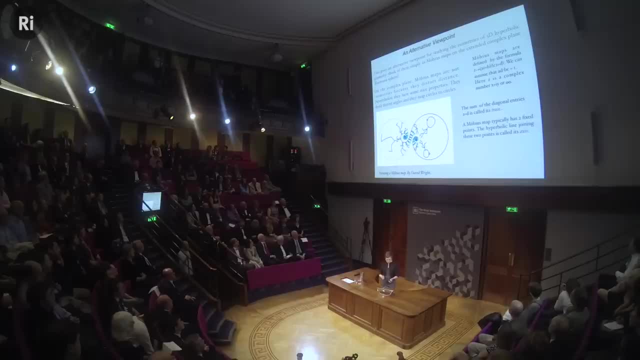 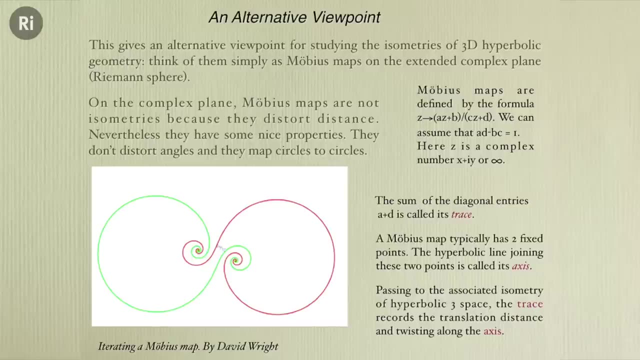 and in 3D. what's this isometry doing? There is a hyperbolic geodesic going from a line, going from one end to the other end, so it's a sort of piece of circle orthogonal to my boundary sphere, and this transformation is pushing along. 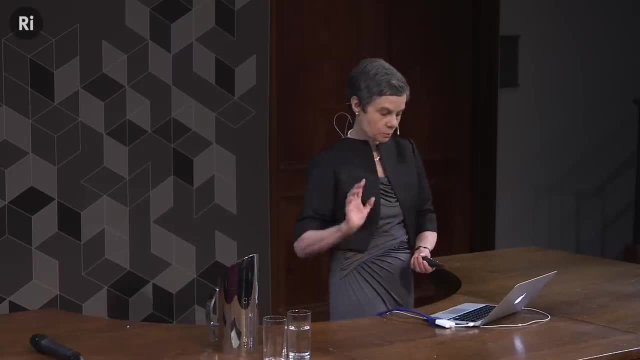 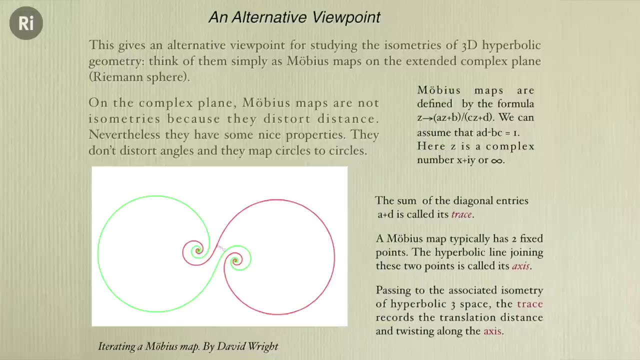 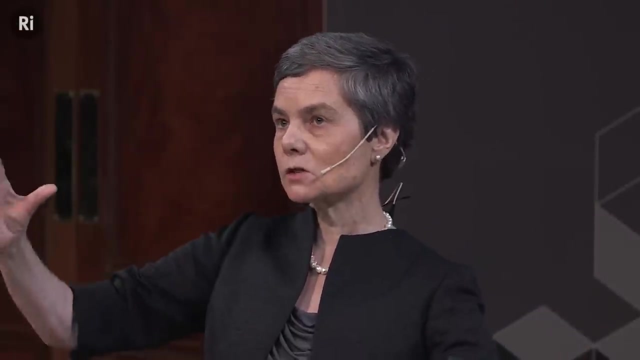 this axis and twisting as it goes. So it pushes along and the twisting is, you see that effect is spiraling. So that's what one of these mappings does. So it's very important when you look out at infinity, all the facts about. 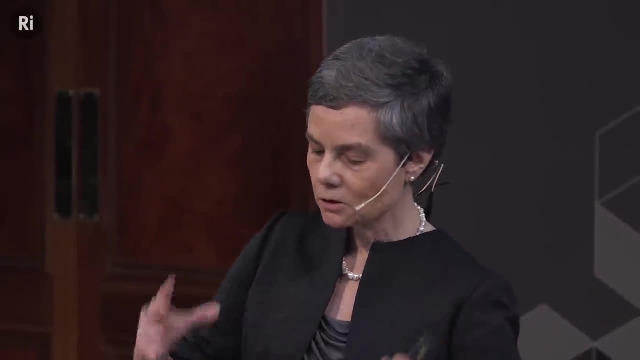 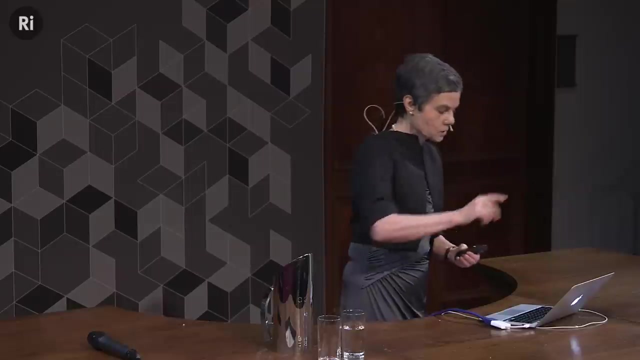 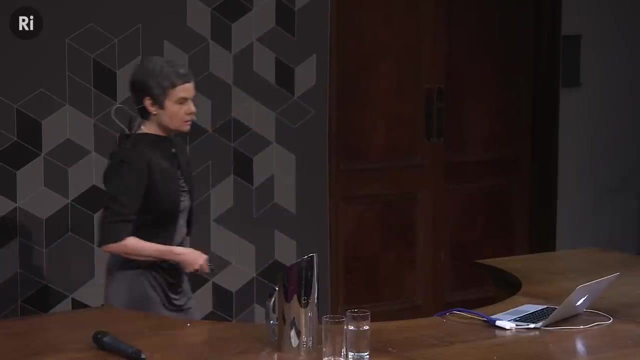 being rigid motions go away, but still a lot of good stuff remains. and just think about this kind of motion along an axis that you translate and you rotate and that can be read off from this A plus D number called the trace. Okay so, 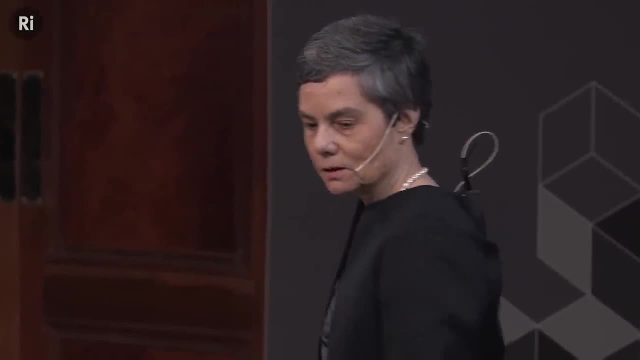 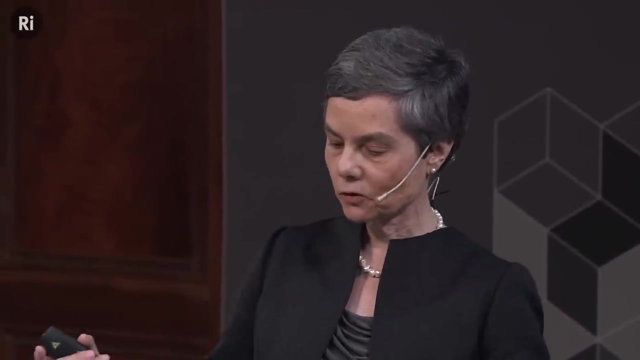 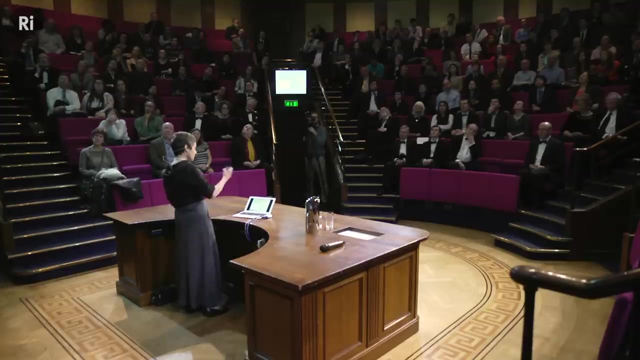 now I need to introduce another idea. That was one isometry. Supposing I had two or several isometries and supposing I do a bit of one and a bit of another, and a bit of another and a bit of another. I keep going with them and I allow them to go backwards. 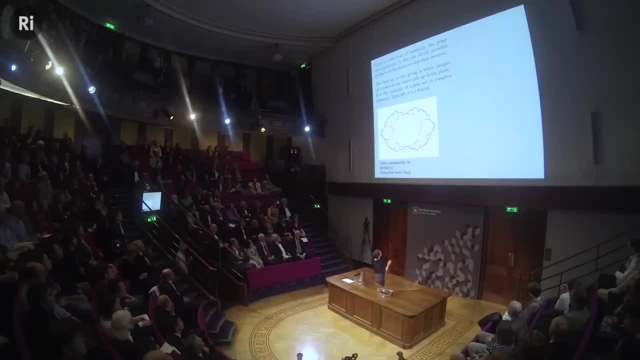 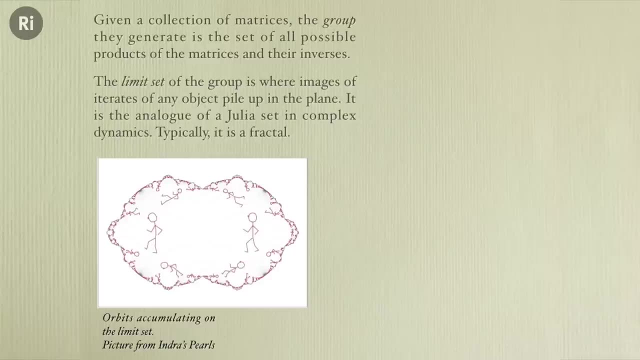 as well, and I pick up a picture of this poor man and I transport him around. This particular one has just got- he's got one thing that's pushing him one way and another thing pushing him another way and he gets twiddled around. 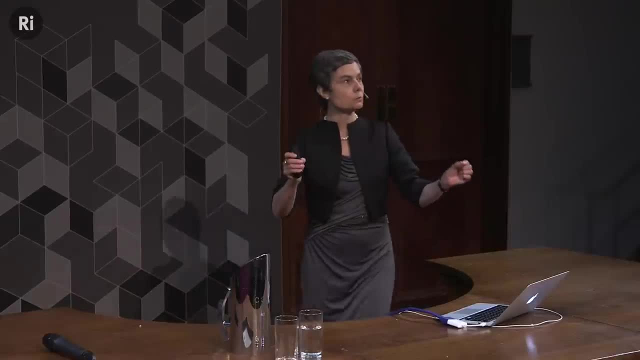 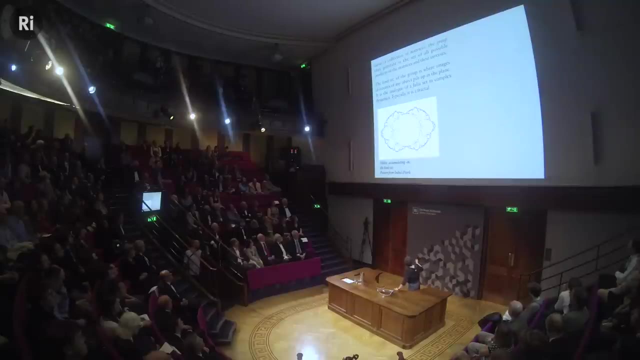 and what happens? instead of there being just two fixed points, a source and a sink, there are actually a whole continuum of sources and sinks, well, a whole countable number of sources and sinks. and he gets. you can see his images get smaller and smaller. 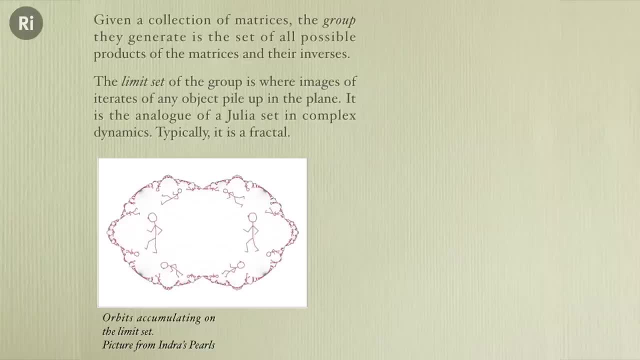 and smaller, but they go all the way around the edge of this thing, and this thing is called the limit set of this collection of matrices, And you can also think of it as the chaotic set. When you get to that level, everything is moving around chaotically. 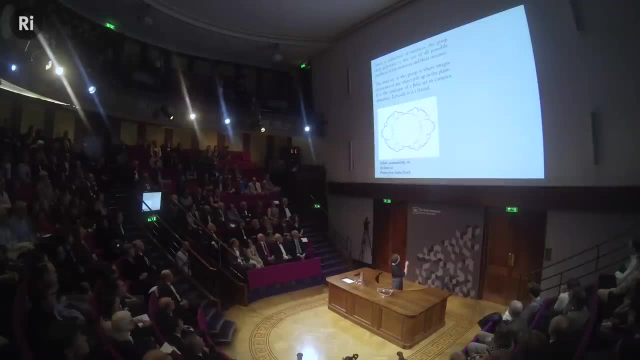 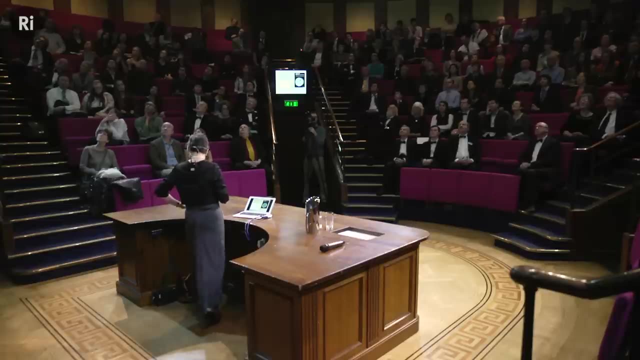 In fact you don't quite see it in this picture, but this boundary here is a very complicated and rather beautiful fractal curve. Now I'm not really going to go into this too much this evening, but we explore. I wrote a book. 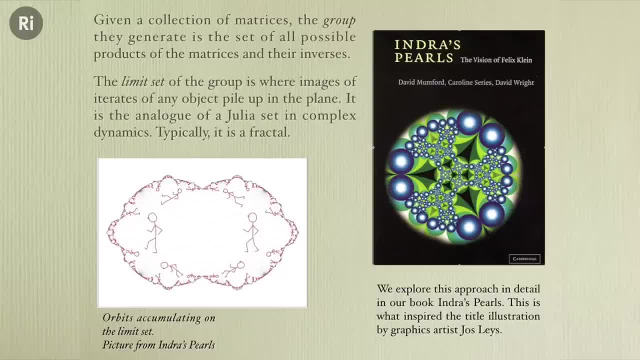 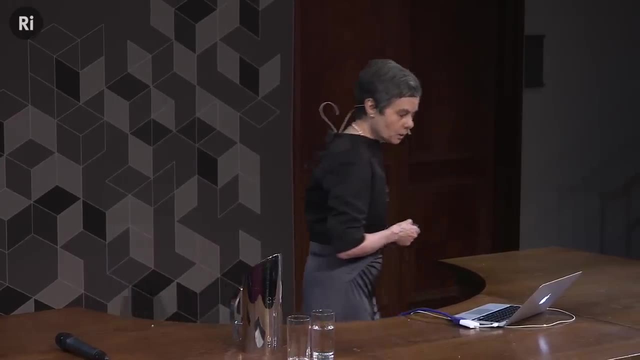 some years ago with these other people, and David Mumford is a very brilliant mathematician. David Wright was originally a student at Harvard. he's also a number theorist, but he's extremely good at computing. We wrote a book explaining how you make. 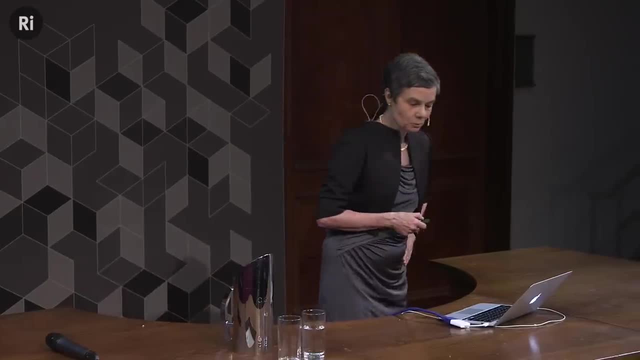 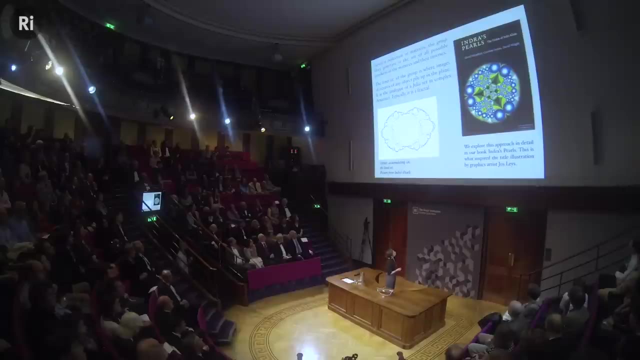 pictures like this and, in particular, a number of people have taken that up. in particular, Josh Lais used some of our recipes and that's how he created some of his pictures. So let me now start. I can now start telling you some. 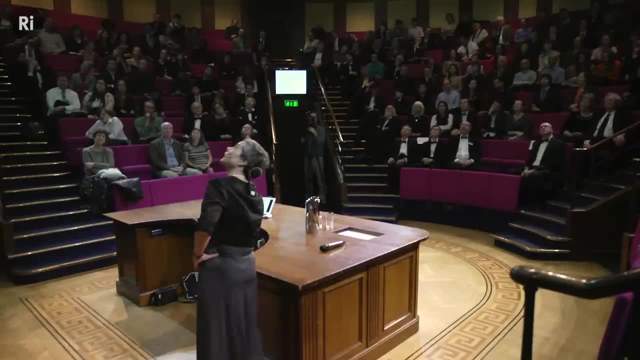 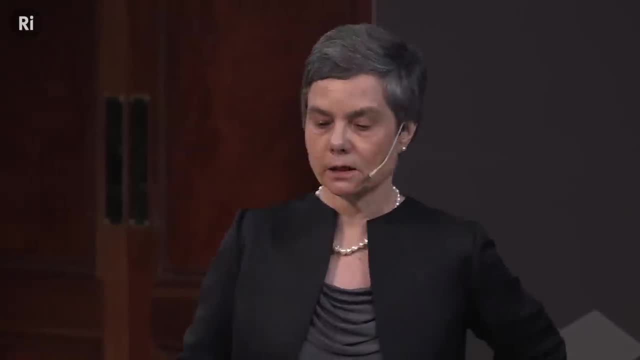 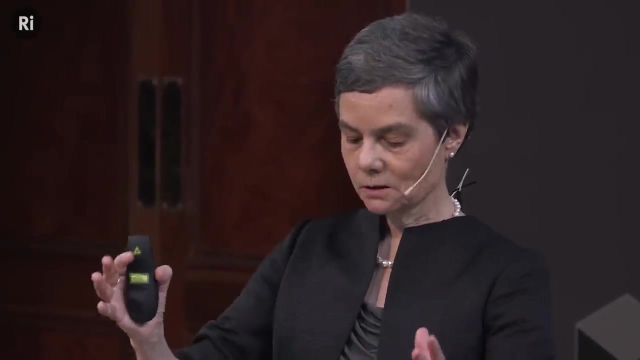 more recent mathematics, And the first thing I'm going to tell you is about hyperbolic manifolds whose volume is finite. Right well, I take a finite sort of original tile or cell, finite size, and I glue up the side, so what I get is a finite size. 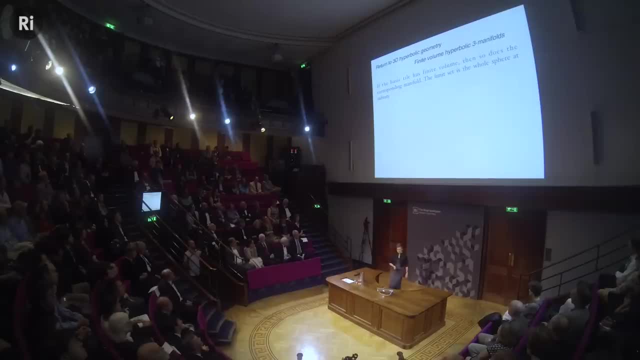 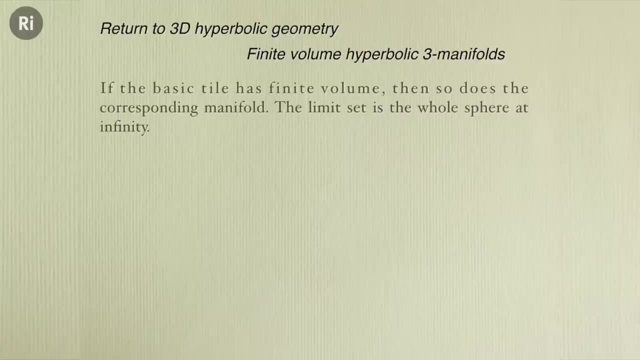 So that's what we're talking about, and we assume that this thing is glued up, so there's no boundary anywhere. and now there's something about 2D. I didn't tell you if I make, for example, a torus by gluing up a rectangle. 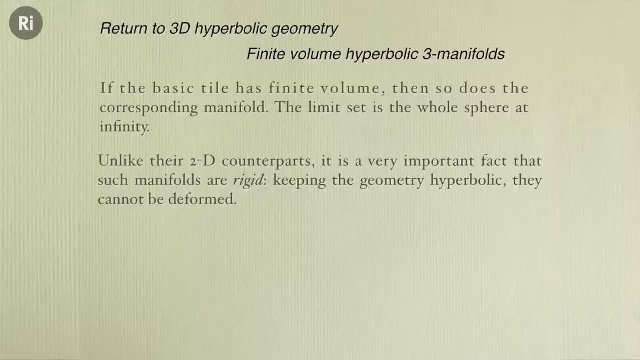 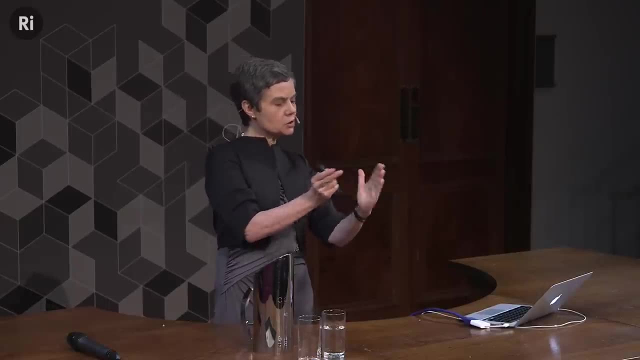 I can make it a long thin rectangle or a short fat rectangle and I can actually skew it into a parallelogram and still glue up the sides. so I can do a lot of things and it'll still be Euclidean, but the tiling of the plane will change. 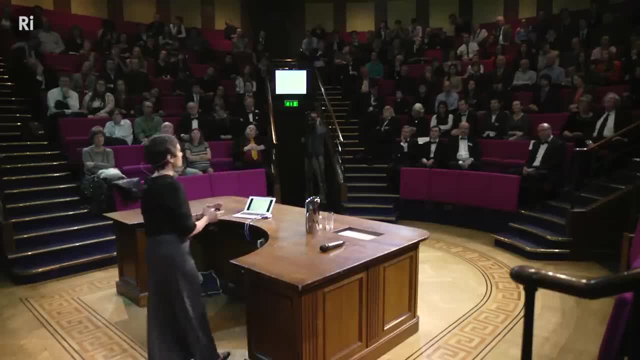 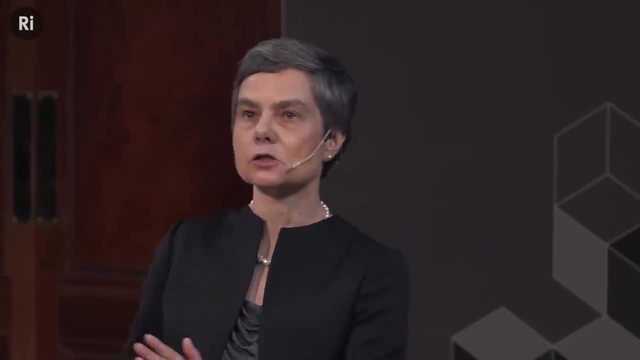 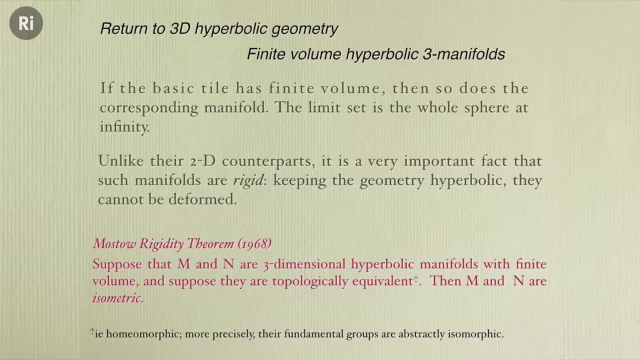 And it turns out in 2D. you can always do that. there's a whole science called Teichmuller theory about how you can deform geometric structures on surfaces In 3D. a theorem, a famous theorem called the Mostar Rigidity. 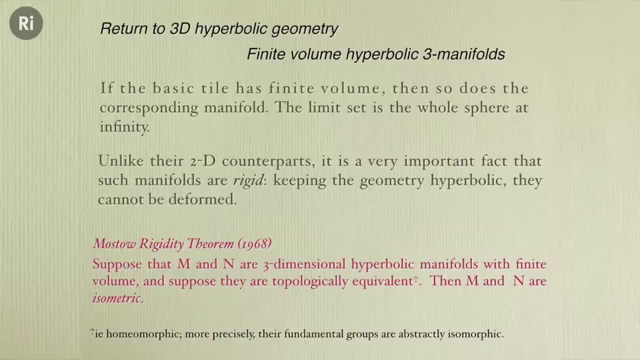 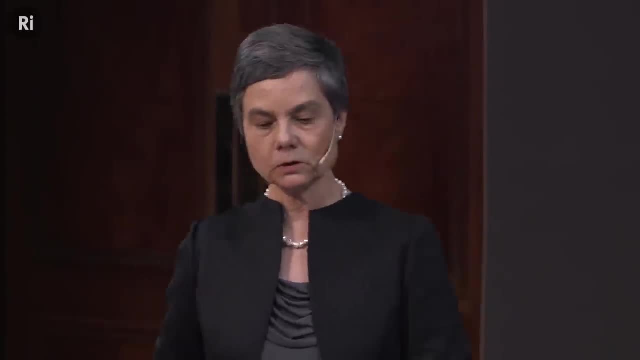 Theorem says: in 3D you can't do that. things are fixed, they're rigid. So what does this thing say? Supposing I've got two of these finite volume manifolds, and supposing well for the mathematicians, supposing they're. 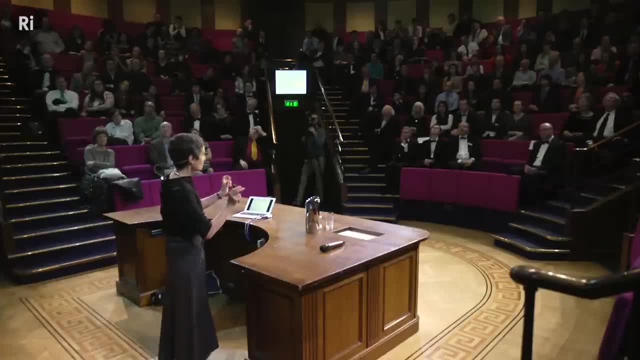 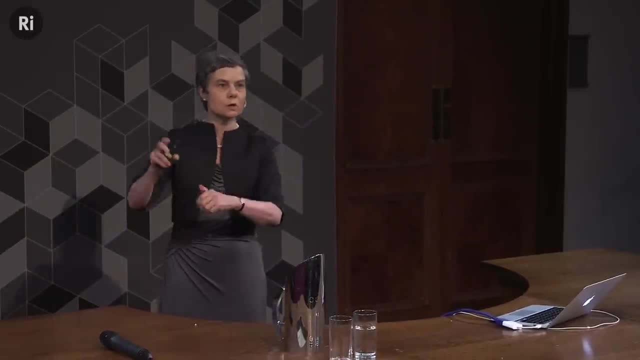 fundamental groups. they're abstractly isomorphic, but imagine not all of you are mathematicians, so supposing they're topologically the same, somehow you know that you can squish one and do all kinds of mess to it. forget the geometry altogether. 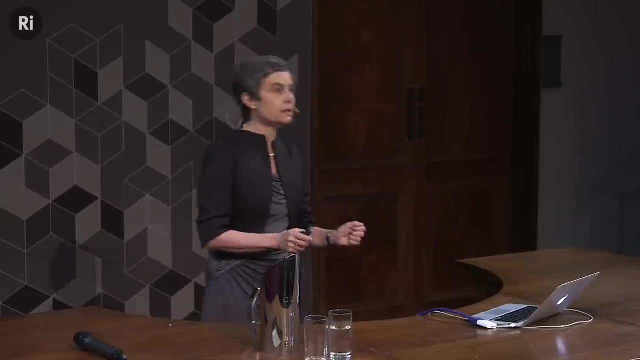 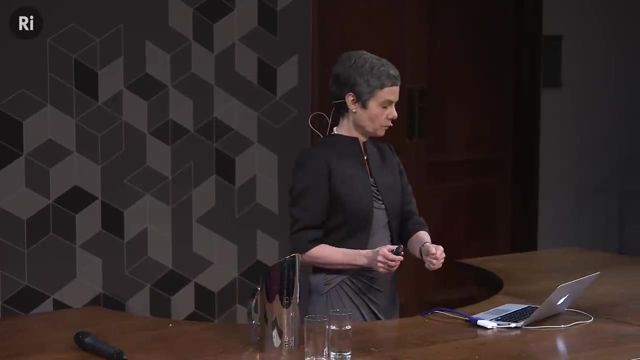 and you can get to the other one. actually, then they're really the same thing. they're isometric, so rigidly, you pick one up and it's exactly the same as the other one. So that's what Mostar's theorem says. 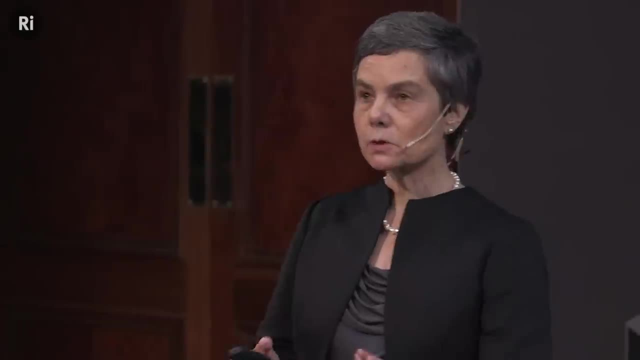 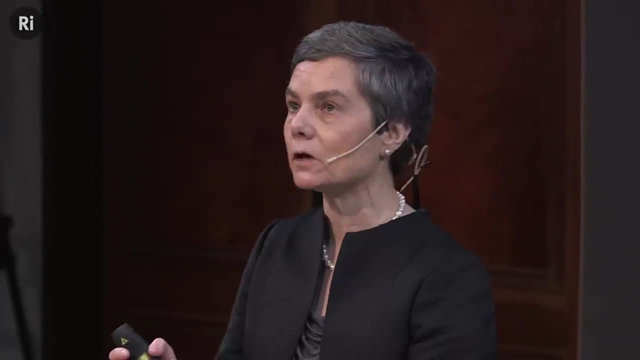 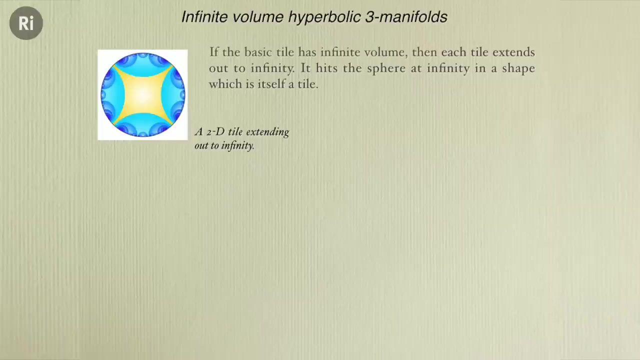 And now I'm going to talk about something else. So that was a tile which was finite volume. I've been more concerned with tiles which have got infinite volume. So here's a picture in 2D. so this particular yellow tile, you can see it goes all the way out to infinity. 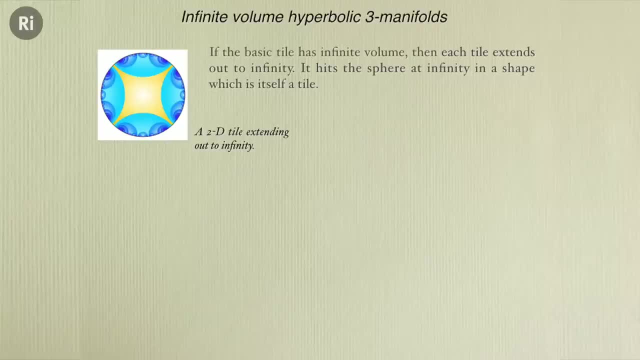 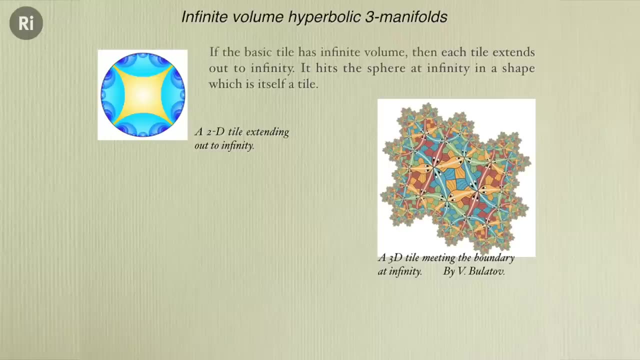 and there's a kind of thickish piece that goes out and that means it's got infinite size. and here's another picture. now this picture is a what you see at infinity from a 3D tile. so imagine I've got my hyperbolic. 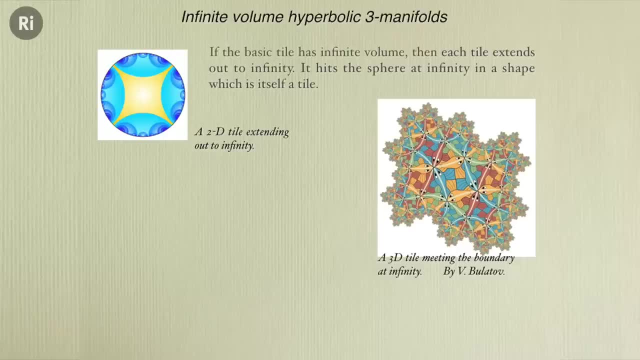 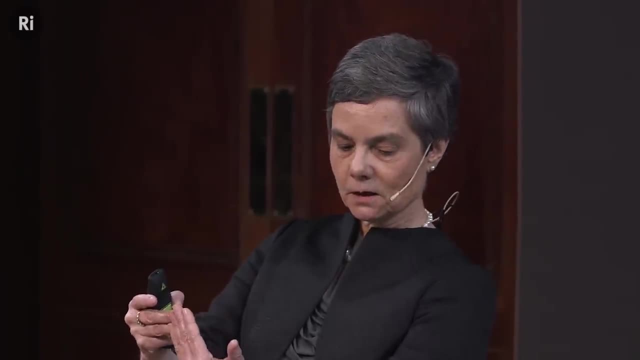 space inside the ball and I'm kind of looking through from the outside in and there's some complicated basic tile and it hits the boundary at infinity, and then you can take all the copies of it and so I tile the stuff at infinity. 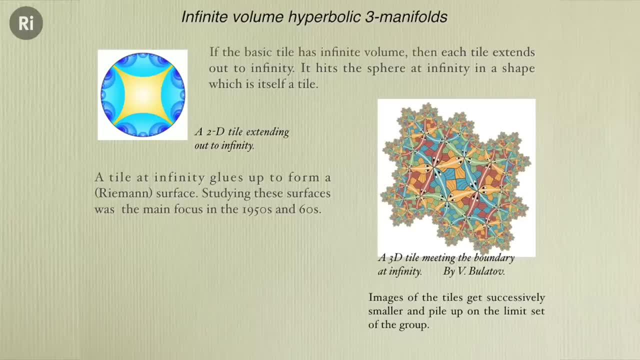 So that's what you're seeing in that picture, and you can see how the tiles get smaller and smaller. and, of course, what do they do? They pile up on this same thing, the limit set of the group. and if you would take this, 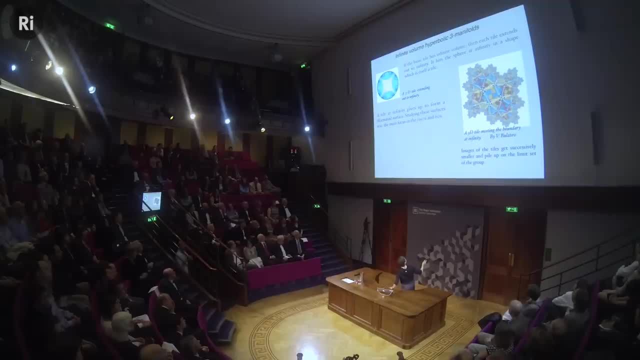 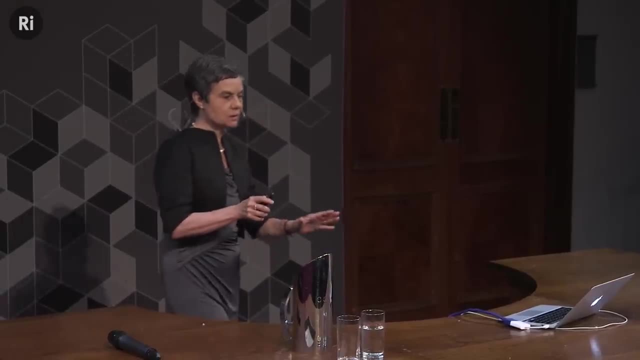 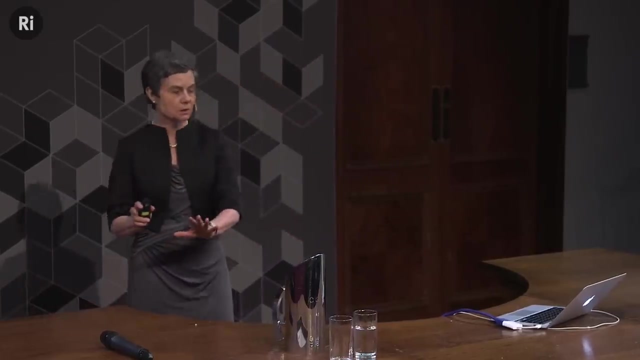 stuff out at infinity. you could play the game of gluing up the sides of the tile, but now we're distorting things by these Merbius maps that have forgotten how to measure distance, but they do know how to measure angles, So you can think. 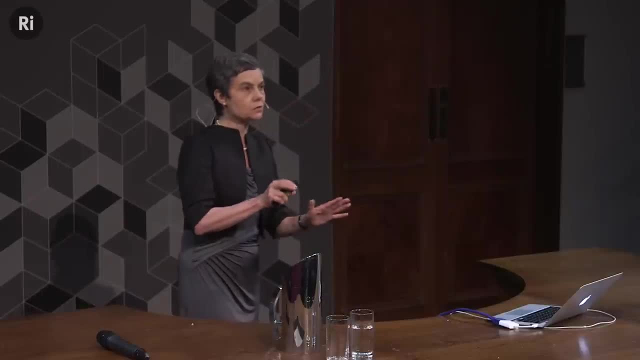 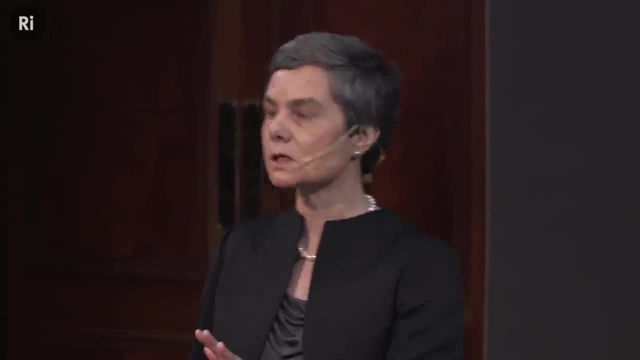 that, whatever it is, I mean by Riemann surface. it's a kind of structure that's like geometry that only remembers angles, and there was a great deal of work in the 50s and 60s studying these things, and here's. 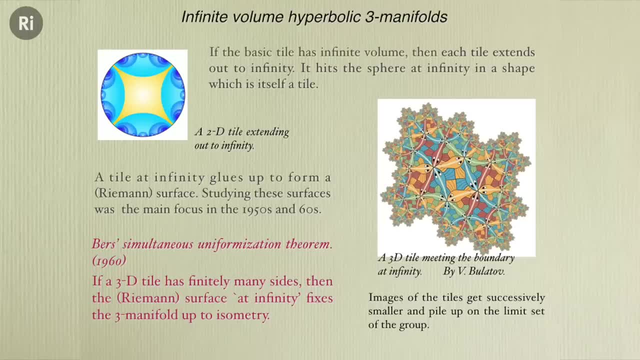 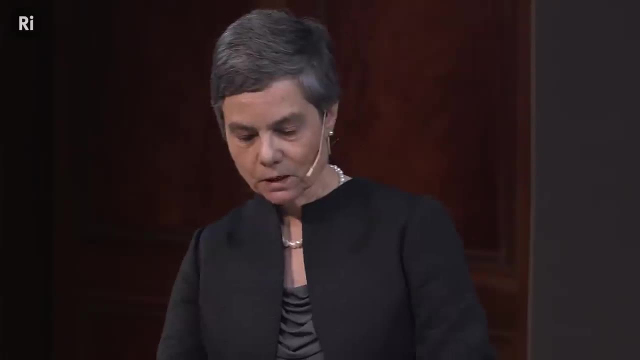 another famous theorem. It's a bit like an analogue of the Mostow theorem. It says that if I stick up these things, then if I control what happens out at. so there's a tile and in the middle of hyperbolic space. 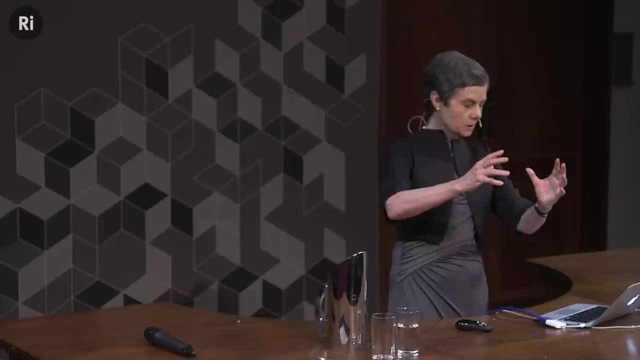 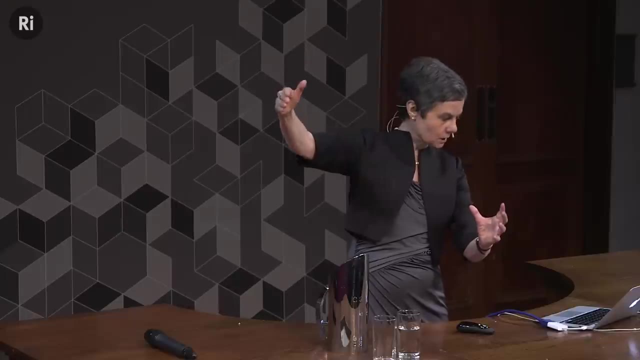 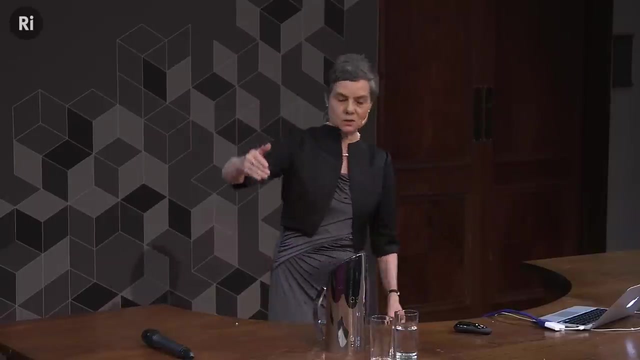 that well, we glue up the sides of the tile and we produce a solid thing that has some bit that goes off out to infinity And out at infinity. we have this floppy tile that's glued up, which only remembers angles, And what Bayer's theorem says is: 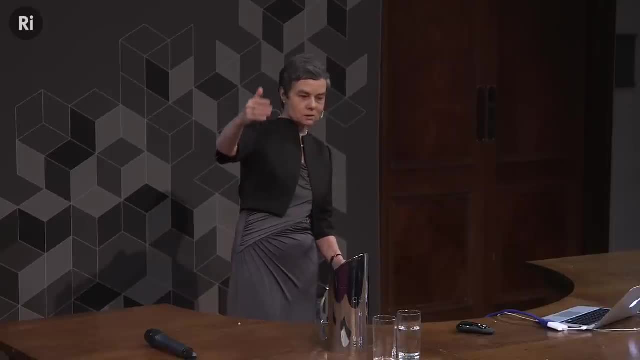 if I know what happens to the angles that stuff out at infinity- and I know that for every part of the tile that went out to infinity, then I know everything. Then it's fixed. So it's sort of like an analogue of Mostow's theorem. 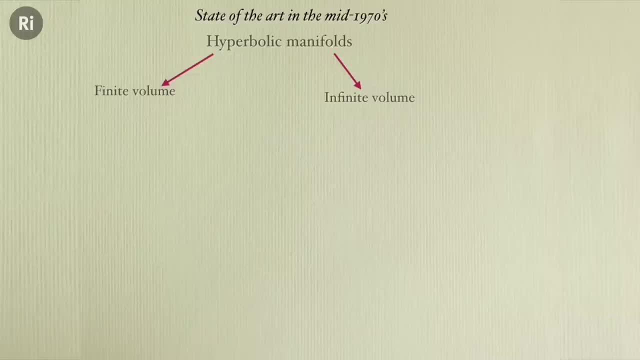 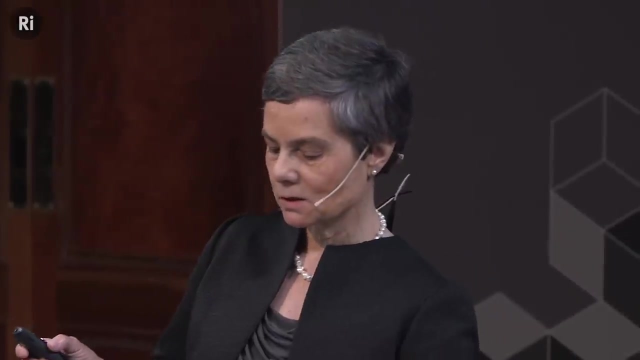 So hyperbolic manifolds, we can think of finite volume, we can think of ones with tiles going out to infinity, and then there's a rather subtle distinction that probably kind of lost at the moment. but anyway, you can have finitely many sides. 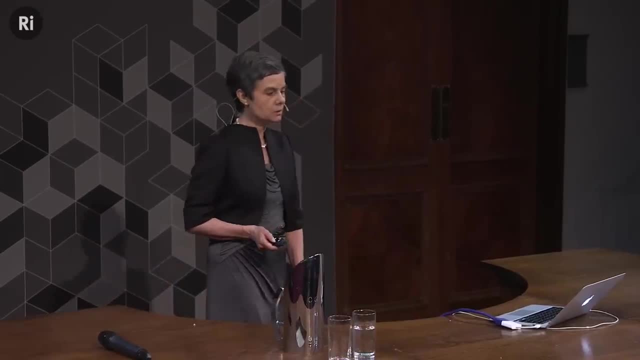 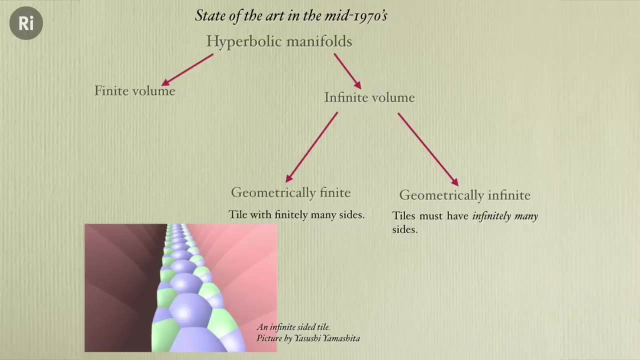 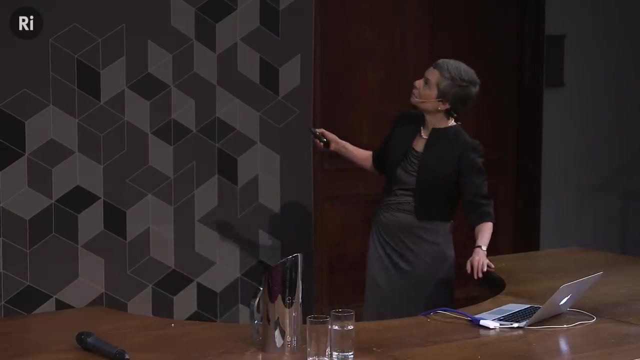 or infinitely many sides of the tile. So what should we know? Well, there's a tile with an infinite number of sides and we're sitting inside a tile. It actually only takes two transformations. You wouldn't quite believe it, but because of spiralling that you don't really. 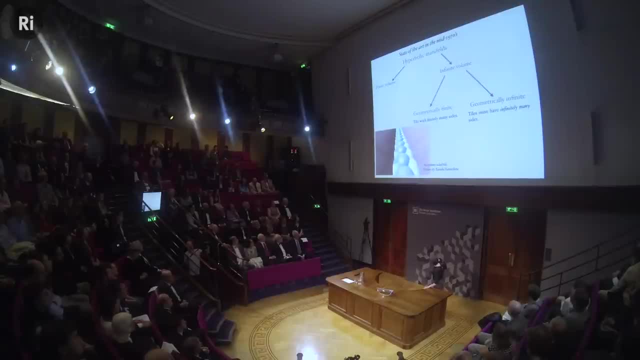 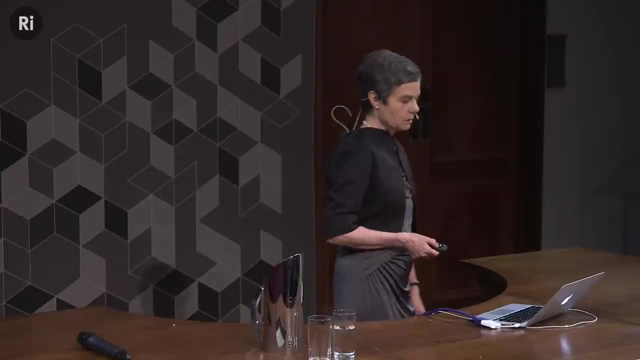 see, it actually only takes two isometries to glue up all of this stuff and make some complicated manifolds. So what was known? Well, we knew this wonderful Mostow rigidity theory, but we didn't really have many examples. 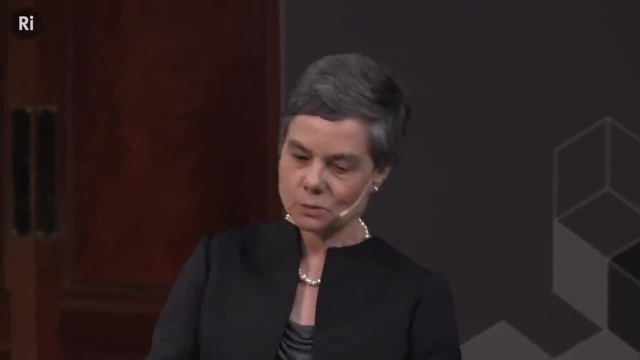 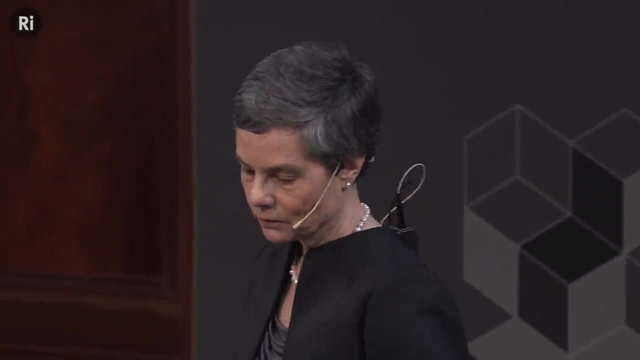 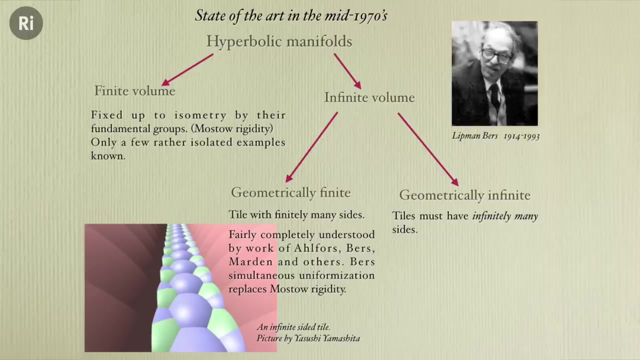 There were some. There were some nice examples, but they were sort of a bit special and almost like curiosities. Maybe some examples to do with number theory. Then we had the theory of Baer's theorem and there's a picture of 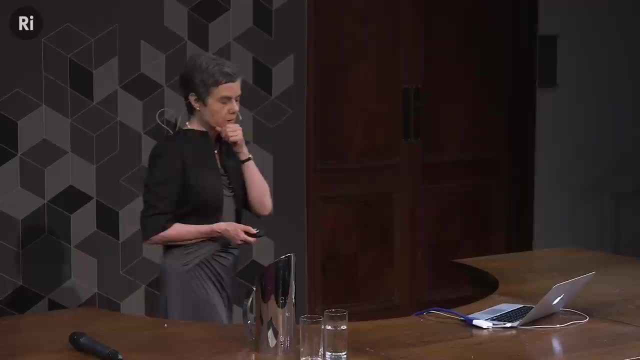 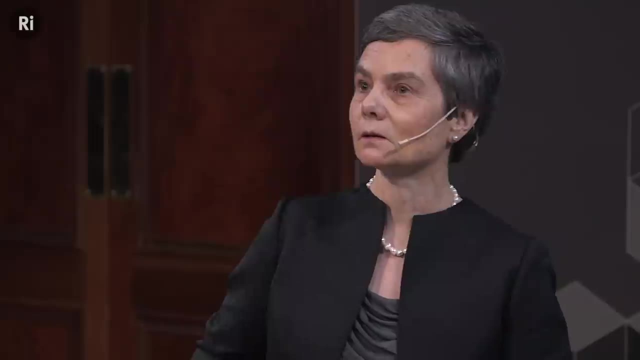 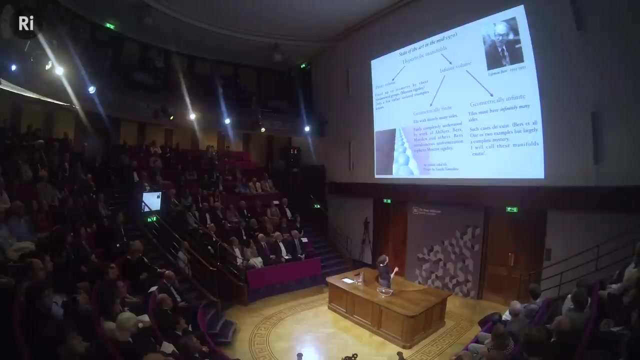 Baer's, who was? I think he was originally Finnish, but he spent the latter part of his life in the United States. Originally he worked on fluids, but he got drawn into this subject. So well, okay, There was this. that was pretty much not. 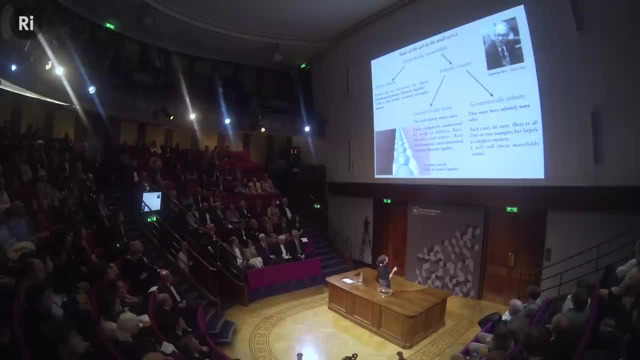 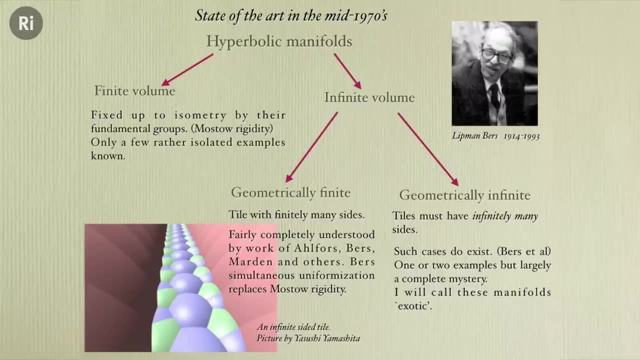 many examples, but we understood something, Something was understood here. These were a complete mystery, except Baer's and the work of a few other people, said there must be some funny things which don't fall into this category. So there are some that we don't really. 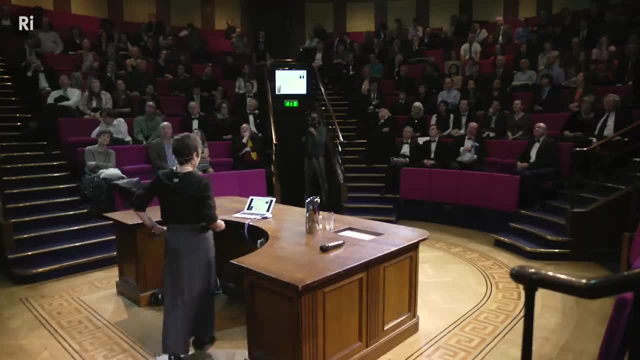 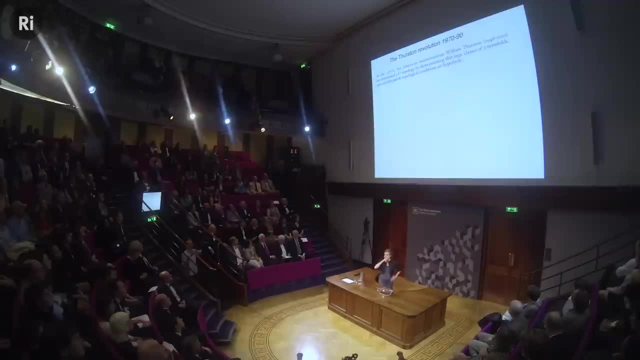 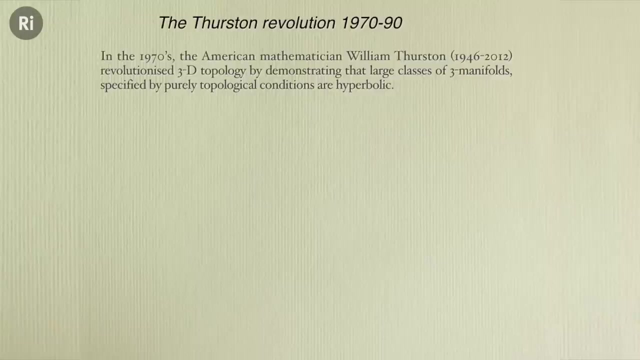 know anything about at all. So that's where we were at, And then William Thurston came along. So in the sort of late 70s and early 80s Thurston started. he came into this subject and he started proving just incredible theorems. 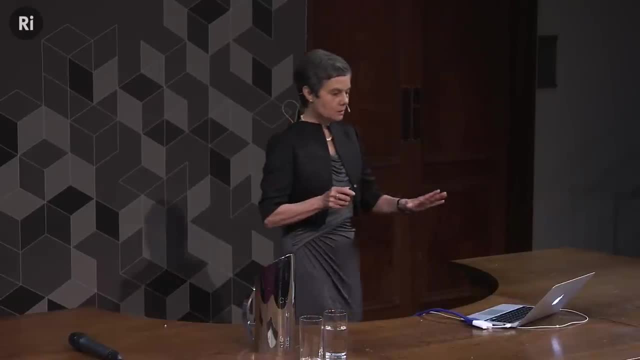 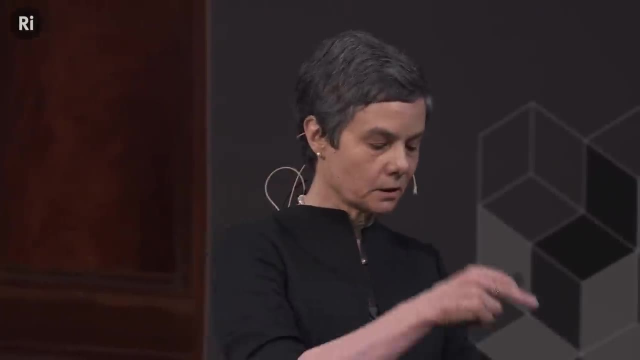 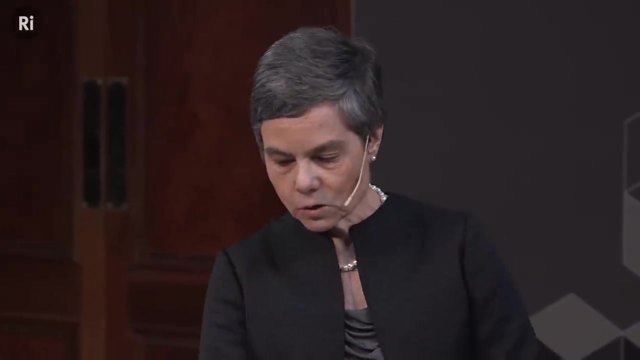 Remember, in 2D we knew that every surface had a certain kind of geometry attached to it, Either Euclidean, hyperbolic or spherical. So the first thing that Thurston began doing was he started taking lots of three-dimensional manifolds. 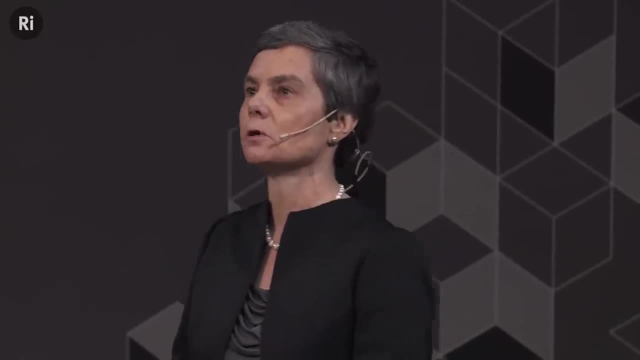 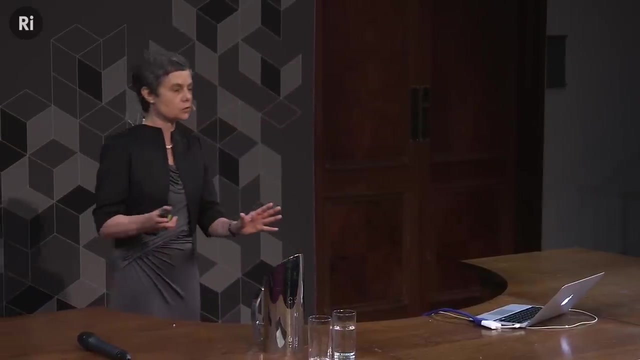 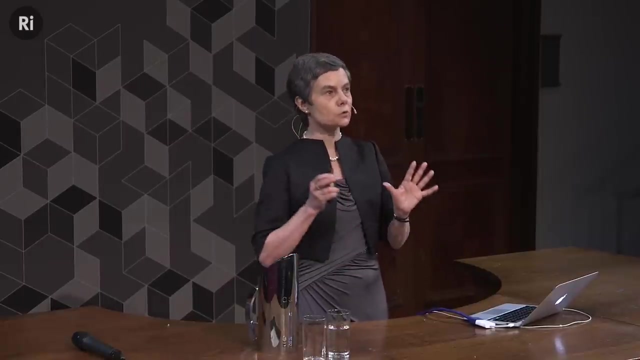 that the topologists kind of understood, but only in terms of topology. They didn't know anything about. they didn't have anything to do with geometry. He just took these sort of abstract constructs of topological objects and he showed that actually you could impose or 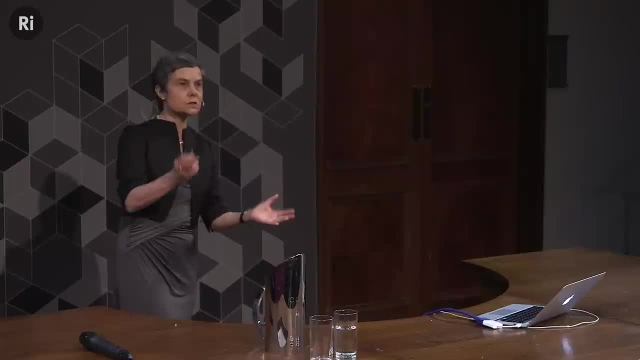 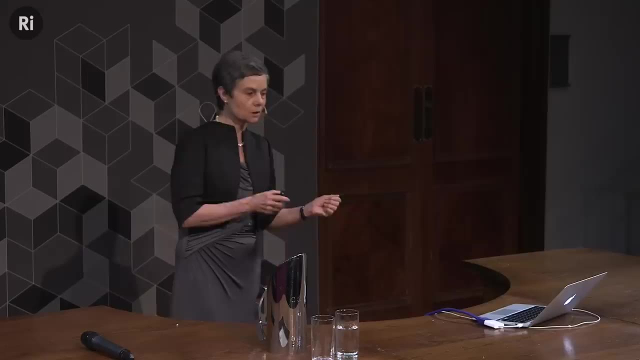 in a natural way a hyperbolic structure. You could make this basic crystal that you could glue up and you could make it hyperbolic. So I don't have time to tell you what is very technical, what classes of manifolds. 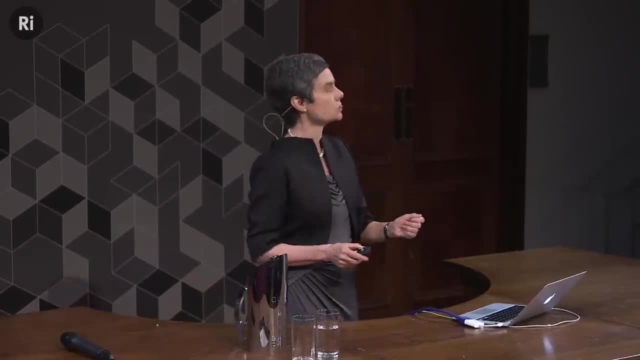 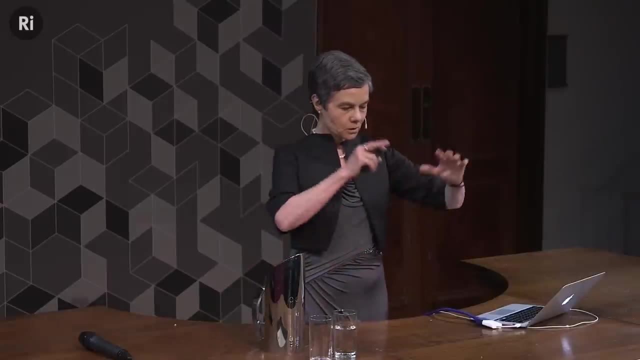 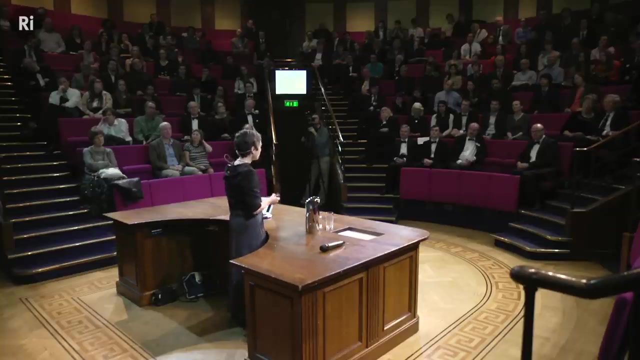 but really very large classes And this was completely astonishing. Nobody had imagined anything like this before. One of the classes was: if you take 3D space and you draw some complicated knotted loop and then you drill that out of space and throw it away. 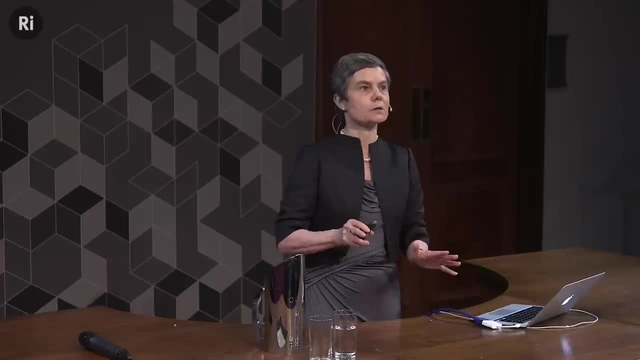 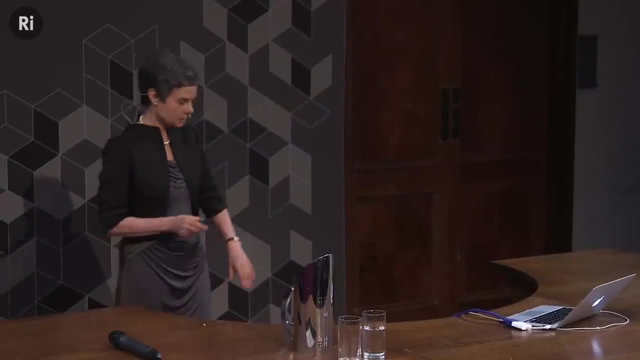 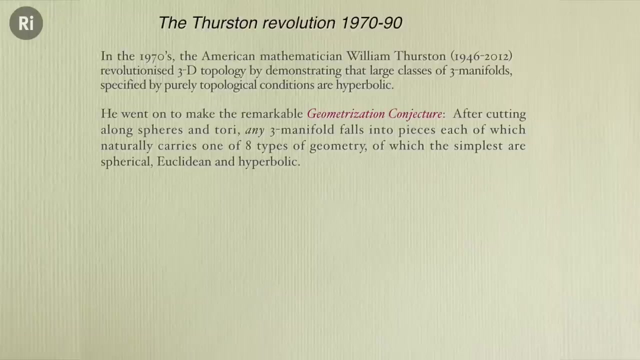 and take everything that's left, that's a manifold, And he showed that most of those are actually hyperbolic manifolds in a very precisely defined sense. So he then went even further and he made something known as the geometrization conjecture. 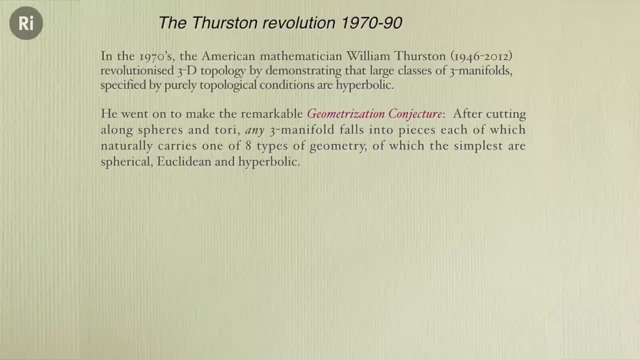 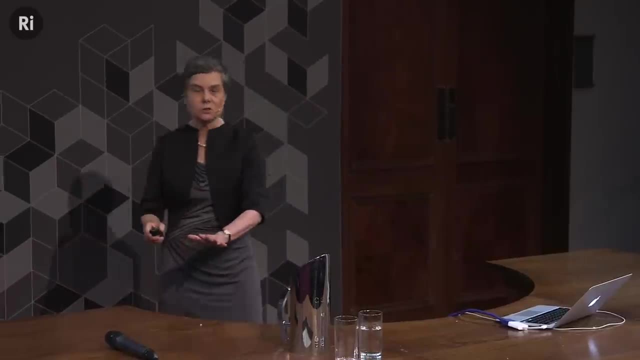 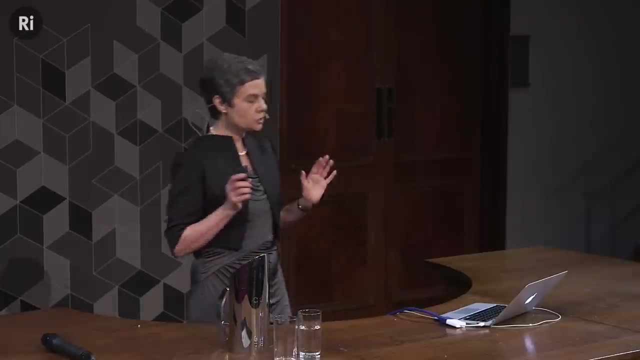 that you might ask. is it possible, then, that there's a way of putting geometry on every three-dimensional manifold And to do it in 2D? well, you know, nobody before him conceived anything like this, but he conjectured that in view of all the things he'd already. 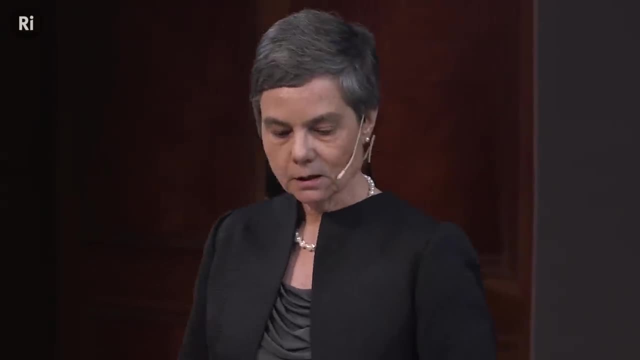 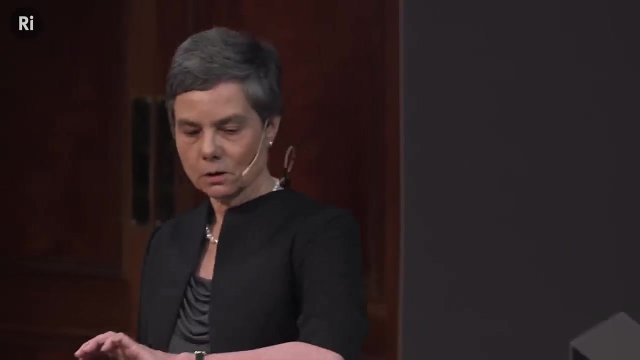 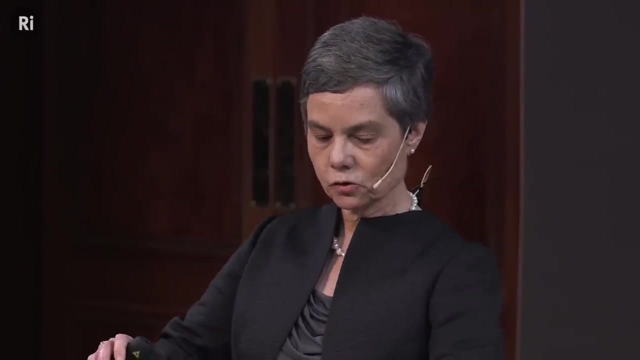 done and he'd shown were hyperbolic, that actually not that there was a particular geometry on every manifold, but that after you. so just as if I take a curve on a surface and cut it, it opens out. if I, for example, draw a, 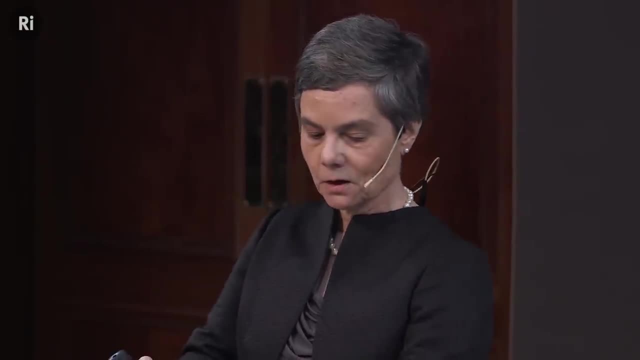 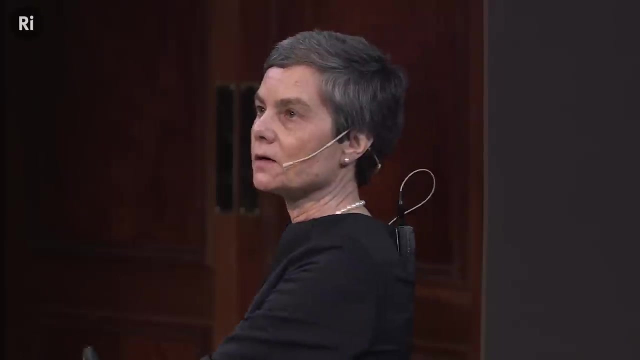 torus inside a manifold and cut along that, I'll get two bits of manifold, the bit that's on one side and the bit on the other, and maybe the bit on one side and the bit on the other side separately have some geometry. So that's. 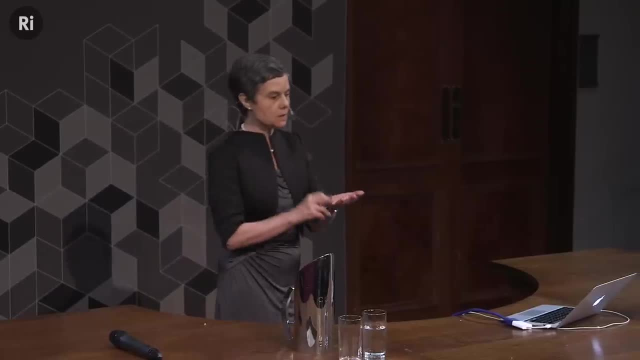 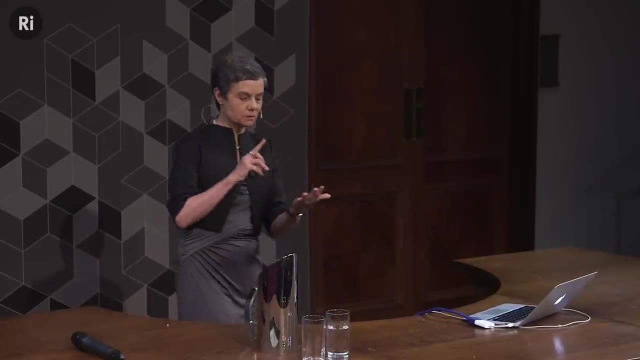 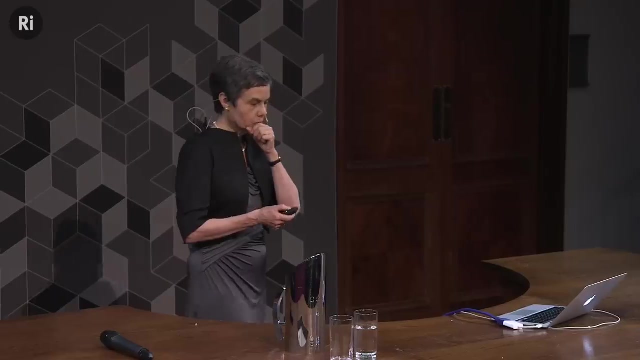 what he showed. And he also showed there are only eight types of geometry and they're all quite simple, and in particular we've got spherical, Euclidean and hyperbolic. and actually so he conjectured this was true. he didn't prove it, To just 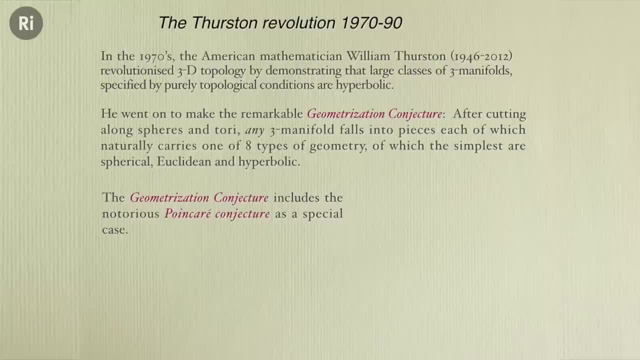 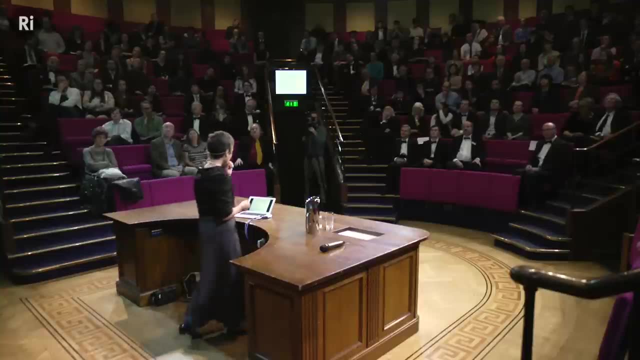 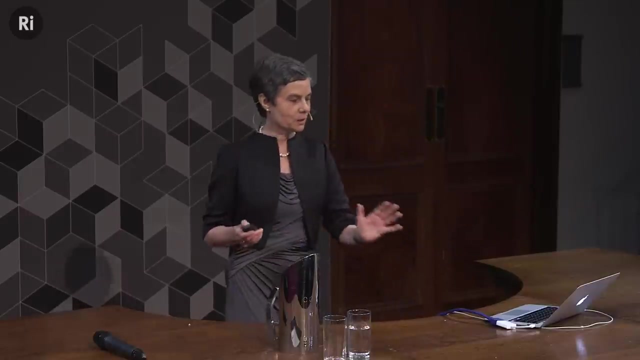 give you a sense of how sort of what an immense conjecture this was. I'm sure many people have heard about the Poincaré conjecture, which I will come onto. Let me not say what the Poincaré conjecture is right now. people may have heard. 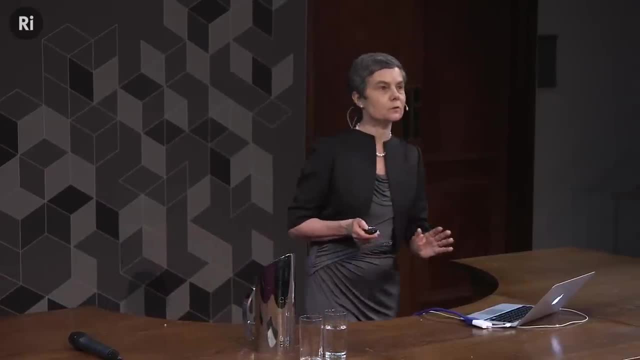 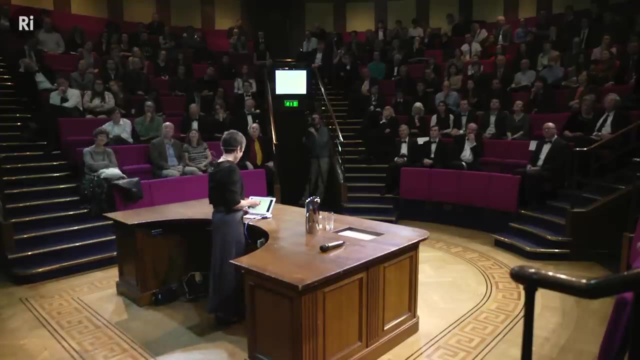 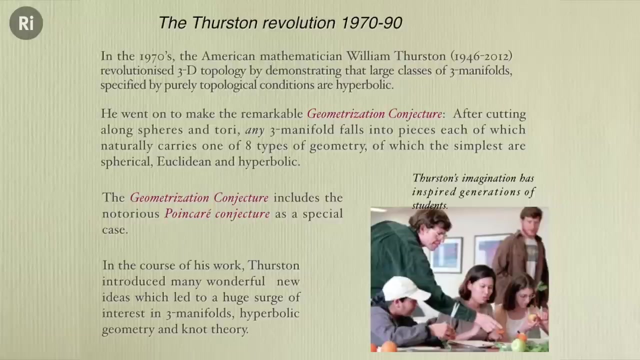 of it, but the Poincaré conjecture was a problem that, throughout the 20th century, was basically driving mathematicians nuts, And to me it's not only that he proved these wonderful theorems, but he introduced all sorts of wonderful concepts. 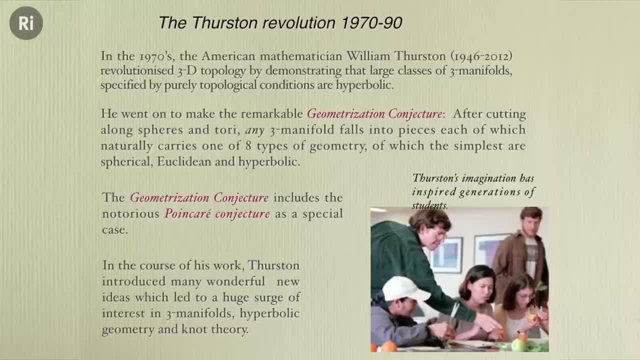 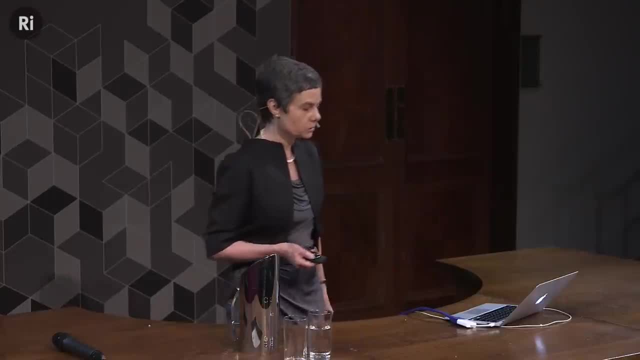 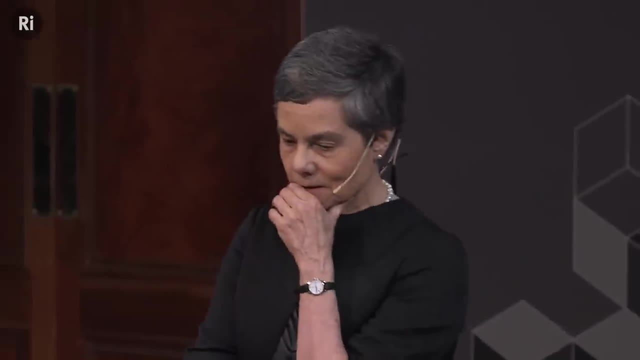 he was a very visual hands on mathematician. Sadly he died quite young- well, not young, but I mean he was not old, you see, a couple of years ago. but he was always tremendously keen on getting students and school children and so on doing things by hand. 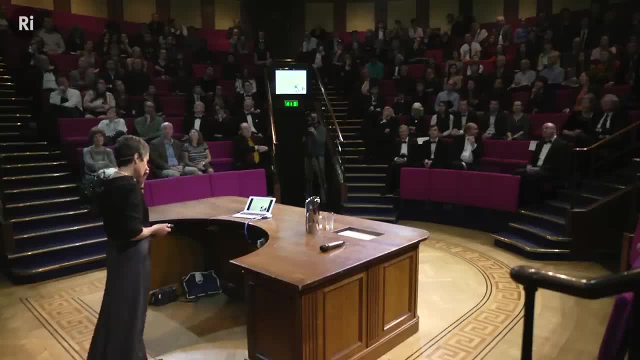 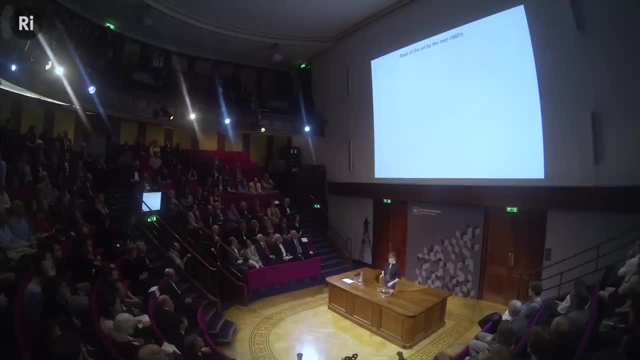 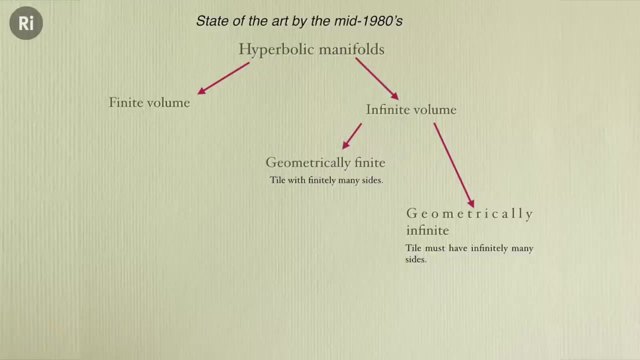 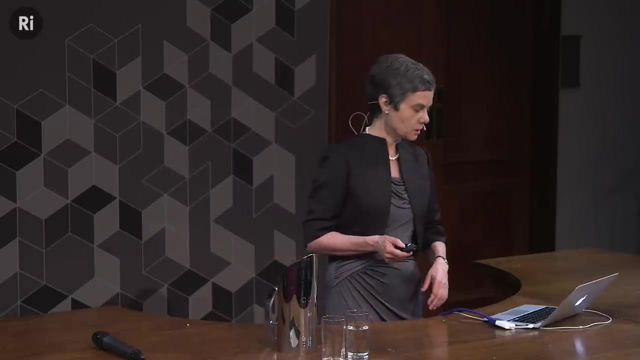 and making shapes and playing with shapes and so on. So he left an enormous legacy of ideas, and he had, so let me show my next slide. So by the time Thurston had been working with a large group of students who were attracted to work with him. 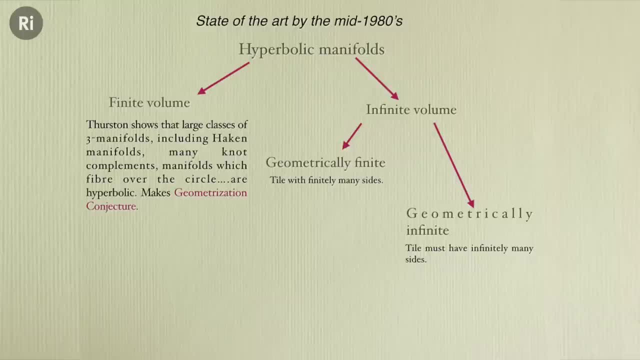 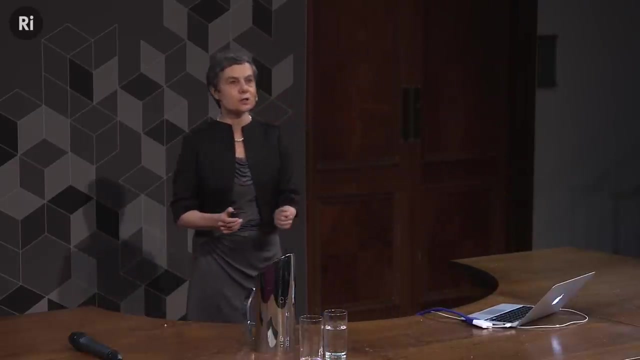 what had happened in finite volumes was that he had enclosed manifolds. well, an enormous amount from being a few isolated examples with a good theorem must have rigidity. it became a huge, big subject, huge, big area. large, large, large classes of manifolds are actually hyperbolic. 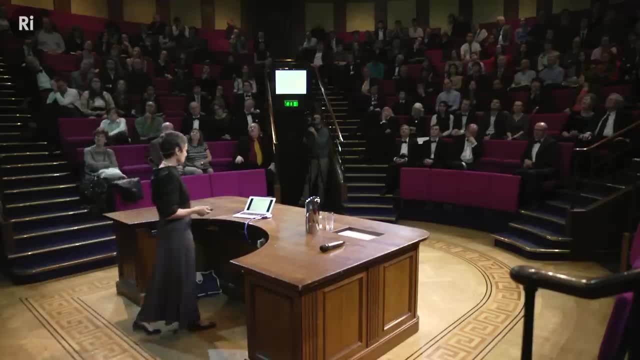 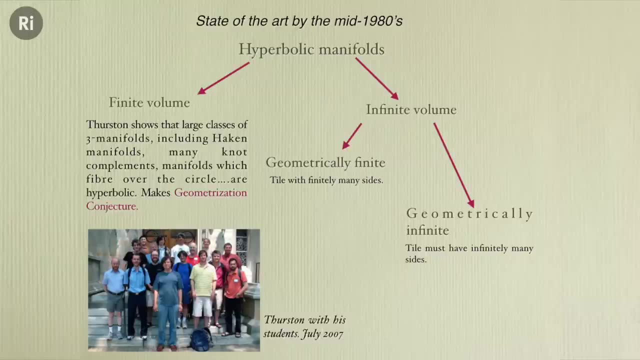 and a great deal of effort went into writing up sort of nice versions of his proofs and so on. Here's a picture of Thurston more recent 60th birthday, and all of these students of his have in themselves made large contributions to mathematics. So this case well. 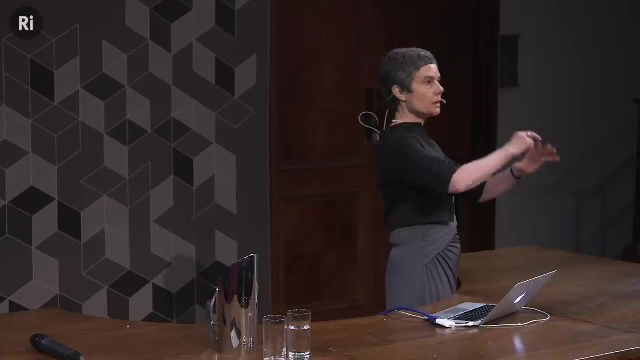 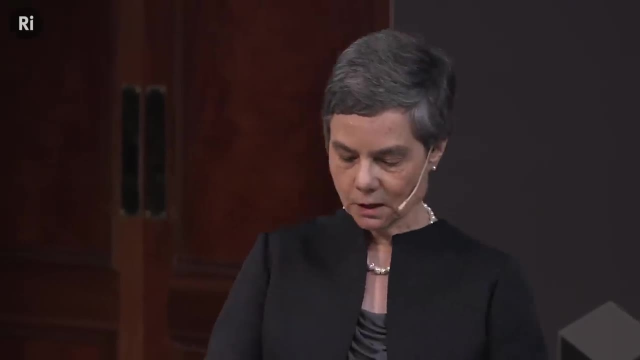 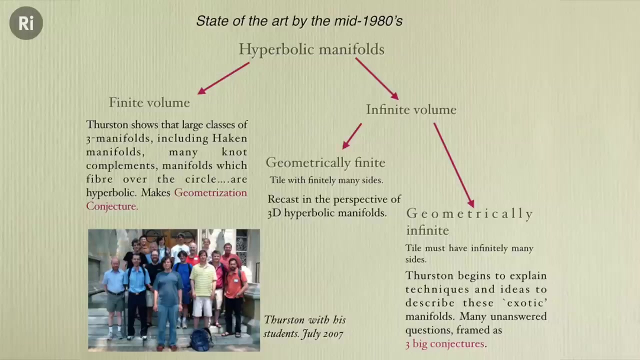 let me just say it was recast from a subject that was mainly about Merbius maps out at infinity into something to do with topology and geometry in 3D and this rather mysterious thing that must exist. well, Thurston did not solve the problem, but he began to. 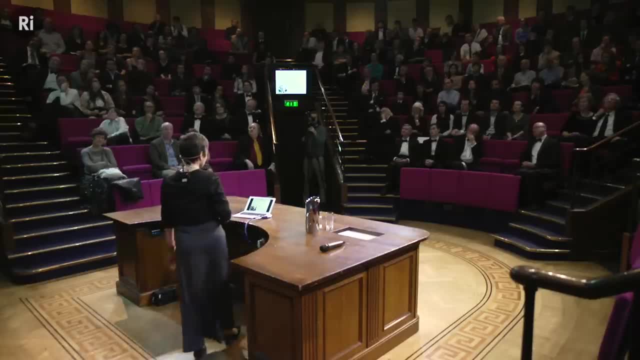 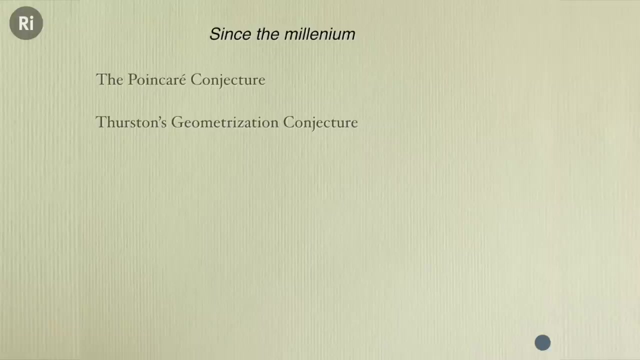 tell us what to do. so what has happened since the year 2000? well, these two conjectures, which I haven't yet told you what the Poincaré conjecture is. but the Poincaré conjecture is geometrization conjecture, which is much bigger and includes the Poincaré conjecture. 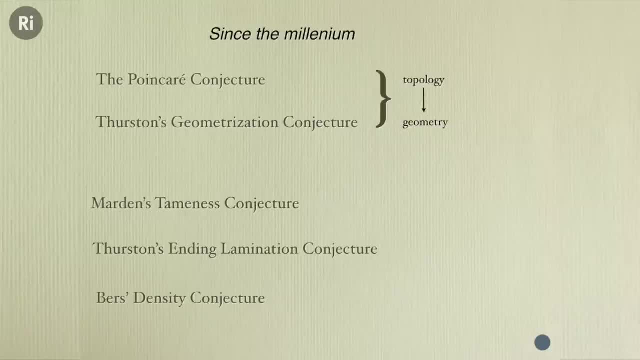 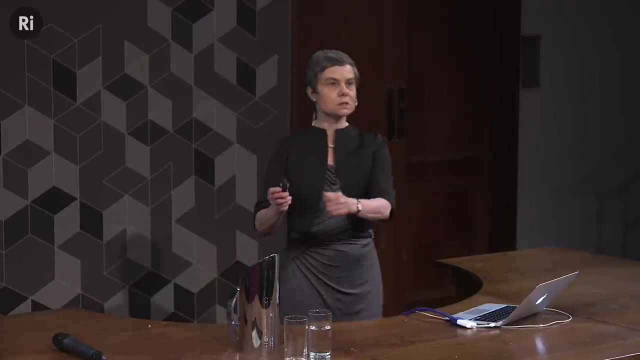 then there are three things whose names won't mean anything, but three other very important things which Thurston and some of his school put together: that between them. if you understood this, you would have understood this mysterious, exotic case, and people really didn't know how to do this stuff. 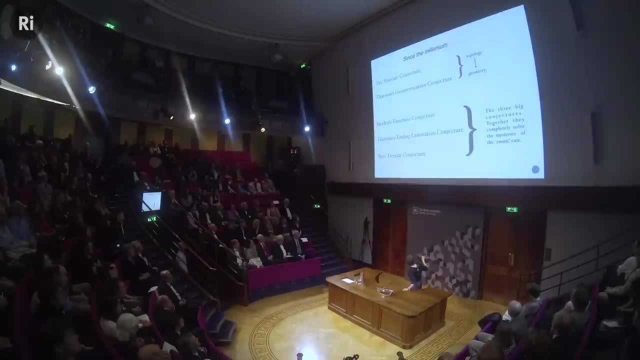 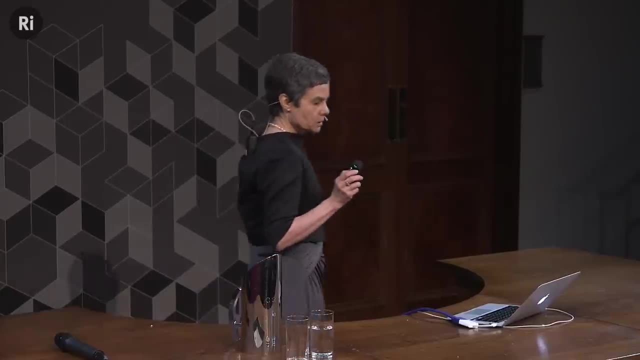 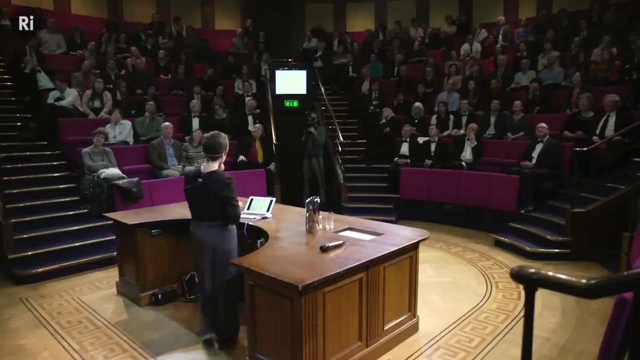 maybe they had a little bit of idea about how to do this, as I'll show you, but really, beyond that, there was a lot of unknown stuff. and what have we done? just to show you, mathematicians have been quite busy, so famously, with an enormous amount of. 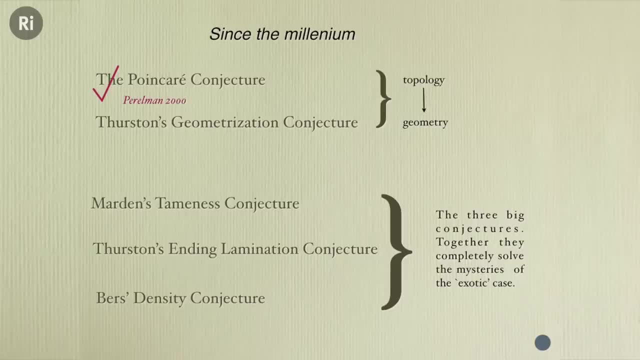 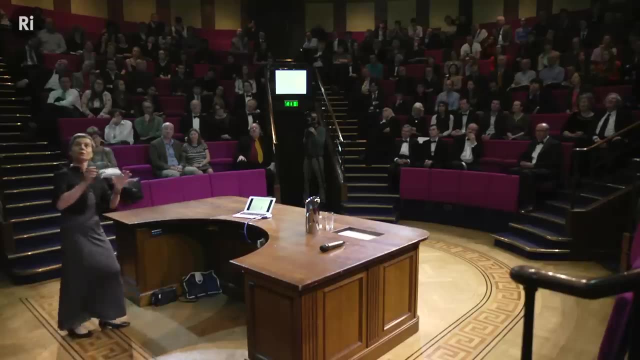 press coverage: Grigory Perelman proved the Poincaré conjecture. I mean it depends when you think a theorem was proved. from the time the person first announces a proof to the time when it gets checked and possibly published can be really quite long in mathematics. 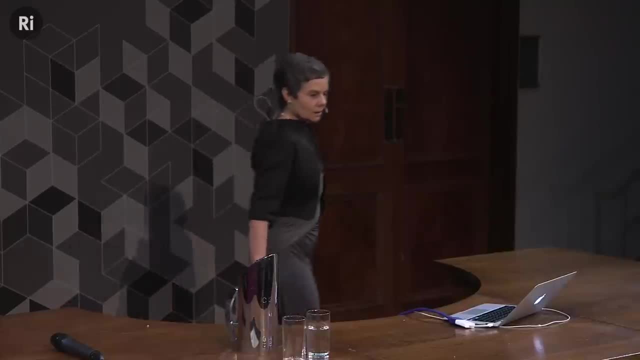 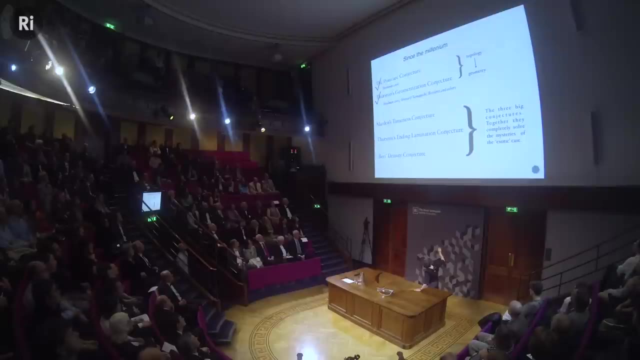 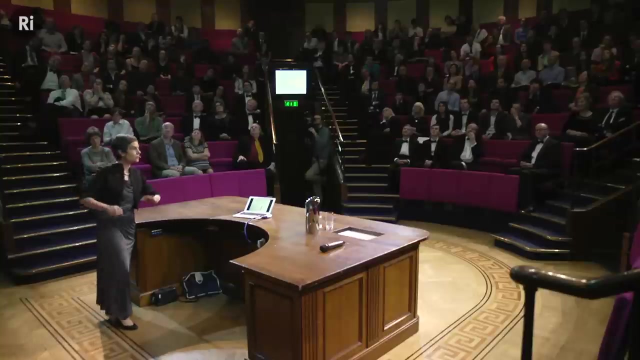 so dates are a little bit so Perelman proved this Poincaré conjecture, whatever that says. and then, based on these methods, this Perelman went further and he explained how to use his ideas, which were completely coming from a completely different direction, to prove geometrization. 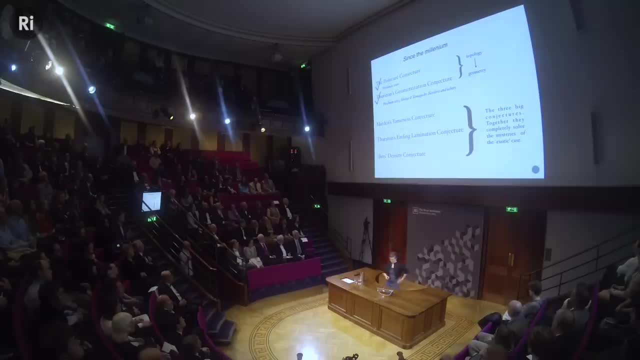 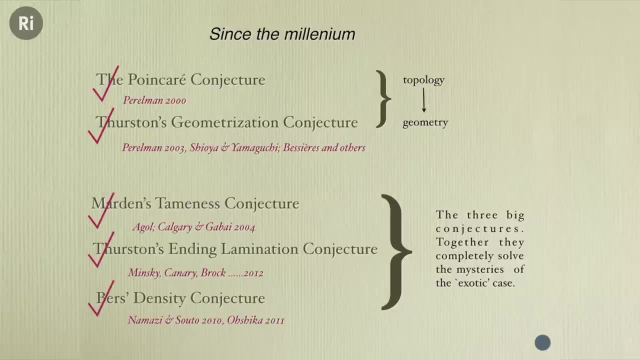 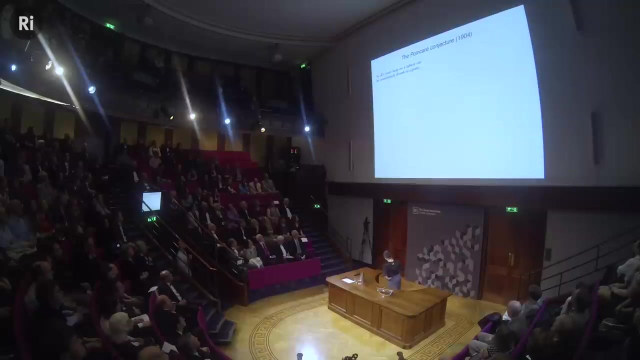 he left some gaps that have been filled in. then these three things, all of these were large pieces of work, so we've kind of done it all. you know everything right. so let me tell you in a little bit more detail what's the Poincaré conjecture. 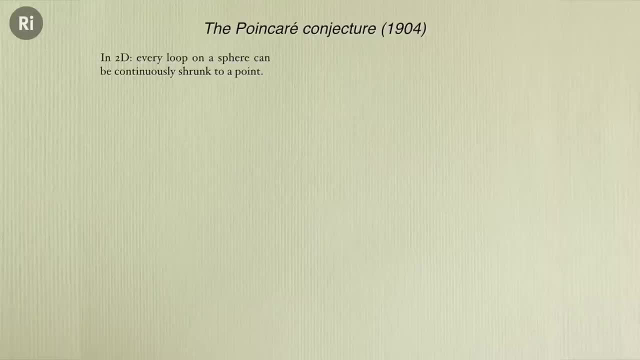 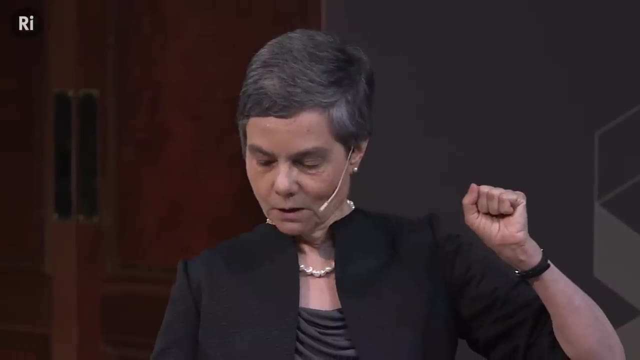 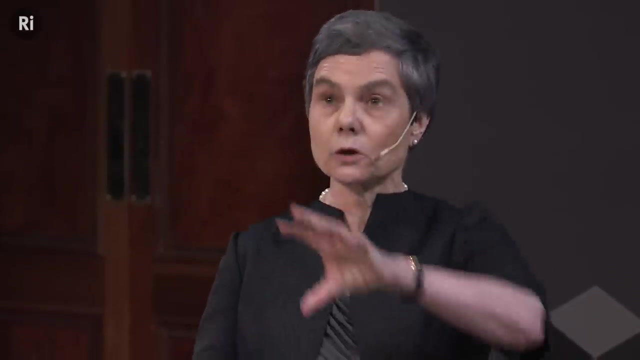 the Poincaré conjecture in 2D: if I draw a loop on a sphere, I can shrink it down to a point. so I could ask the opposite question if I had a surface such that any time I drew a loop on it I could shrink it down to a point. on the 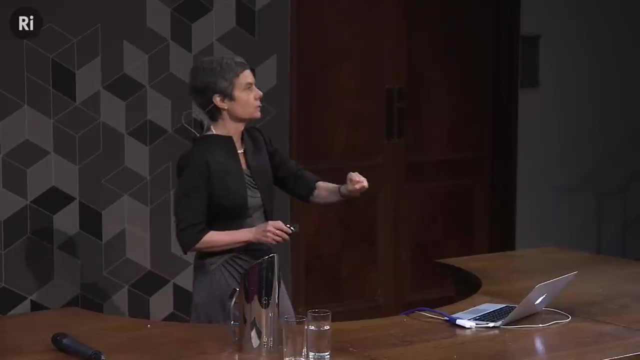 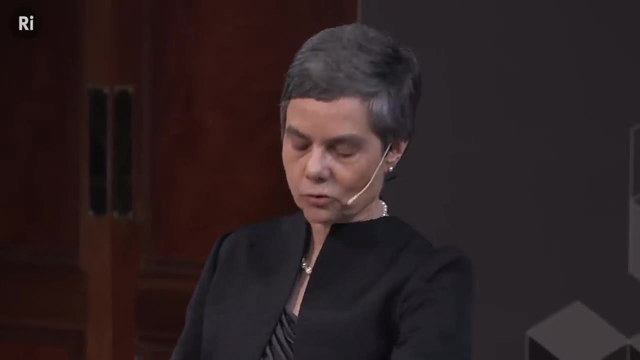 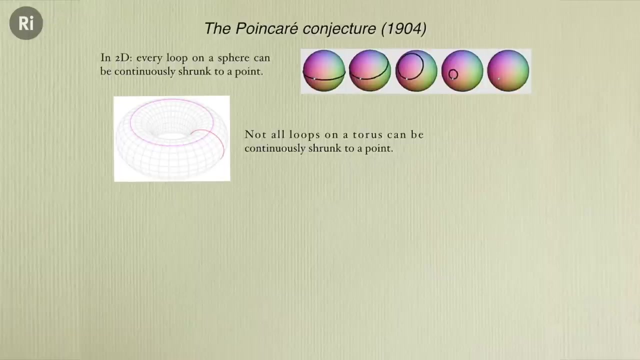 surface, would it be a sphere, and that's part of how you classify surfaces. so it's true that if I gave you a surface and every loop that you could draw around the surface, so here's a torus, I can draw a loop. say this orange thing round here and no matter. 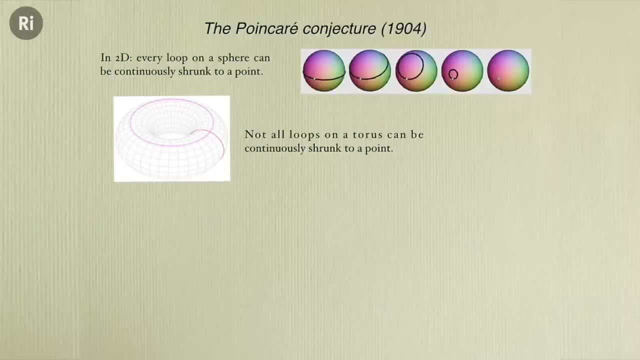 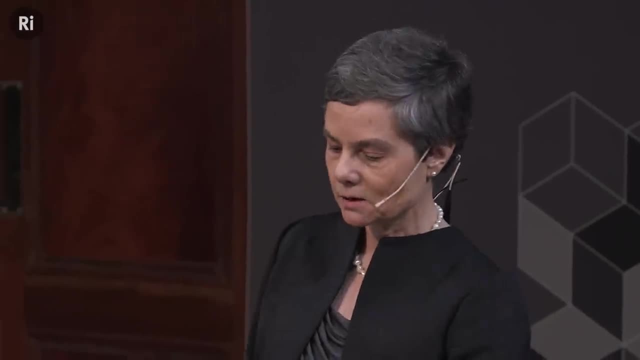 how I move it around and stretch and twist. I will never get rid of it. I can't shrink it down to nothing, so I can detect if I was a fly. I could detect whether I was on a sphere or on the torus by looking at these loops, and could I shrink them down or not? 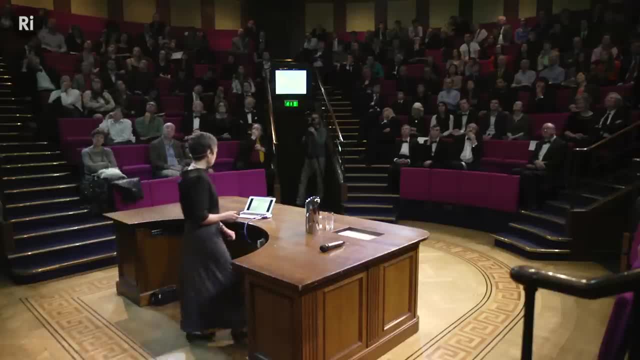 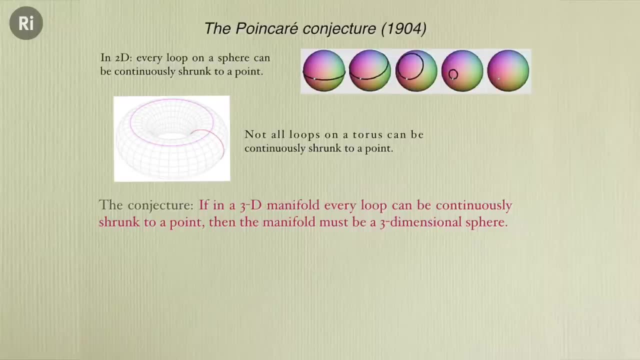 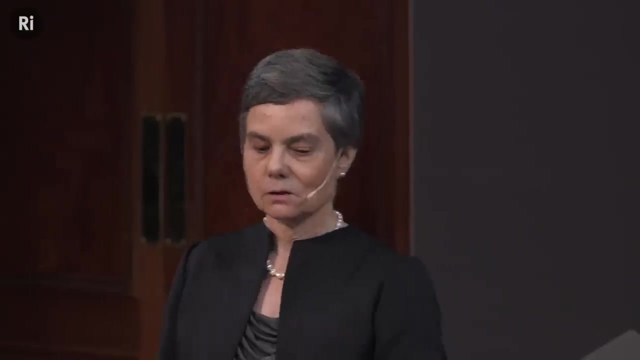 so an innocuous sounding thing. supposing I went up to 3D, I had a three dimensional thing. if I was in a three dimensional sphere, I could do the same thing. I could shrink everything to a point. what happens the other way round? if I could shrink everything, would it be a sphere? 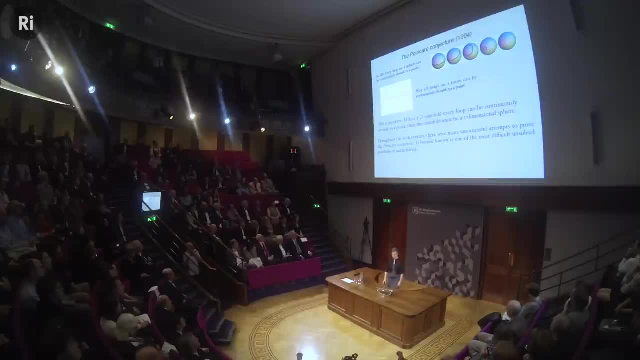 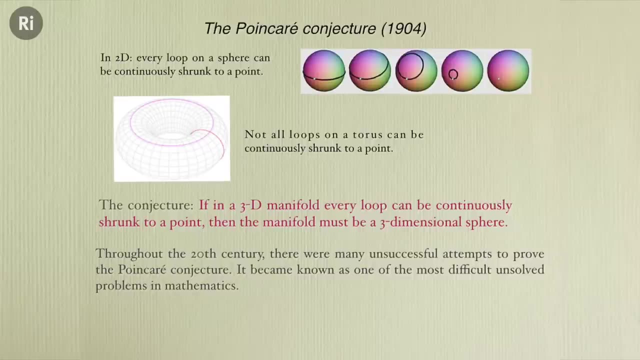 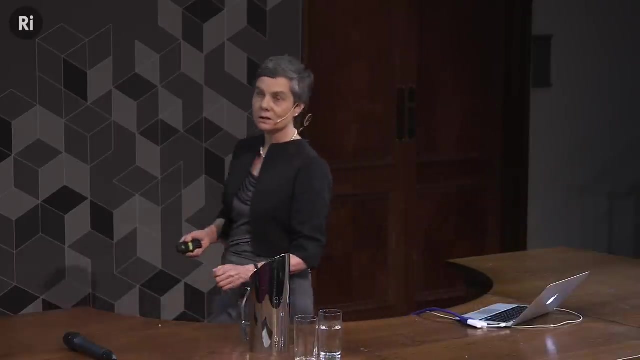 well, you might think that wouldn't be so hard, but actually it's incredibly hard, really incredibly hard. all sorts of people tried and there were many sort of incorrect proofs that were announced, and then people worked hard and found a mistake in them, and this went on and on. 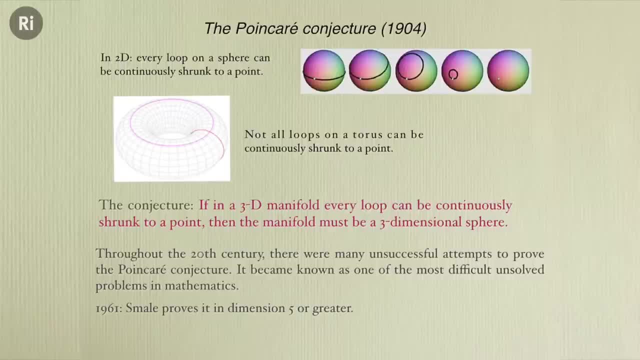 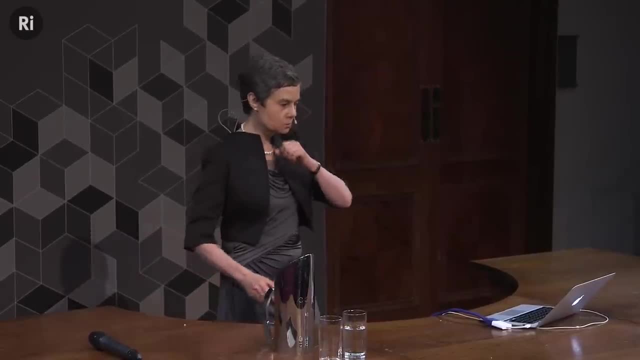 another slightly strange thing in mathematics: you might not be able to do something in three dimensions, so let's try and go to higher dimensions. maybe it's easier. and it's kind of easier because there's more space, so it's kind of it's harder to think about it, but you don't think about it. 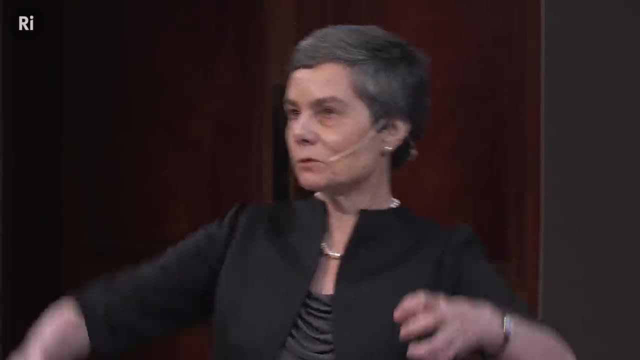 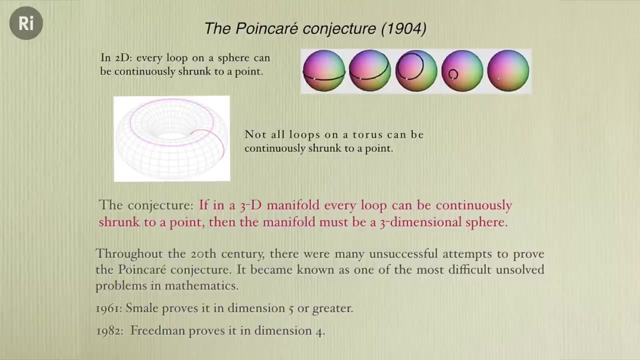 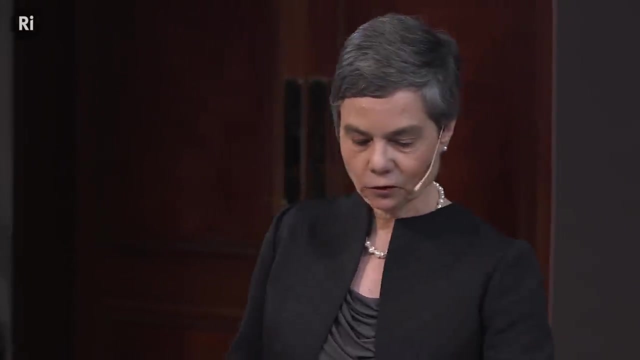 you just move things, so you can kind of move things out of the way and move them around each other, and so it could be proved in dimensions greater than or equal to five. and then it was proved in dimension four and it was still sitting there, unsolved in dimension three. 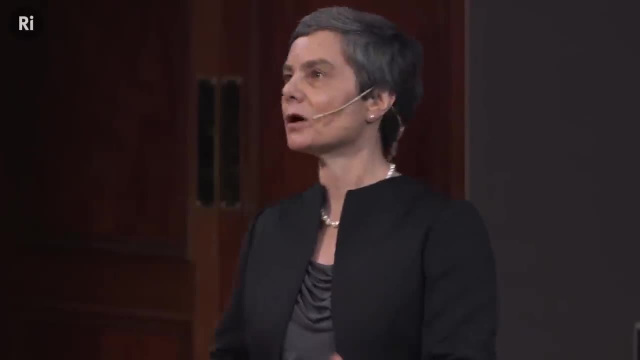 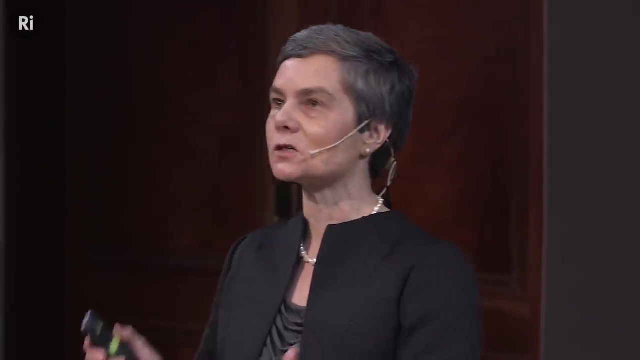 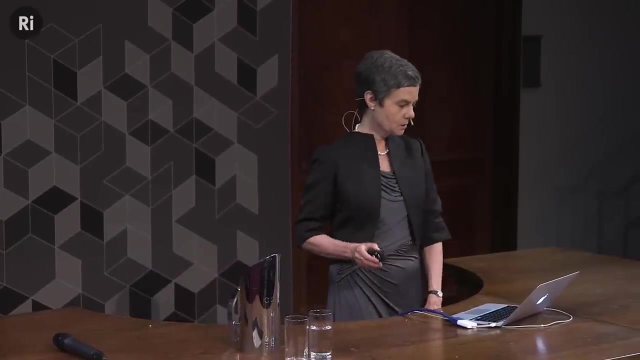 and some big prizes. the clay millennium prizes were set up just before the year 2000 of some outstanding problems of mathematics. there was going to be a million dollar prize for the solution of any of these. the Poincaré conjecture was one of them. 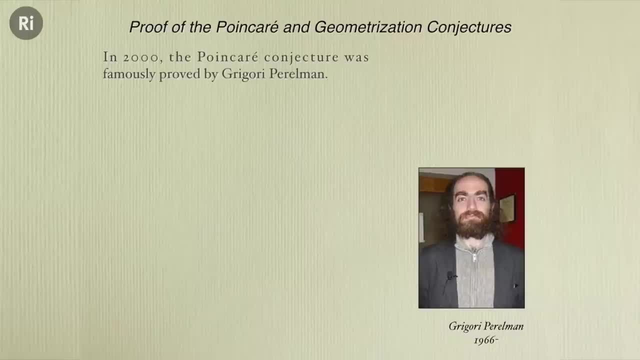 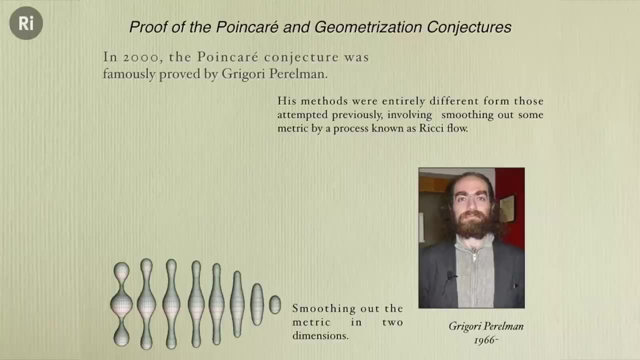 and well, just about the time, Grigory Perlman you see here proved it and he used. I'm not an expert on this at all, but his methods were completely different. he started with not a homogeneous kind of metric at all, but a way of measuring distance. 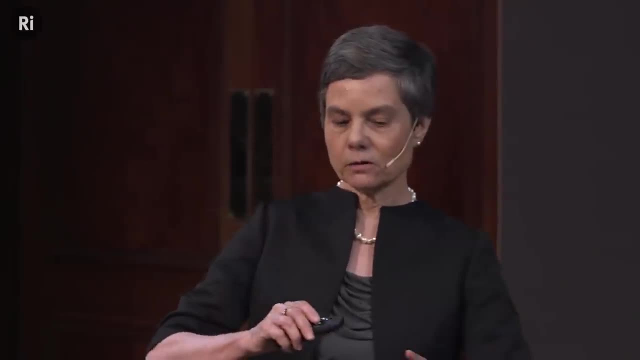 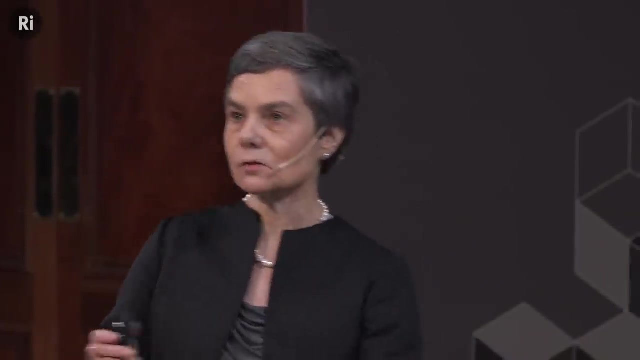 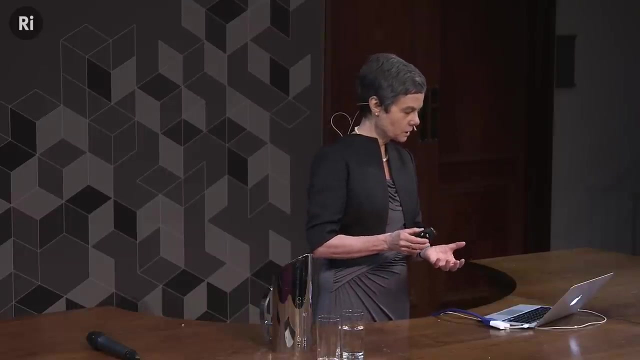 that was just sort of anything and as a clever way of kind of smoothing it out and smoothing it out and you come to sort of singularities and you have to get random cleverly, but eventually you proved that this thing that you didn't know was a sphere has to be a sphere. 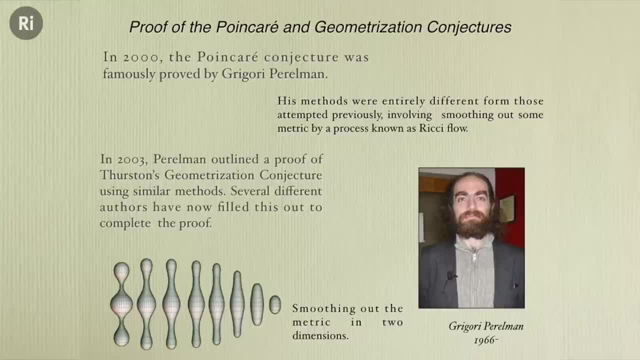 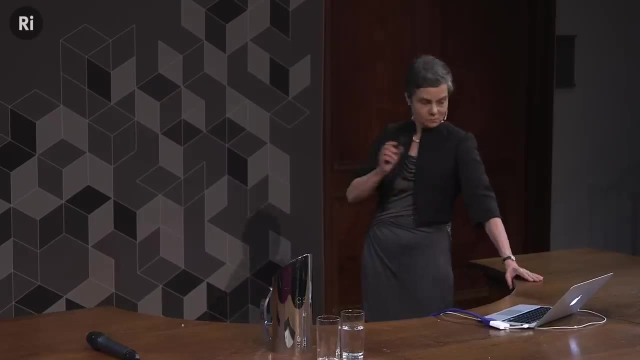 and then he went on and outlined how to prove geometrization and using similar methods. and, as I say, there were some gaps, but they've been filled in okay. and then we have the other three conjectures, which is the direction I've been involved in. so here's a picture. 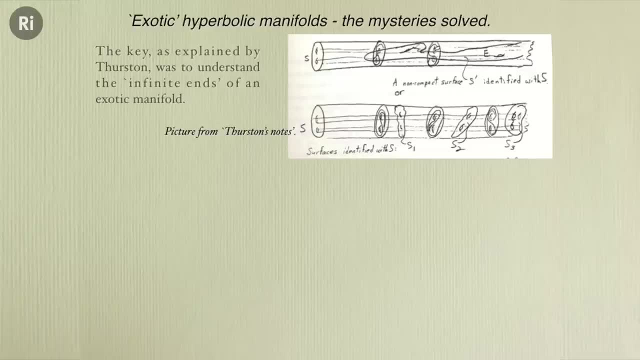 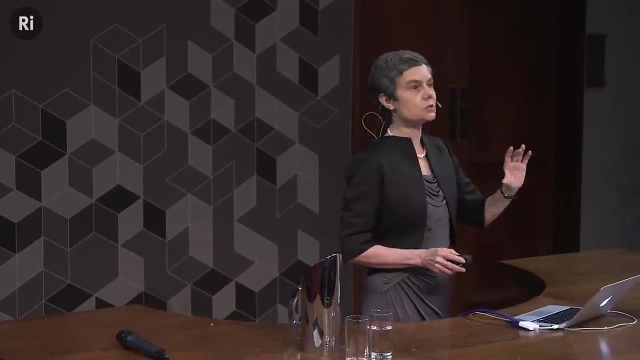 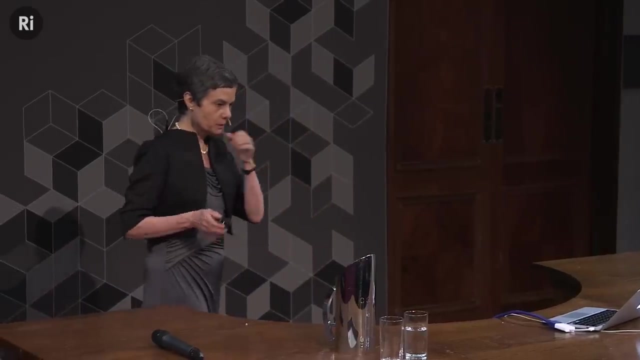 one of the things Thurston did. he didn't have time to write up his stuff nicely, just throwing out ideas every day. but there is a huge volume known as Thurston's notes, which were lectures he gave and were typed up and the sort of beginning part has now been. 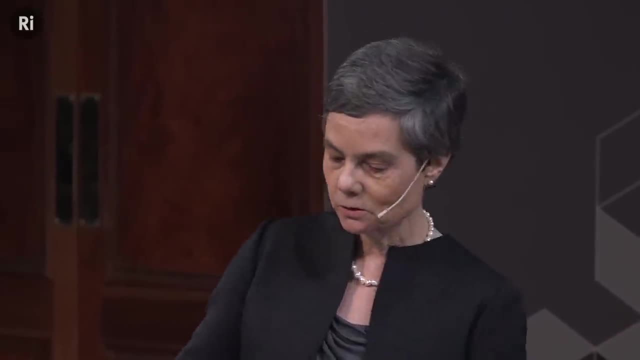 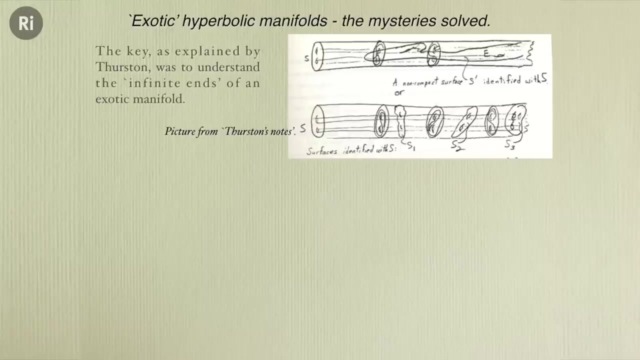 very beautifully edited and filled in and produced as a book. the latter part is still sitting there. you can find it online, of course. here's a picture about. so we've got this manifold with infinite volume and the thing is what he said: it looks like you really don't know what happens, as it goes off to infinity. 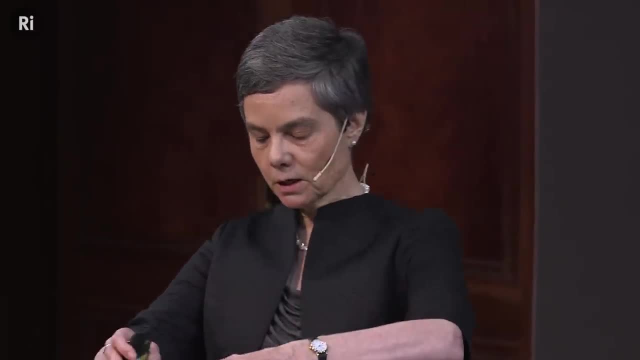 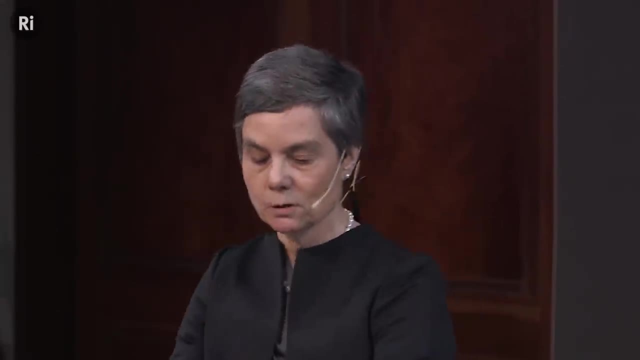 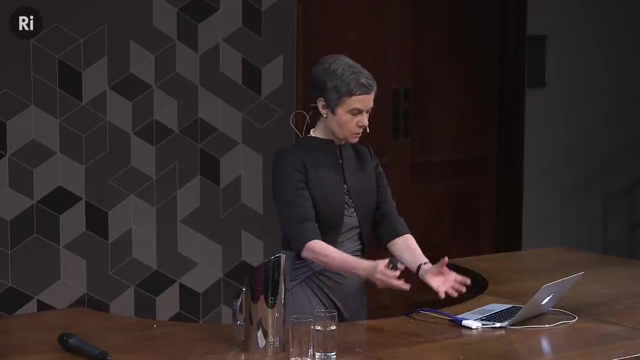 but what he said it might look like is this: you might have a surface and then just take copies of the surface all the way going up and create a three dimensional object. so just like you can take a circle and then a line and make a cylinder, you can take a surface of some kind. 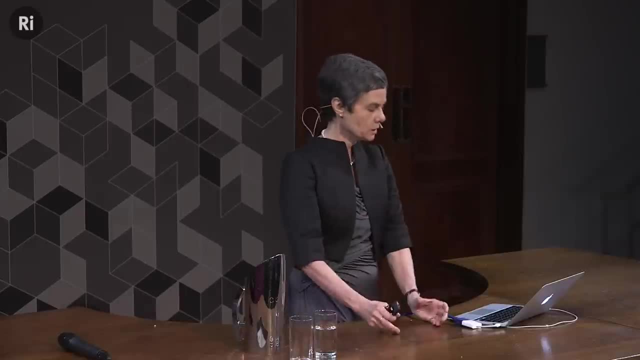 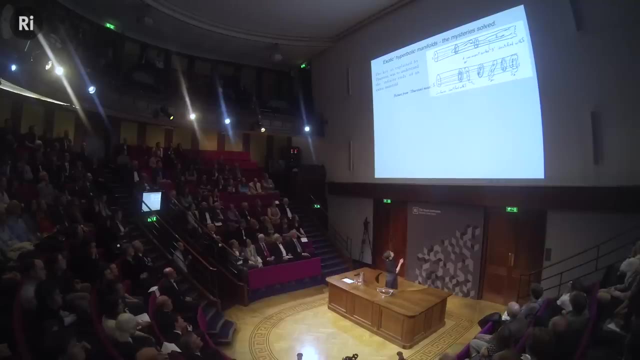 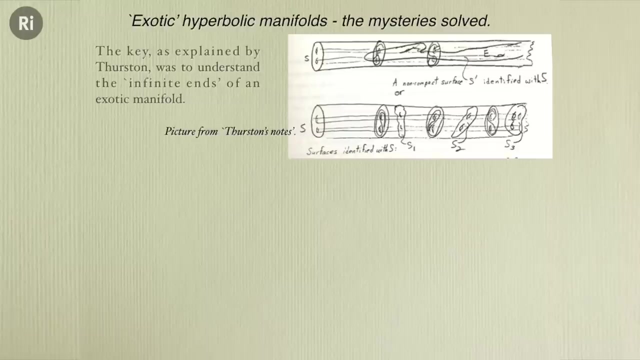 genus two in this picture and go up and you make a 3D thing. and the key point really was that as you go out along here, in these weird examples, these exotic examples, there would be geodesic loops that wouldn't be getting very long all the way out along this. 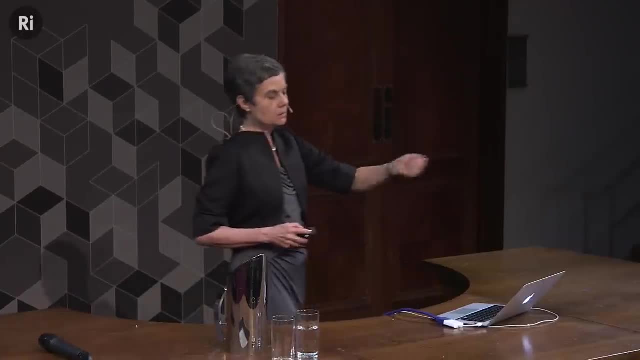 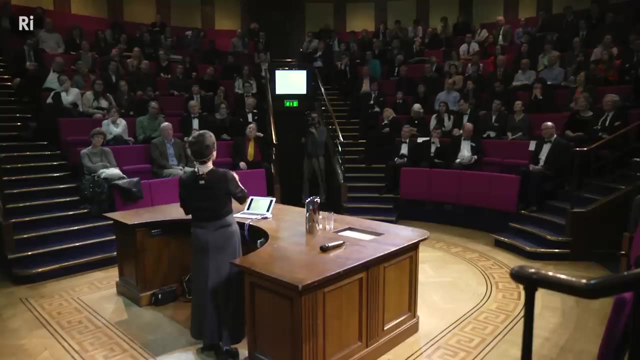 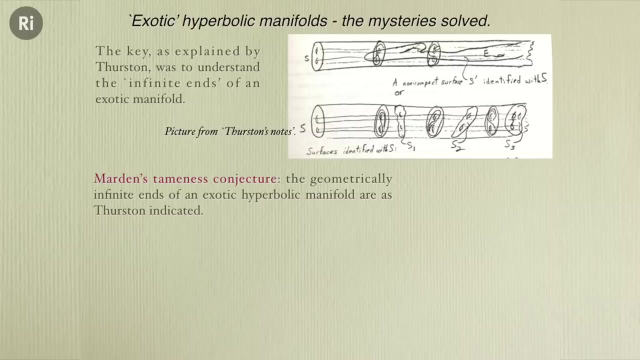 thing forever and ever. so, on the face of it, this end of this manifold, this infinite volume bit we couldn't understand, might have done anything. it might have been twisted in all kinds of terrible wild ways, but actually he sort of tamed it. and this tameness conjecture. 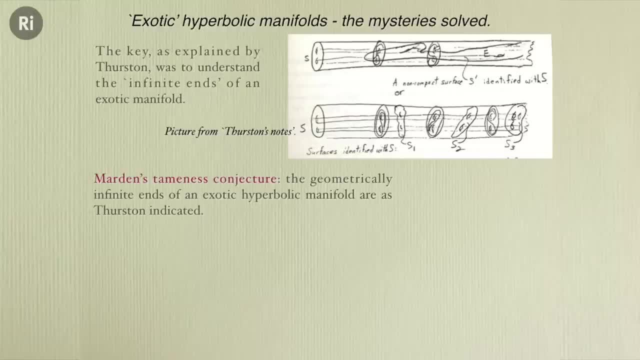 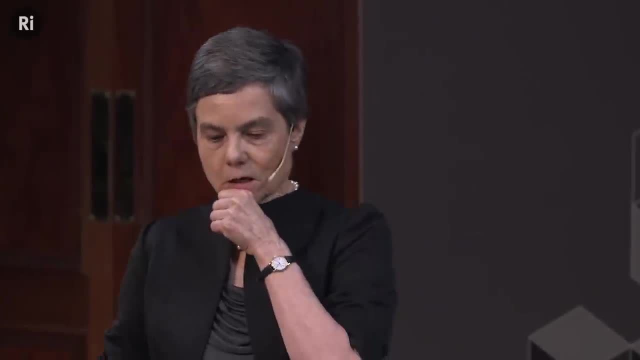 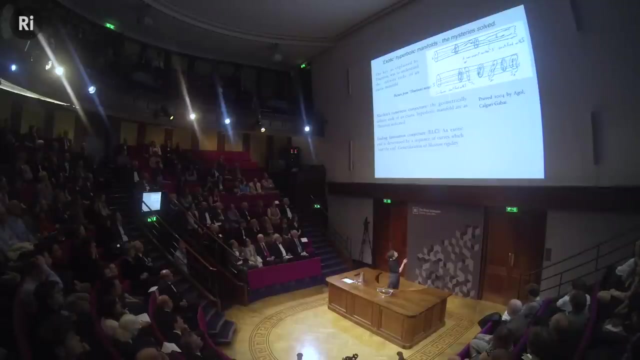 says that, well, maybe it always looks like this. so Thurston showed in certain cases it looks like this, and then Thurston also showed that. well, how would you recognise which type it was? it turns out these curves that go sort of lie on these surfaces, these geodesic loops that go out and out and out. 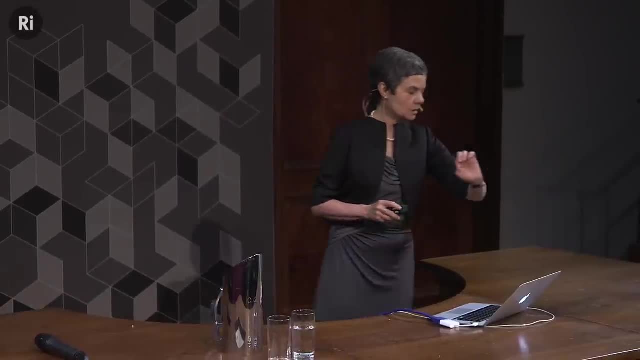 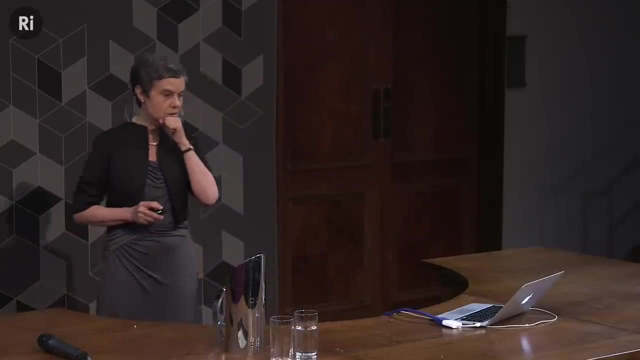 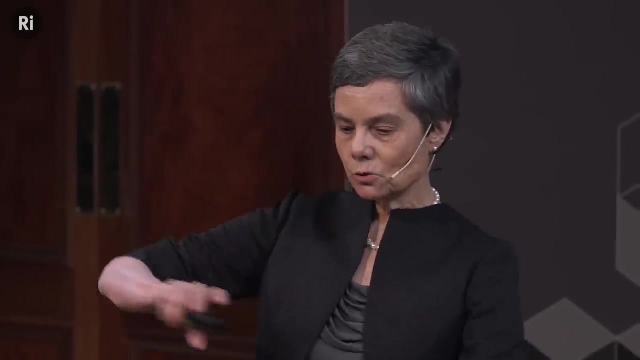 you can sort of think of them like rational numbers, and they have a limit which is some kind of irrational number, an object Thurston introduced called a geodesic lamination, and what he conjectured was if you knew what the irrational numbers, as it were, connected to each of these. 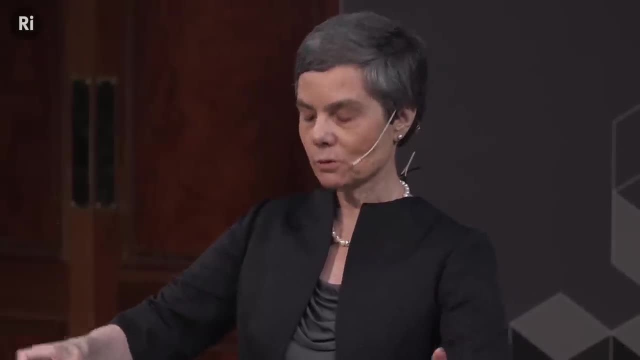 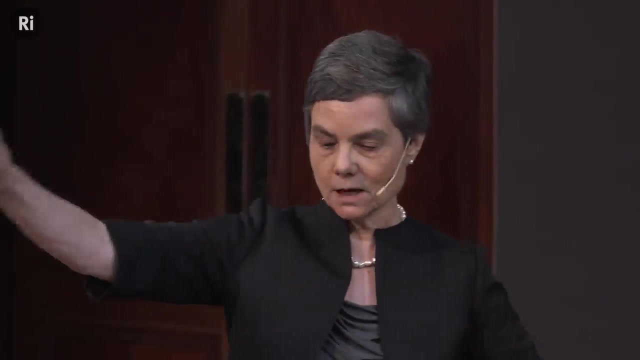 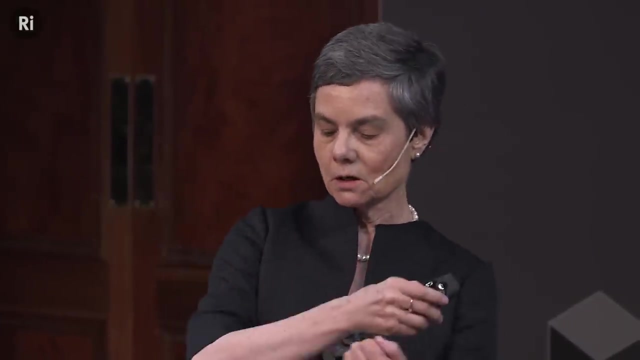 ends were, then you'd know everything. well, that seems pretty remarkable, but actually turns out that's true. and not only is it true. if you know what happens on the ends here, actually you can more or less reconstruct everything that happens in the middle. and this was not Thurston, this was 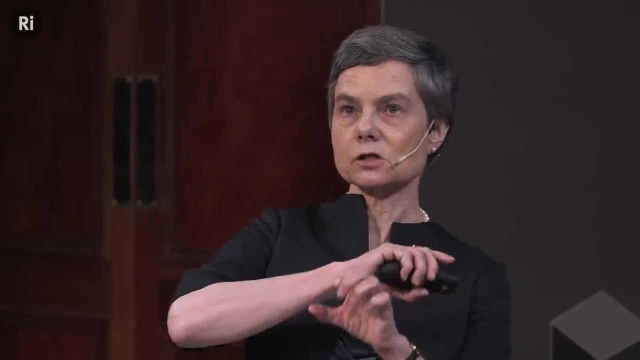 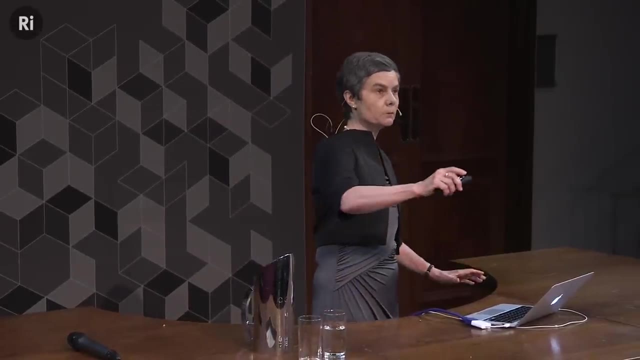 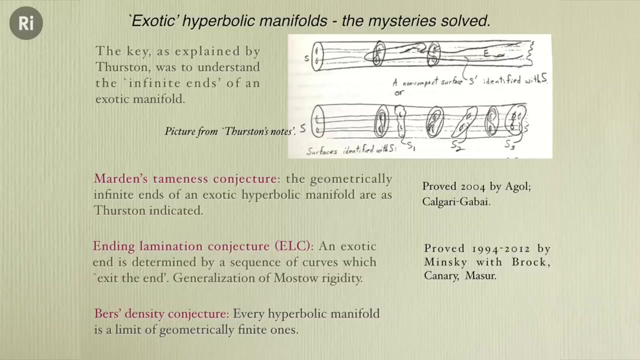 largely Yair Minsky, working with various other people, introducing some really beautiful mathematics and understanding the kind of coarse geometry of the whole hyperbolic manifold just from a very small amount of data about the ends, and then finally, well, could there be any of these things, kind of 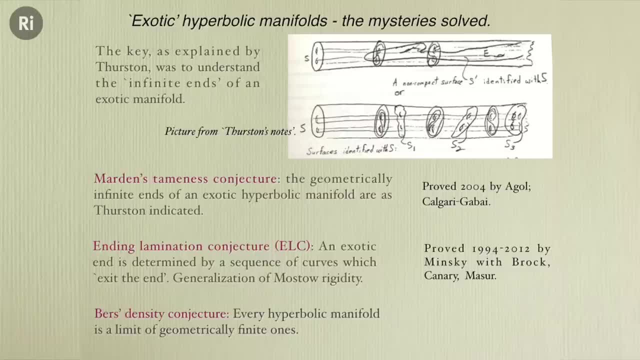 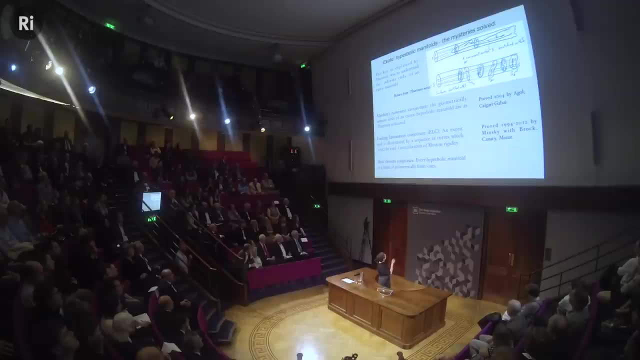 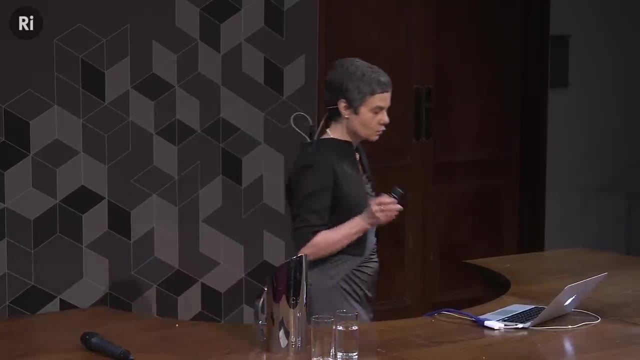 sitting out there we don't know where they are. well, the answer is no, they couldn't. they'd always have to be limits, of ones that we knew about, and it turned out that, once we kind of got this far, this bit was fairly routine, quite routine, but it was more. 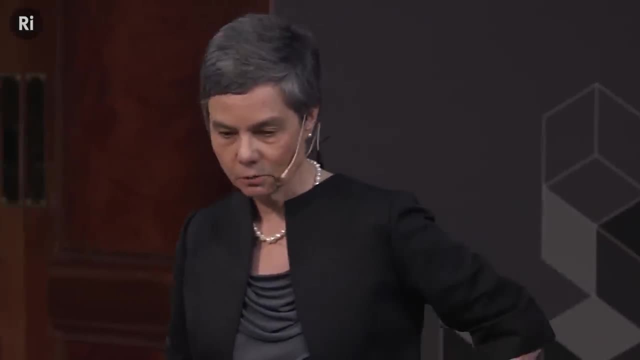 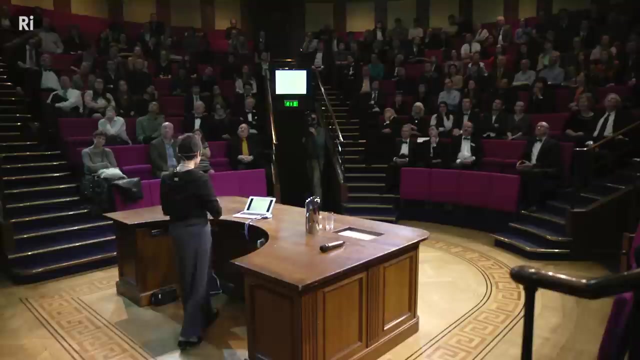 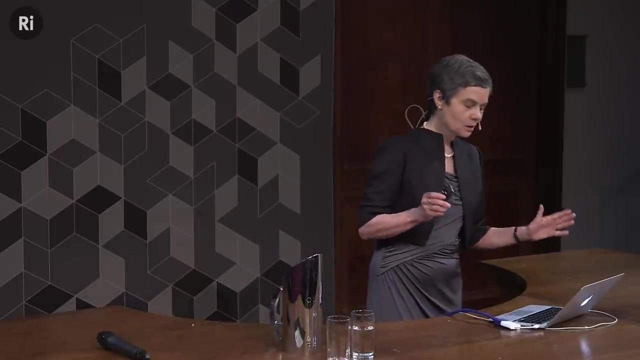 obvious to see how to go about proving that. so that was also proved, right. well, now I don't know if I have time, but let me try to go very quickly through. so you might say: we've solved all the problems, so we. one thing I didn't say was: 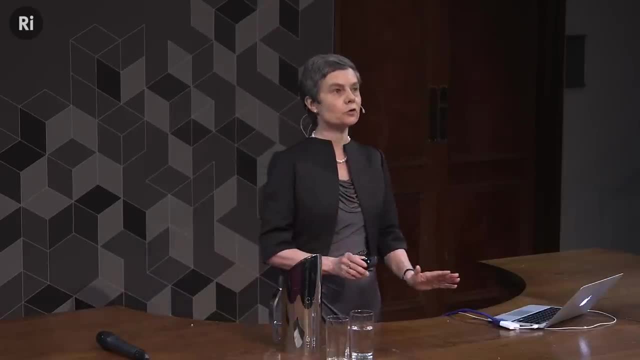 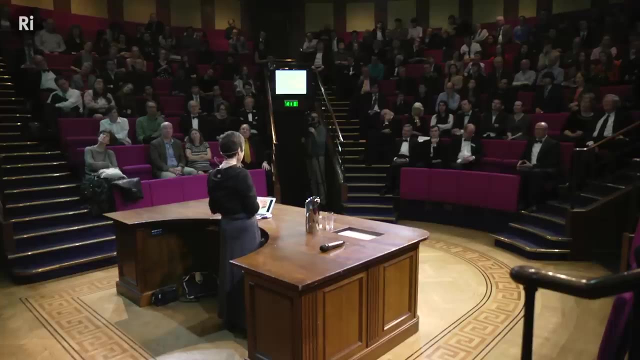 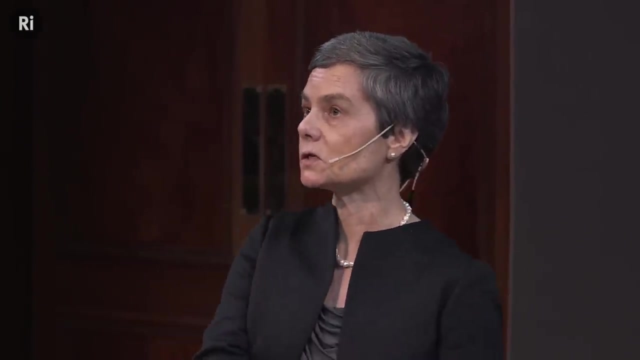 these three dimensional things, you can put geometry on them. we know a great deal now about the geometry examples. it actually turns out that if you in many senses pick a manifold at random, it's going to be hyperbolic, just as most surfaces are hyperbolic, so in 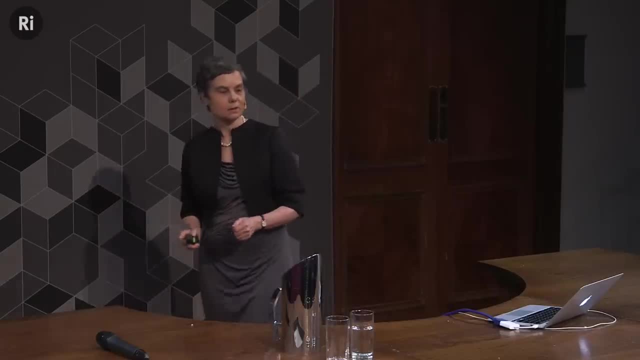 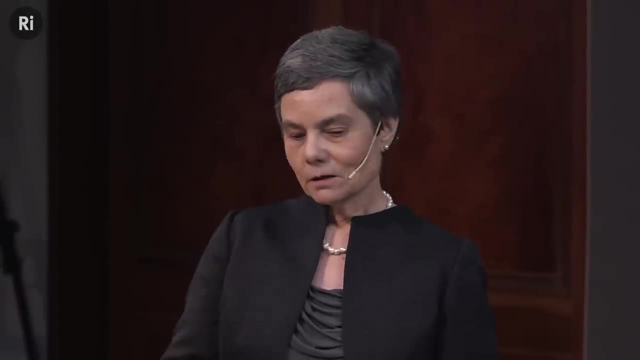 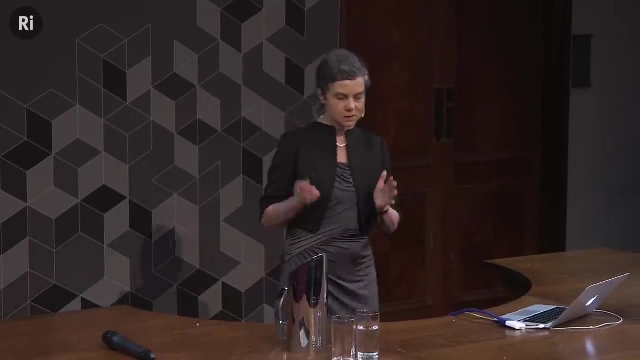 three dimensions. by far the most common thing to happen is for your manifold to be hyperbolic. so hyperbolic has gone from being a kind of slight sideshow to something really fundamental, and I would say we're at a point now where we kind of understand. 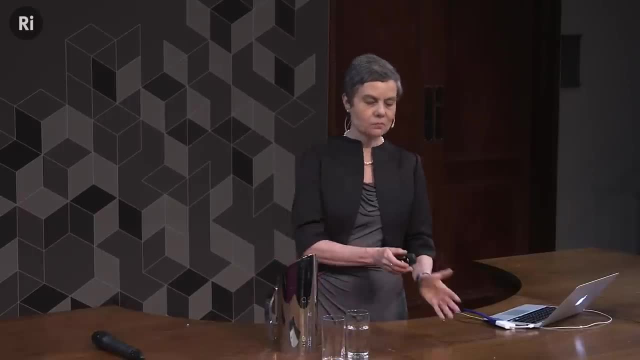 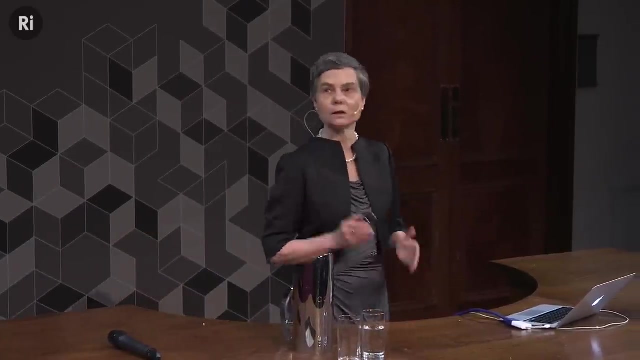 that, but I said that surfaces were used, for example, to develop things to do with chaos theory. people are playing now, but I think the facts we now know about these three dimensional things are surely going to come into play in the future in ways that we haven't as yet. 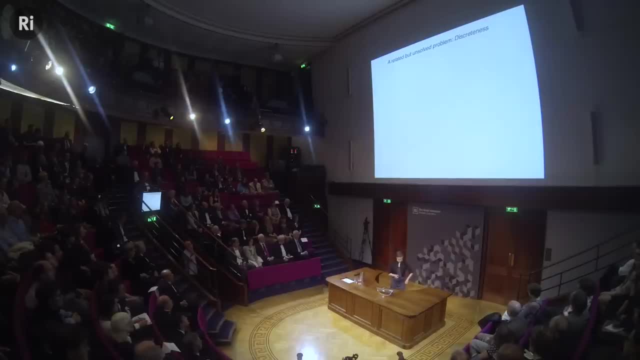 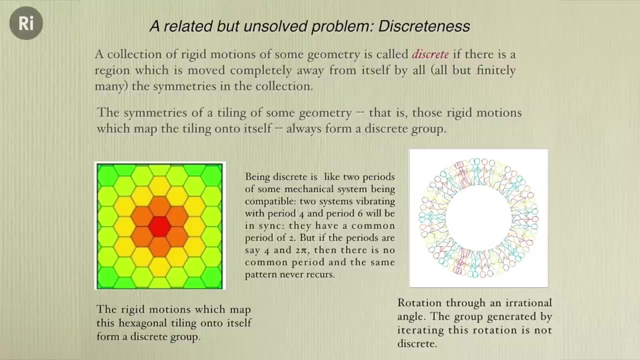 understood. okay, so well, very fast, okay, so discreteness. so discrete means that you can move things away. if you've got rigid motions of some tiling, you can move the tile away from itself and it never comes back and hits itself. on the other hand, if you start, 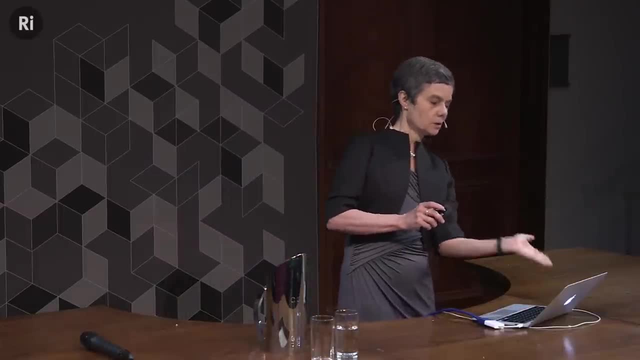 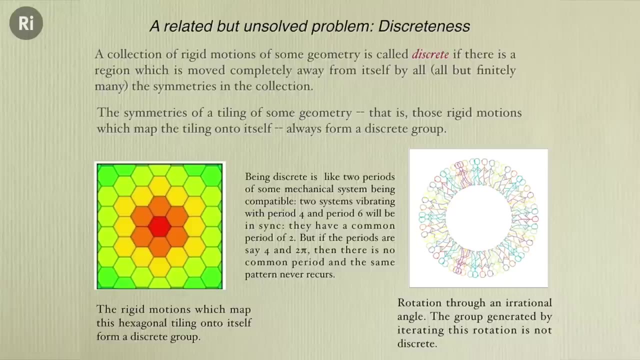 rotating thing and you go around an irrational angle, an angle that's not commensurable with two pi, then you can go around and you'll come back, but you won't come back exactly on top of yourself and you'll keep going round and round and round and you'll. 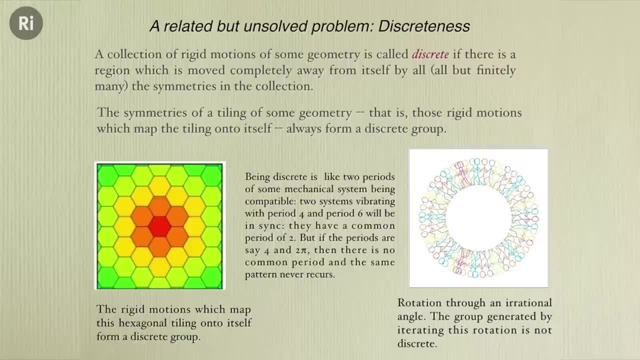 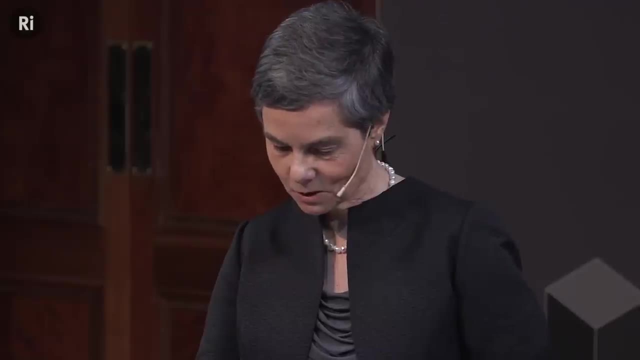 end up producing a picture like this, and the longer you go, the more you'll overlap yourself. so being discrete is kind of nice. let me just skip here and let me just show you my last slide. so I don't have time to tell you that, but let me just leave you with. 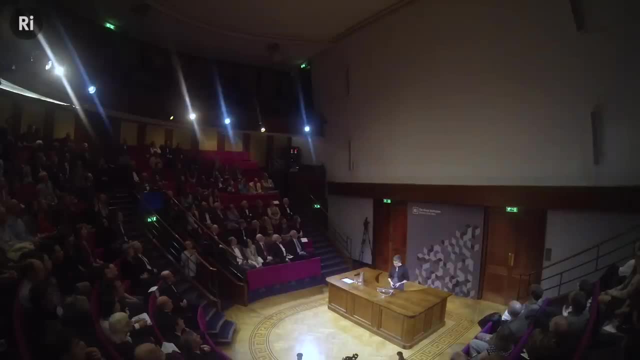 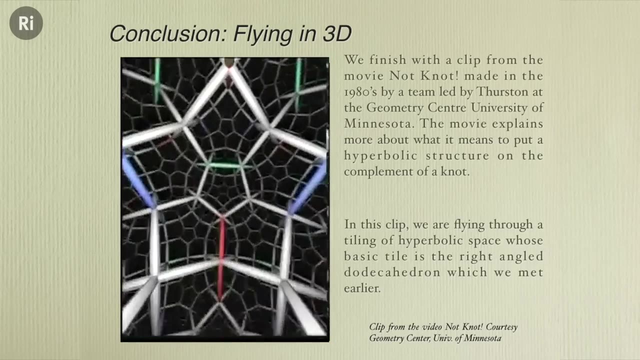 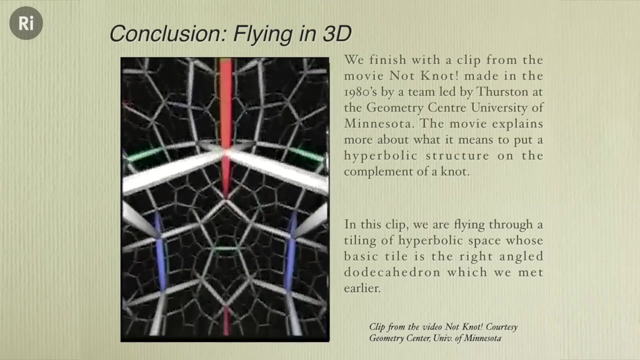 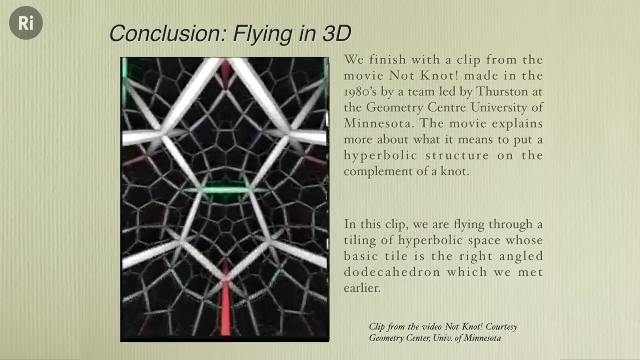 this last picture, so just a picture of what it looks like to fly around in three dimensional hyperbolic space. this picture was made by this geometry centre, which was part of the offshoots of all the flurry of activity around Thurston's work, so I'll leave you there.